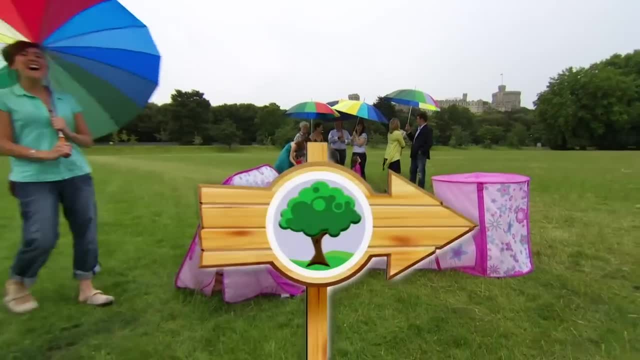 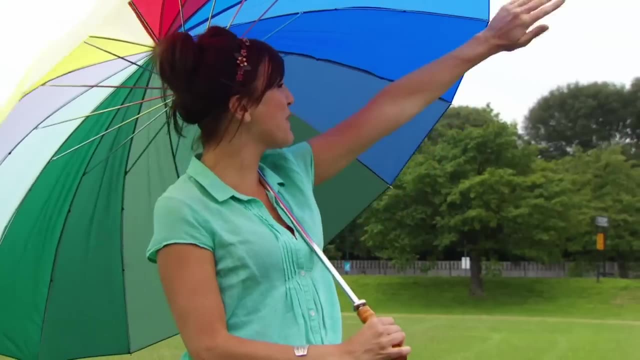 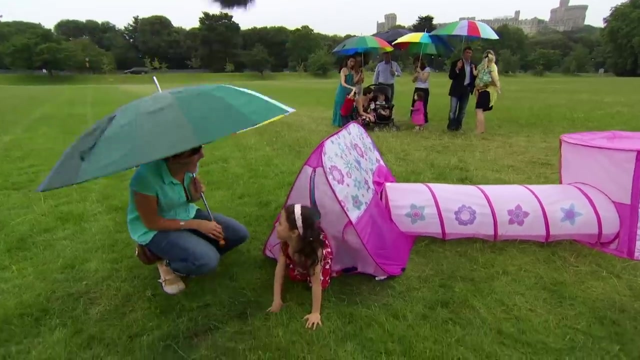 Let's cook a feast for everyone. Here we are, next to the castle and, oh, it's a little bit rainy. Now I can see all of Pula's friends and family. Hello, everyone, Hello, But I wonder where Pula's hiding Katie? There you are, Pula, and who's in your tent with you, Katie? 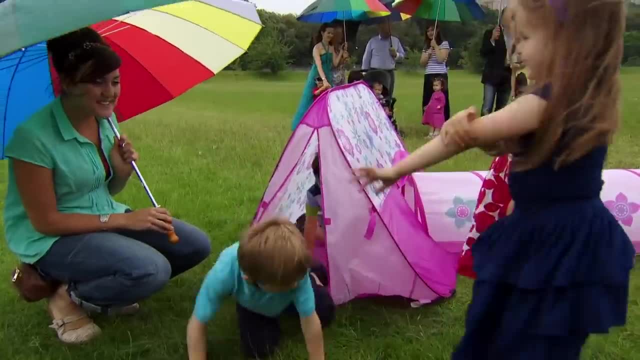 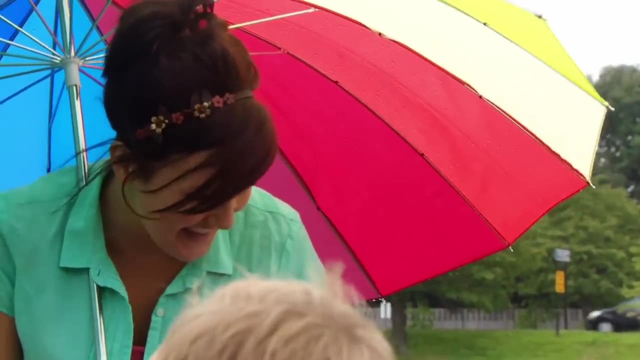 Hello, Katie, lovely to meet you. Freddie Hiya, Freddie, good to meet you too. And what's your name? Khan Khan, great to meet you. Pula. what are we going to do? We're going to do today: Make something for my tea party, Brilliant, and I have got just the thing that. 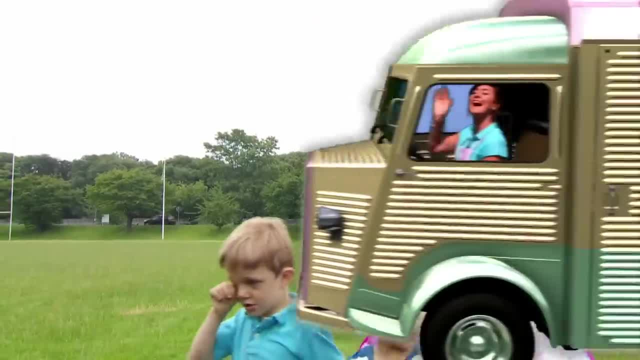 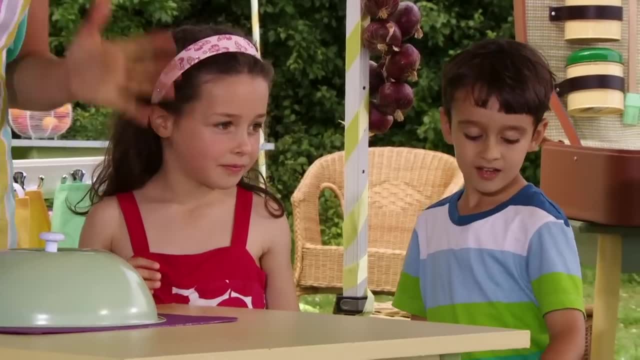 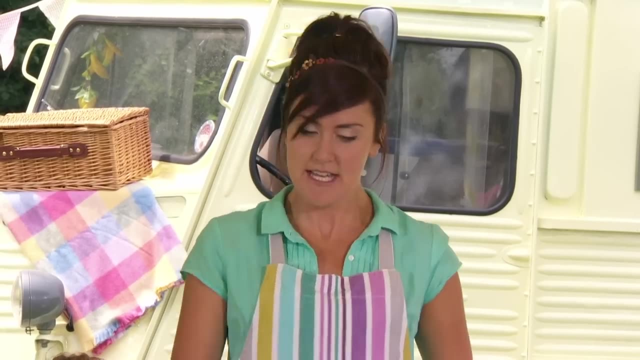 we can cook. Follow me, Welcome to my outdoor kitchen Now. would you like to know what delicious recipe we're going to cook today? Yes, Alright, I'll tell you. Today's recipe is very special. It is the delicious, the scrumptious strawberry crown. 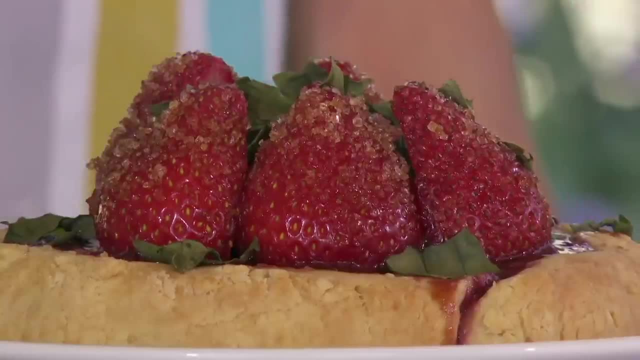 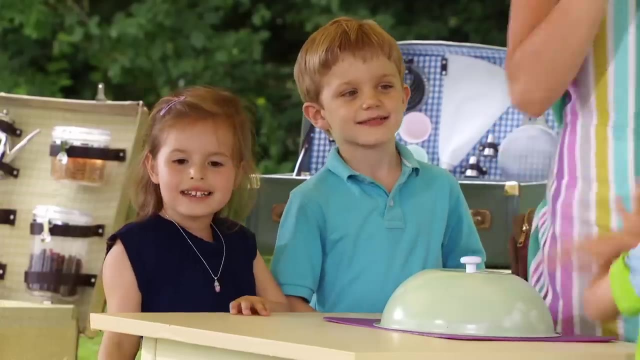 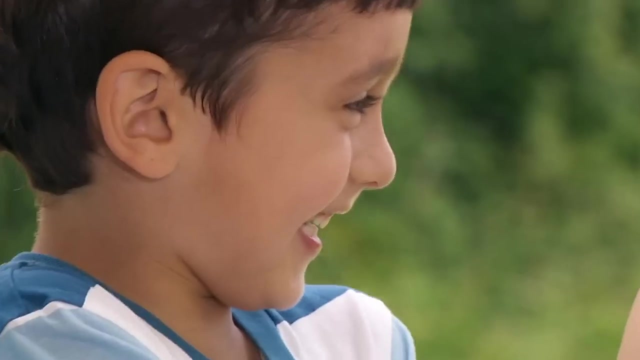 That looks so good. I can't wait to make it. But before we do make it, there's something really important that we need to do first. Do you know what it is? Wash our hands. That's right. we need to wash our hands Off. we go everyone. Roll up your sleeves, Give your 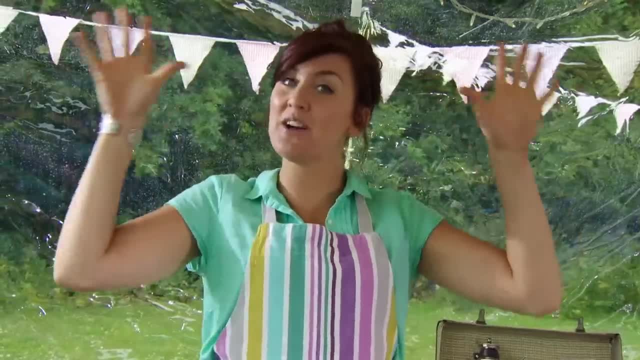 hands a wash with flippy dippy soap: Splish splash splosh. Have you done your hands Washed and dried? Splish splash splosh. Have you done your hands Washed and dried? Splish splosh. Have you done your hands? Washed and dried? Splish, splosh, splosh. Have you done your hands? Have you done your hands? Slipped your hands? Gl implies: we're washing our hands. Slipping wear your hands. We're washing our hands. 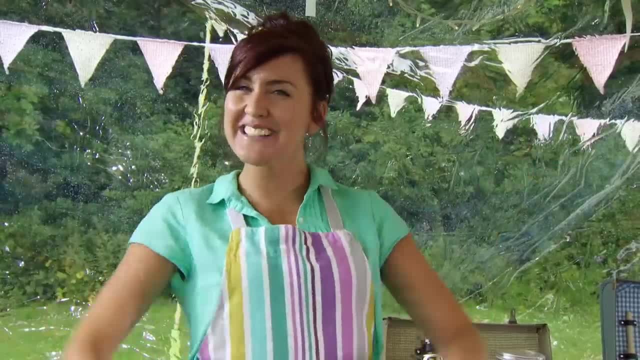 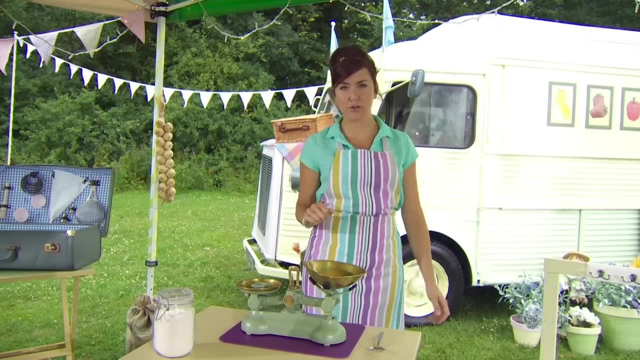 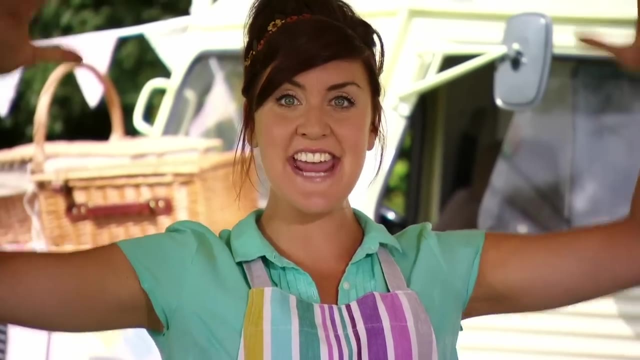 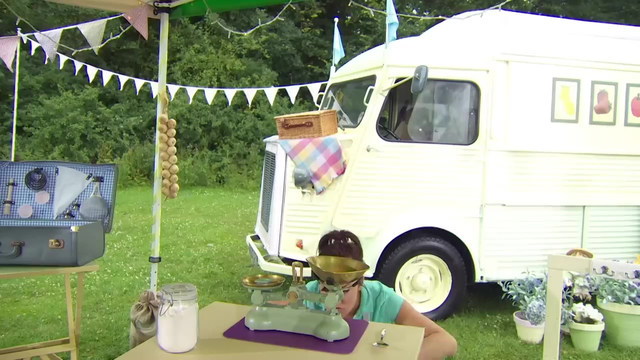 Slipping. wear your hands How we clean our hands. What we're doing right now is washing our hands, using our slimy hands, Knitting their hands with our szczang Shawn on her sweater. Ready Go, And this time. why don't you join in? 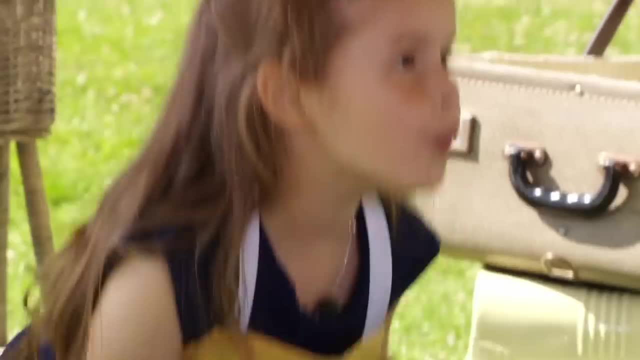 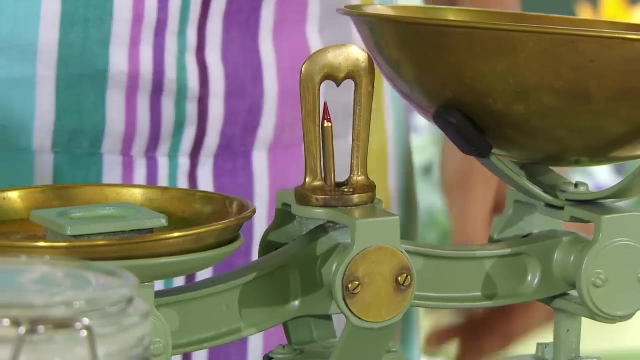 OK, we go down, down, down. Now we're going to play the weighing game with our self-raising flour. So we've got some scales here Now. this weight weighs as much as the flour that we need, which we're going to put on the other side of the scales. 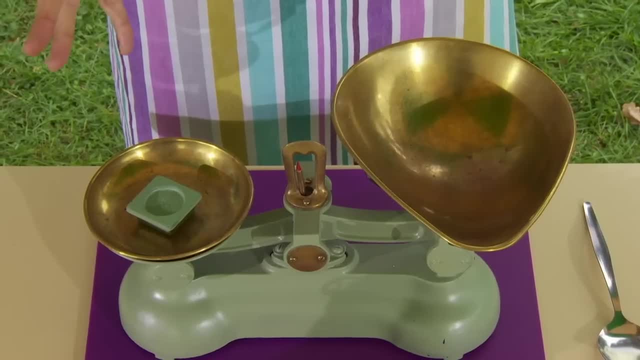 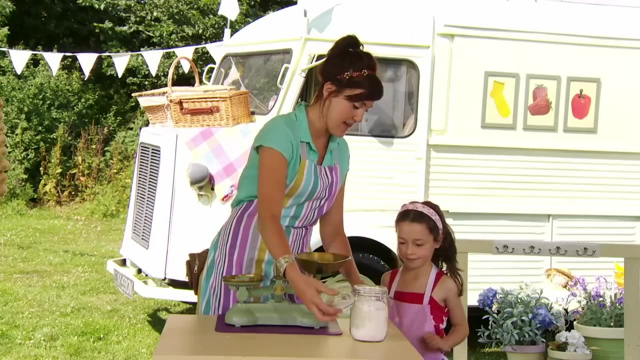 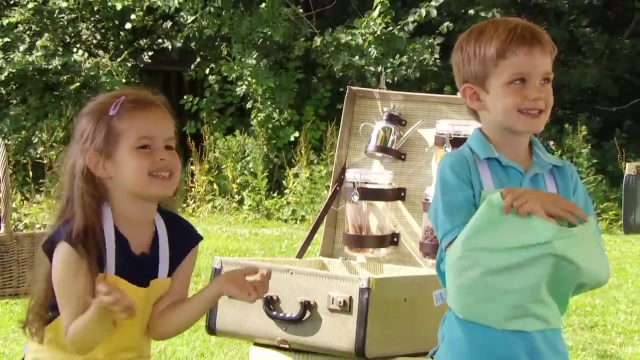 And we keep adding the flour until the two sides are exactly the same. Pula, why don't you come and help me? OK, here's the jar of self-raising flour And there's your spoon, And we are all going to shout out if we need more or less. 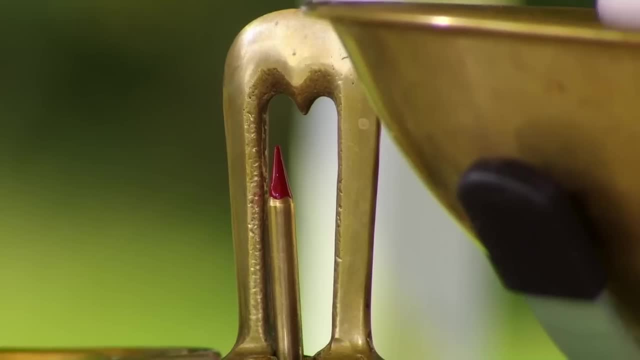 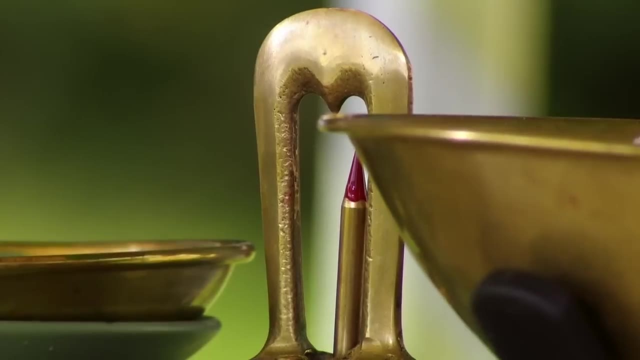 OK, let's play the weighing game. OK, Pula, More, More. You're doing a great job, Oh, Less, So you need to take some out now. Less, OK, quick, quick, quick. Less, less, less. 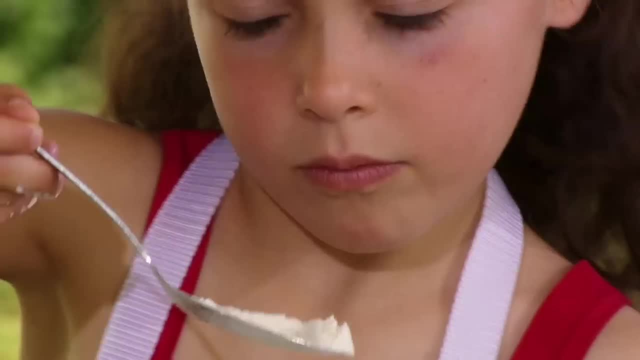 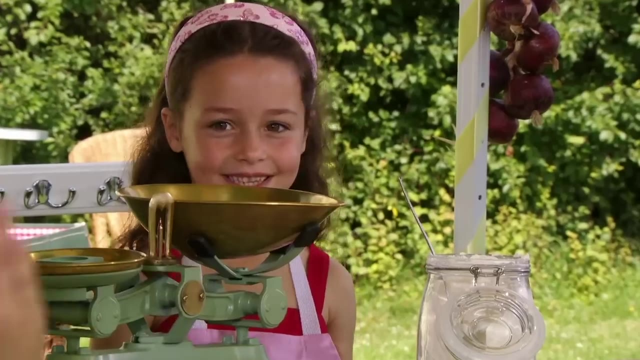 Oh, wait, wait, wait. A little bit more, a teeny bit more. Have they balanced out everyone? Yes, Let's give Pula a big clap. Woo-hoo, Now we've added some butter to our self-raising flour. 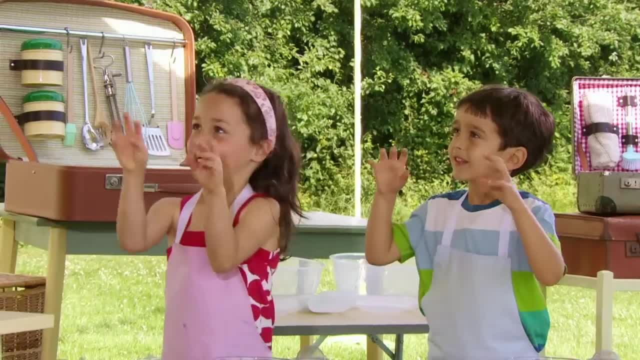 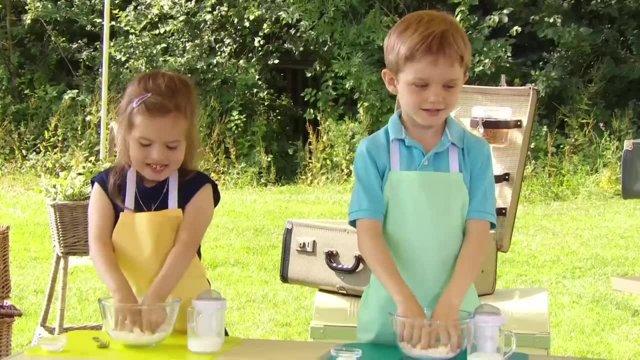 and we're going to give it a good tickle. Everyone go tickle, tickle, tickle, tickle, tickle. So have you got your tickle fingers ready? Fantastic, Let's get tickling Pula. what does it feel like? 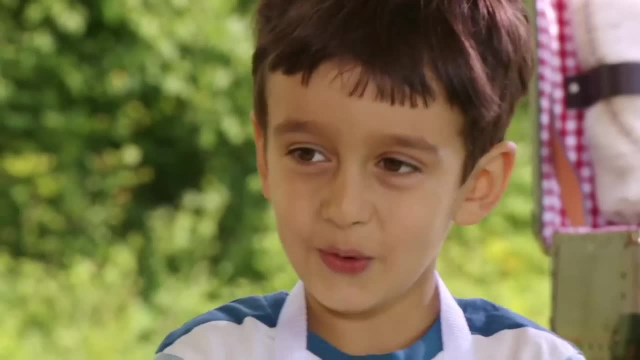 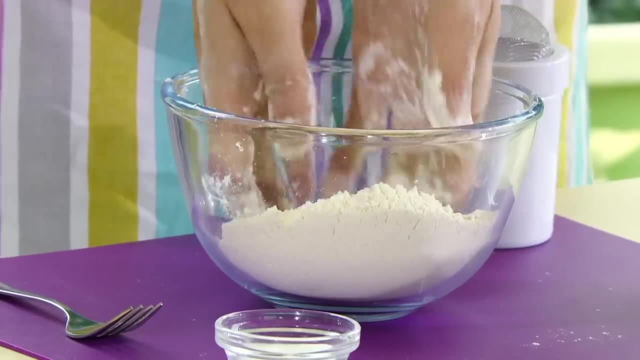 Soft and squishy. Squidgey, Squidgey, Squidgey. Oh, my butter's all disappeared. It's all crumbly in little pieces. The next ingredient is caster sugar. OK, so pour that in Whoosh. 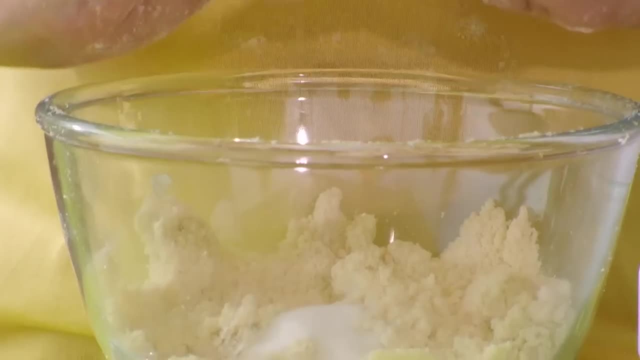 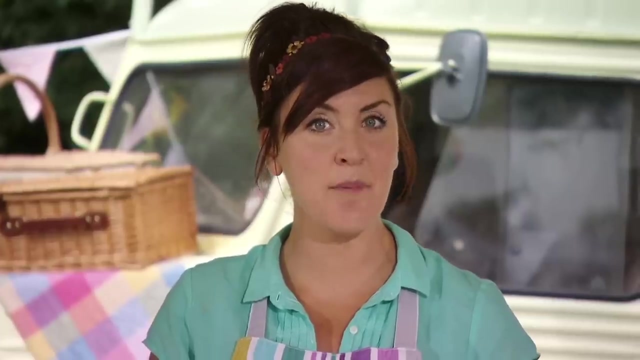 Oh look how sparkly it is. It's like glitter. And the next ingredient is milk. Now, where do you think milk like this comes from Cows? Can you moo like a cow with us? One, two, Three. 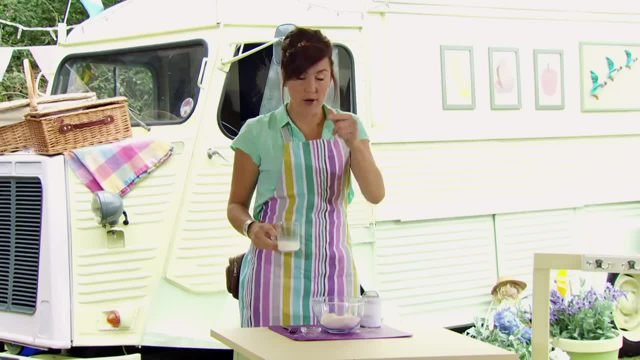 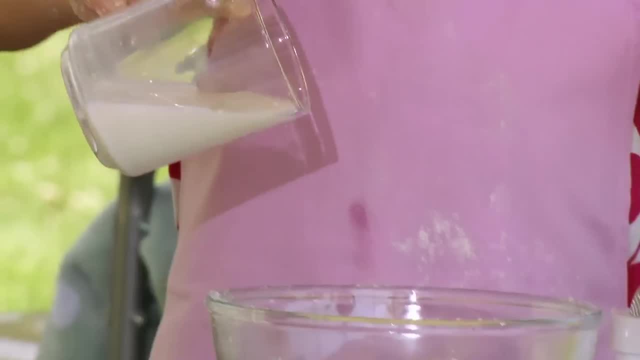 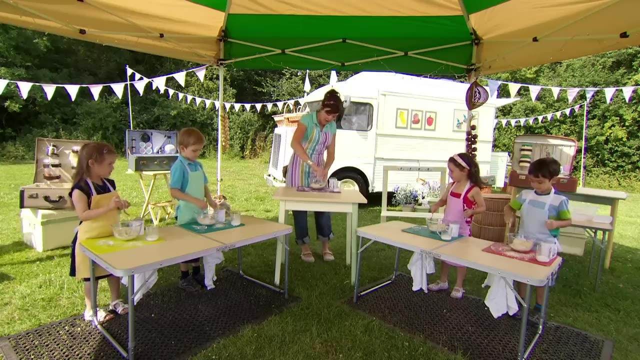 Moo, So you need to get your cup of milk. We're going to add some, but not all. Go and stop, And now we're going to use our fork to give it a Mix. All right, everyone, hold your bowl and give it a good mix. 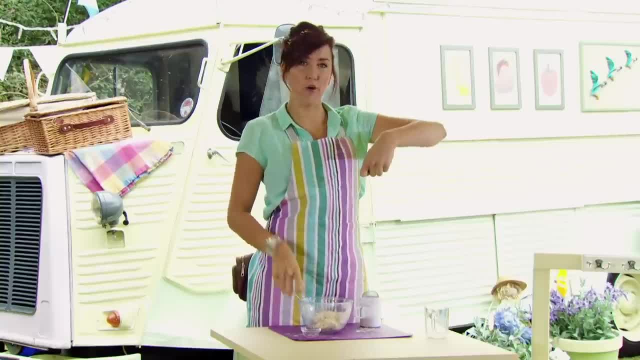 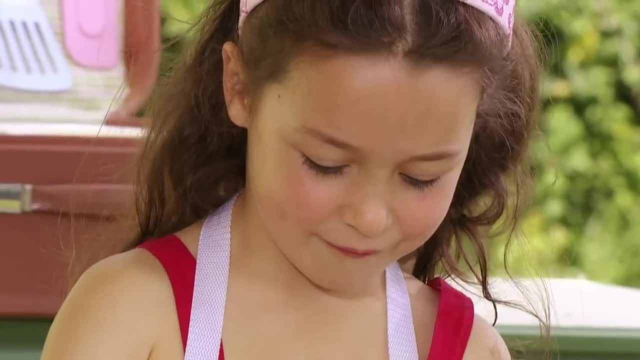 Don't forget that you can mix with us as well. You can get your bowl and your fork and you can Mix, mix, mix, Mix. Mine's all sticking to my fork- Pula. that's fantastic. It's exactly what we're looking for. 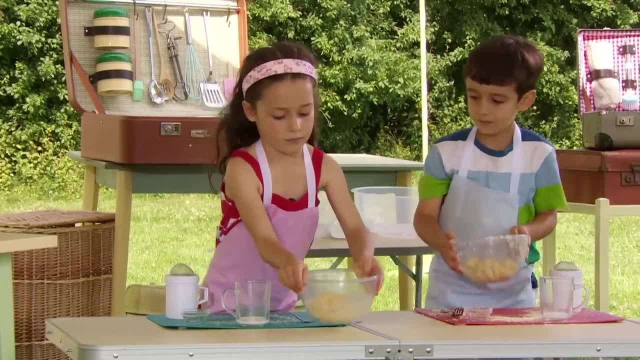 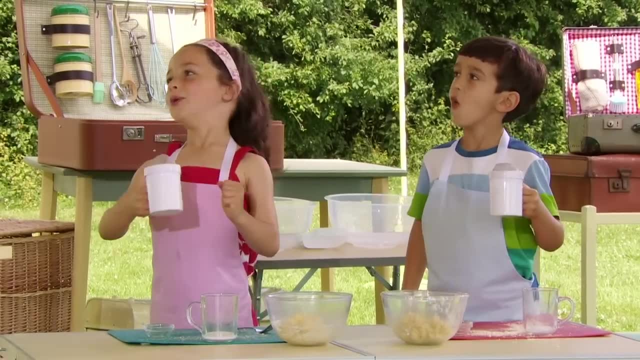 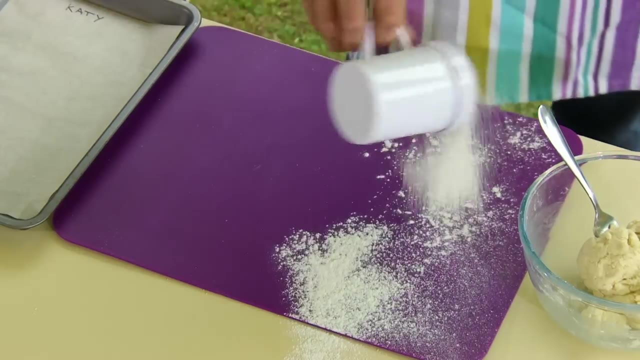 So let's put our dough mixture to the side for now, because we have to do something amazing. We've got to make it snow for the dough, So let's make a giant snowstorm. Three, two, one, Go, Whoosh. 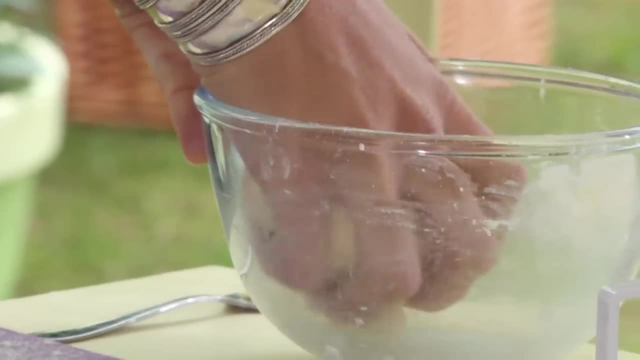 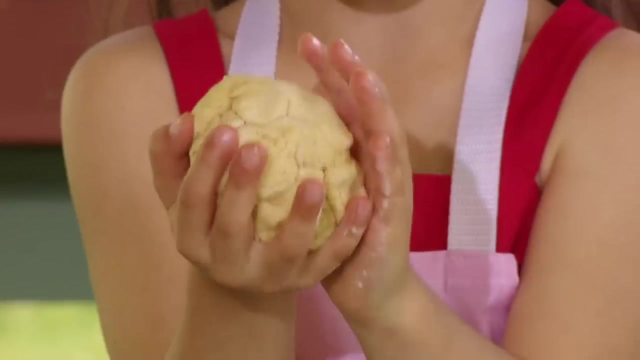 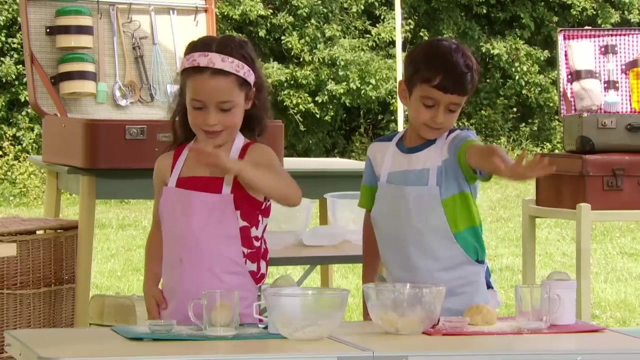 Brilliant. Now take your dough out of your bowl And we're going to make it into a ball. Can you see? that's a nice ball shape. Look at mine. it's nearly a ball. Mine is already a ball. Put your hand out like that and we are going to flatten our dough ball. 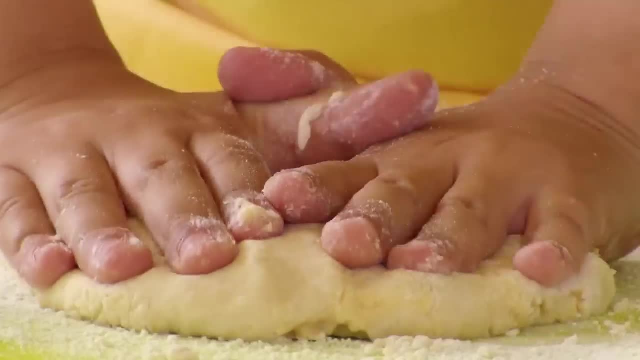 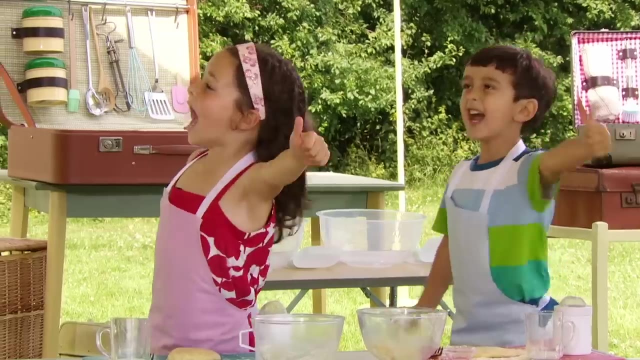 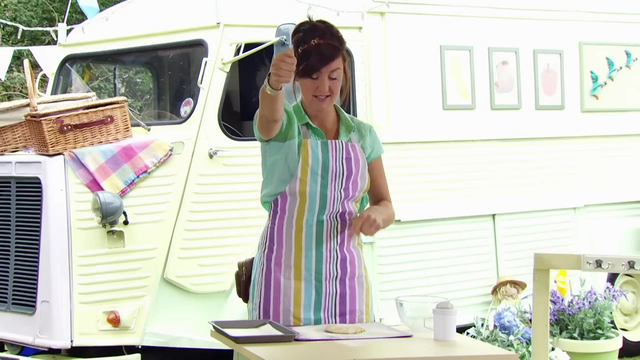 Squish, That's it. There we go. We've got a nice flat base for our fruit crown. I need you to put your thumb up like this and go: Yeah, Yeah, Now tuck your thumb in And we're going to use our knuckles to make a dip in the base. 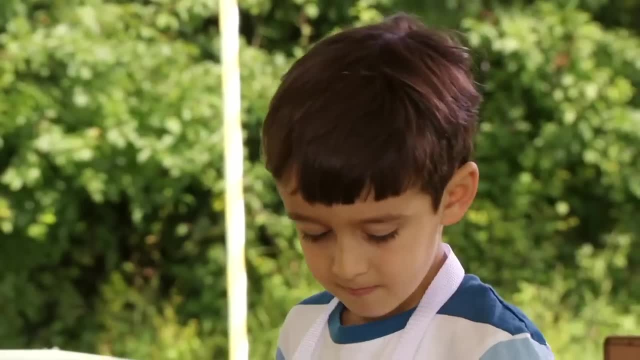 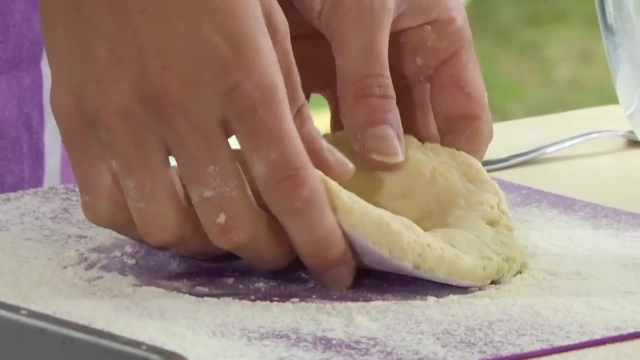 We do a few little dips like that. It should be getting flatter and flatter in the middle. It's a bit like a plate, And then we're going to pick our dough base up and put it onto the baking tray- Fantastic. 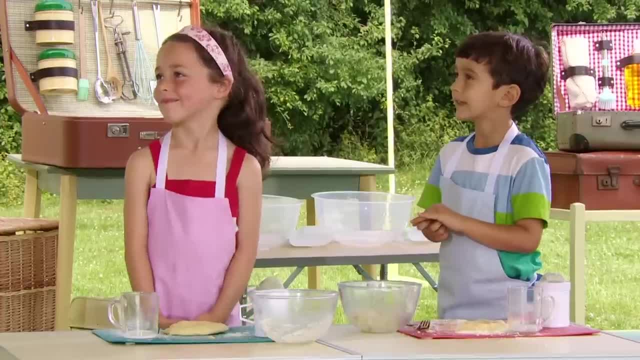 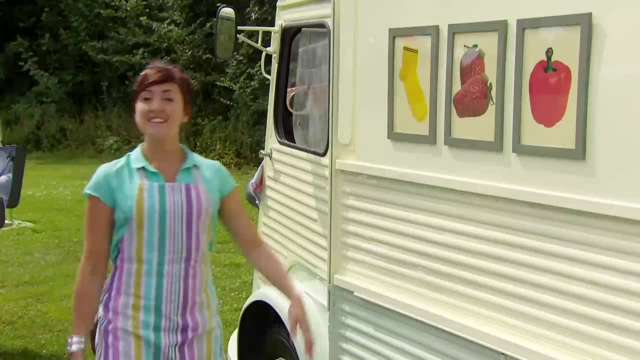 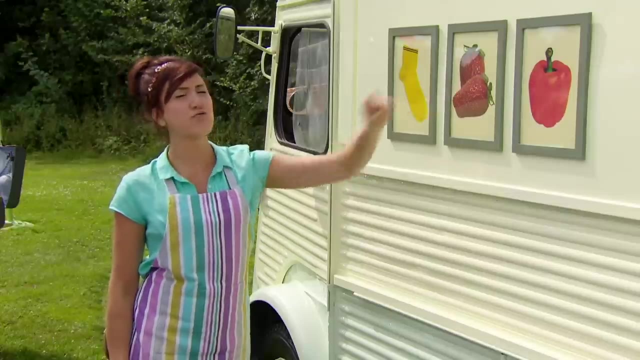 Now I wonder what ingredient we're going to need next. Well, let us see If you can guess what it could be. So we've got a yellow sock, some strawberries and a red pepper. What would you choose to go in our strawberry crown? 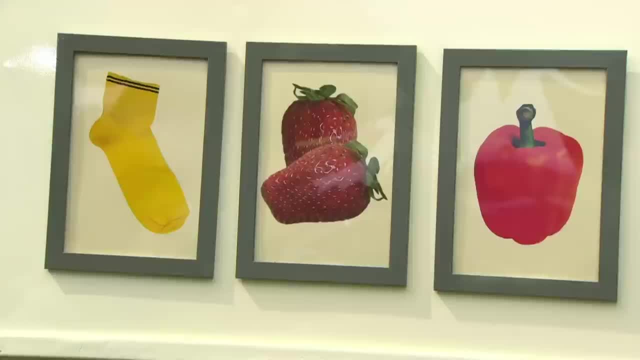 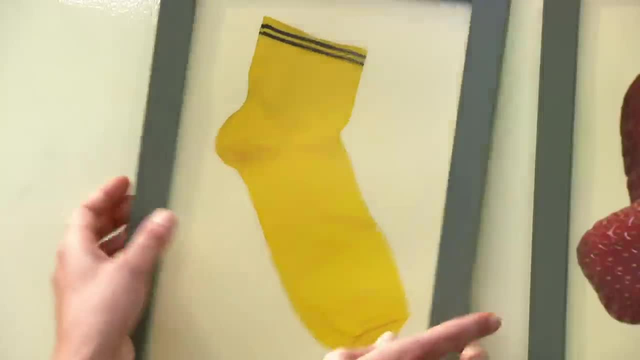 I'll give you some clues. The special ingredient is red, So it can't be a yellow sock. We wouldn't want to put a yellow sock in our recipe. No, thank you. The special ingredient is a berry. It can't be a red pepper, because that's not a berry. 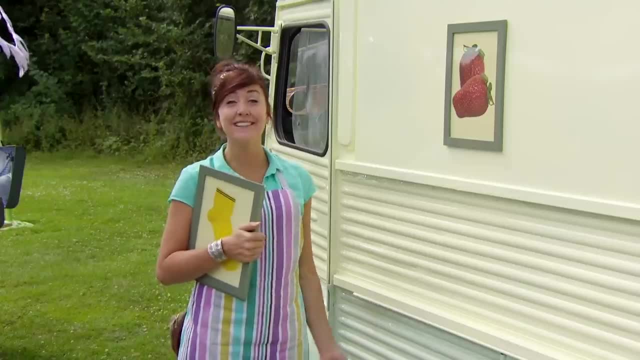 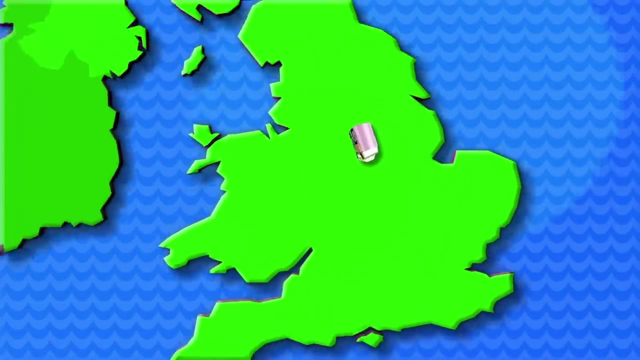 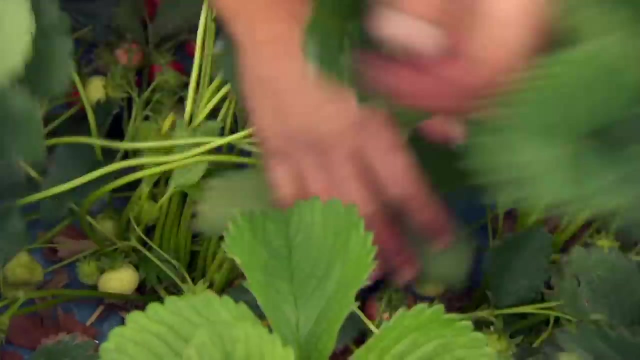 We'll take that one away. The special ingredient is strawberries. We're going to need them for our strawberry crown, And earlier I went to find some. I've come to Merryworth in Kent to look for strawberries. The strawberry plants in this field grow under plastic tunnels. 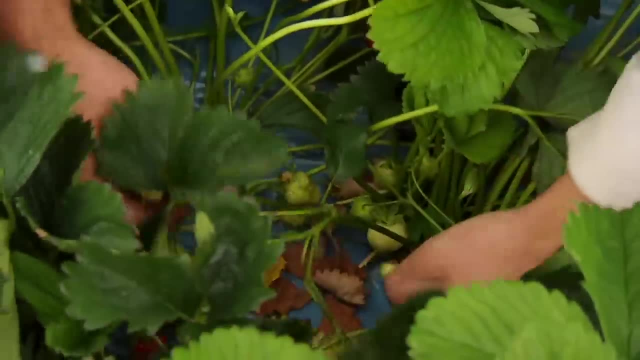 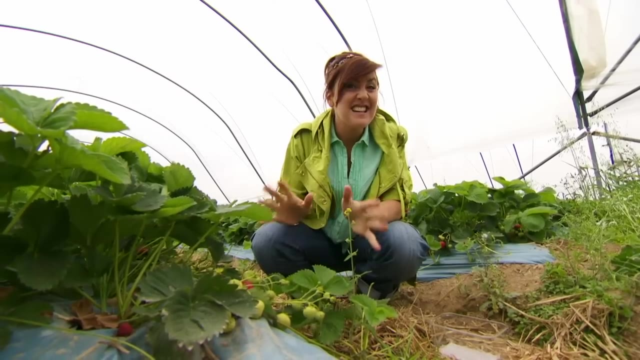 because they protect them from the wind and the rain and keep them a little bit warmer so people can pick them for longer. Now, when a strawberry is ripe, which means it's ready to eat, it turns red and big and juicy, just like this strawberry here. 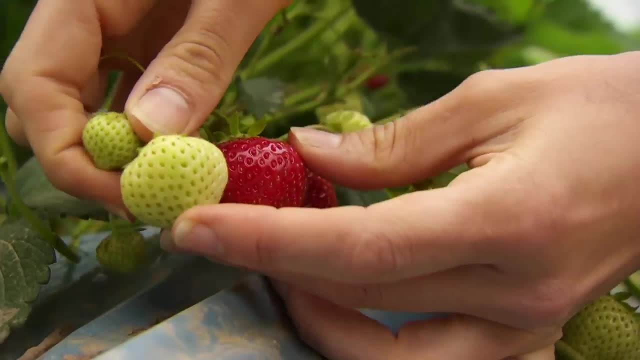 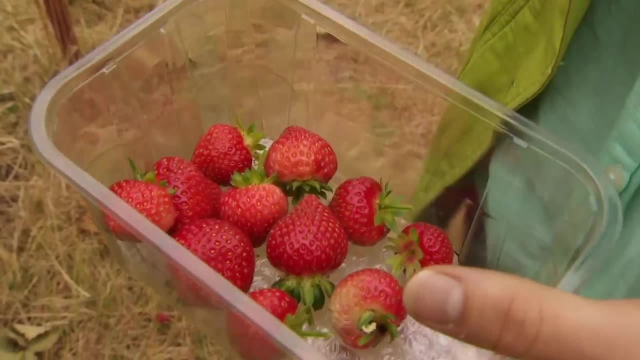 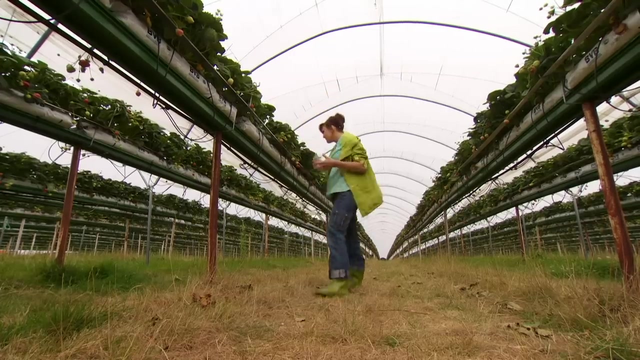 The one next to it is green and that's definitely not ripe. So we won't pick that one. We'll pick the nice red one. Let's go to another field where the strawberries grow in a different way. The strawberries in this field grow in bags on table tops. 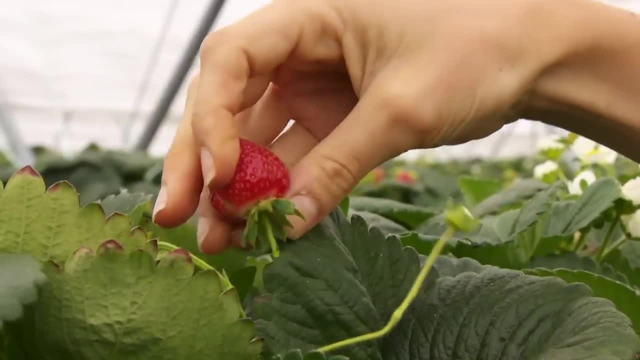 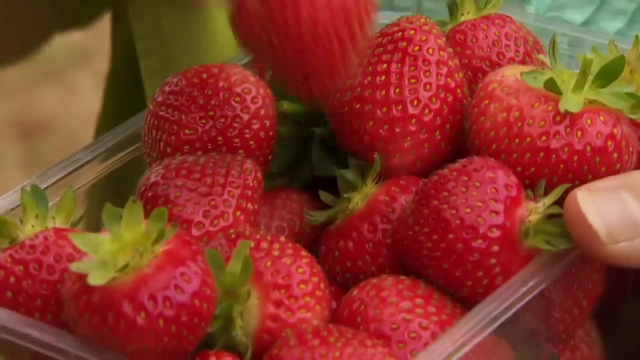 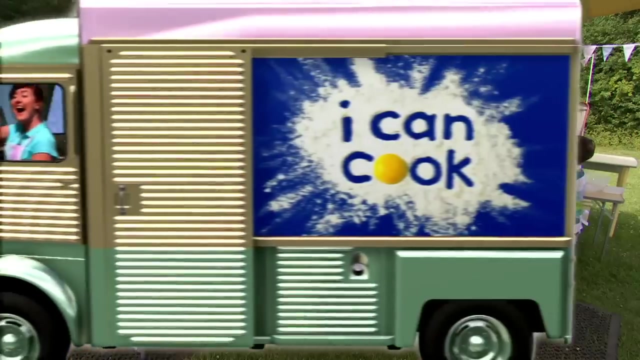 which makes them much easier to pick, and it keeps them healthier too. Oh, look at that one Yum. I think that's enough for everyone. Let's give these strawberries a wash and then use them in our strawberry crown. I've never seen so many strawberries in my whole life. 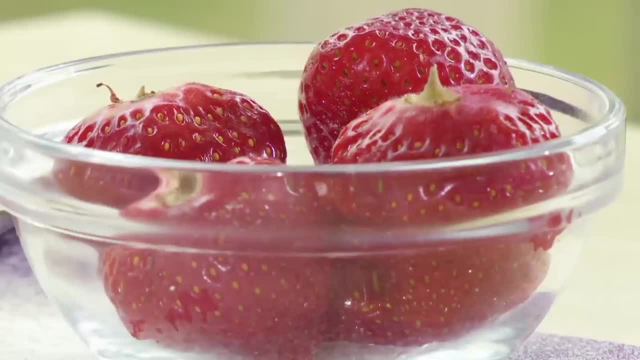 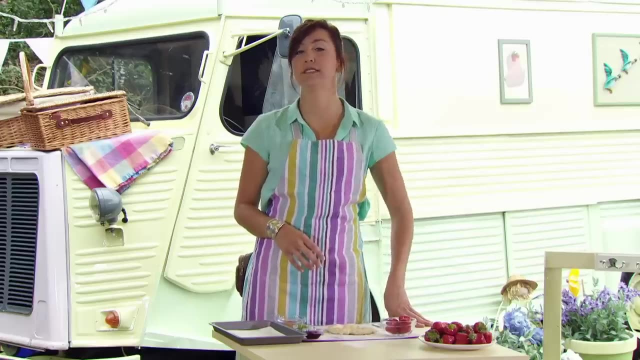 And now we've got our lovely ripe strawberries, so let's use them in the recipe. Now the first thing we need to do with our strawberries is some cutting. Some knives can be quite sharp, so you do have to be very careful. 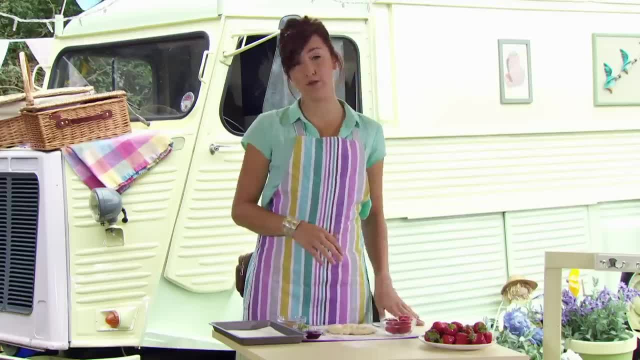 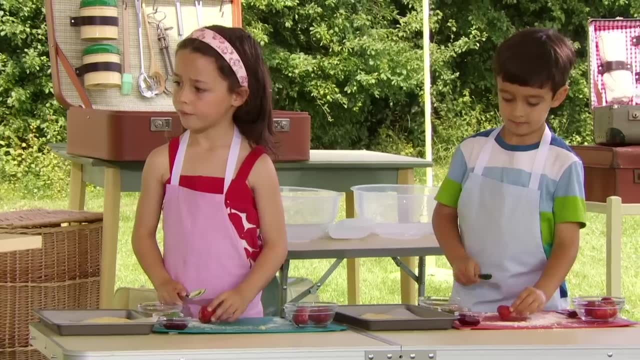 But a table knife is the kind of knife that you're used to using when you're at home and they're fine for us to use. Take the first strawberry and your table knife and we're just going to cut it down the middle very carefully, like that. 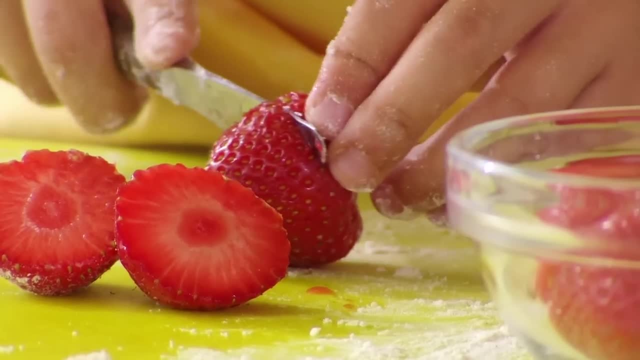 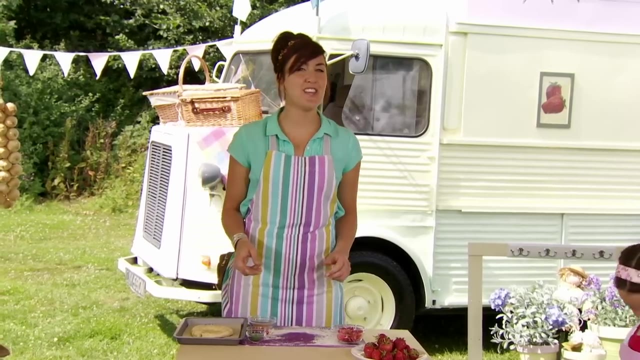 So keep doing that with all of your strawberries. Brilliant, So has everyone finished doing the cutting? Yes, The next thing we need to do is some spreading, and for that we need to use strawberry jam. We need to play the two-spoon game. 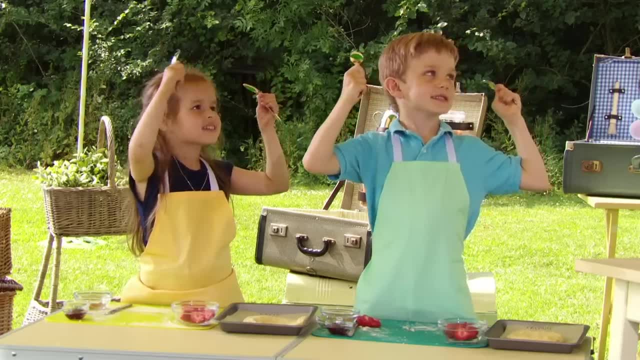 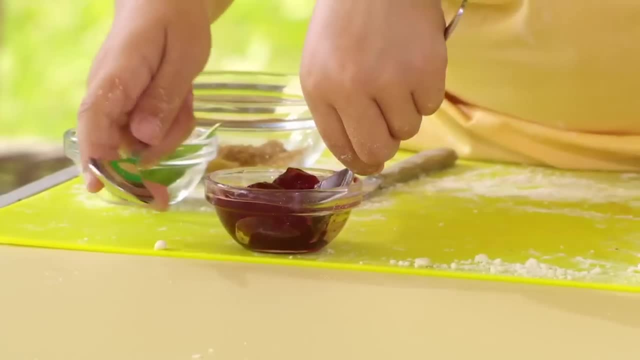 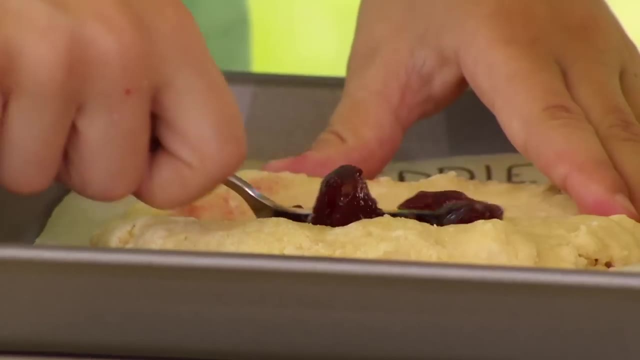 So pick up your two spoons- Yes, Give them a wave- And scoop up some strawberry jam with one spoon and slide it onto your dough base with the other spoon, like this Slide, And then we need to use one of our spoons. 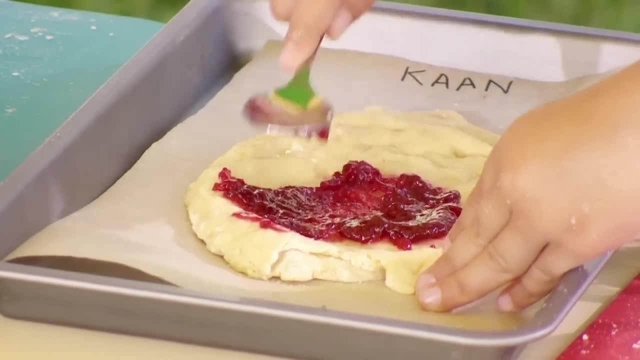 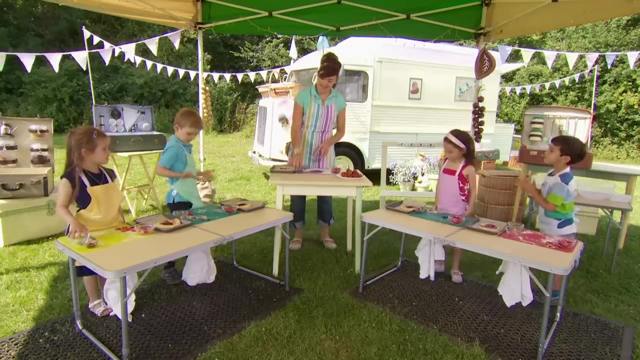 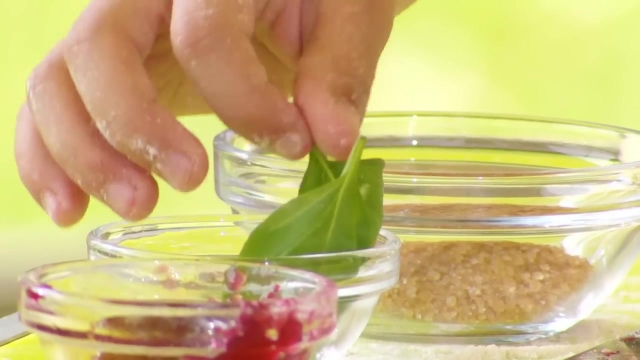 to spread the strawberry jam. So we make a jam, pond Spread, spread, spread. The next ingredient we need is this: Does anyone know what this is? That's a something that you can eat and it smells really good. That's right, and it's actually a herb. 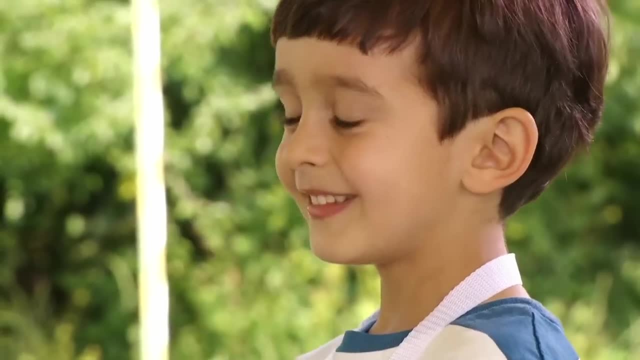 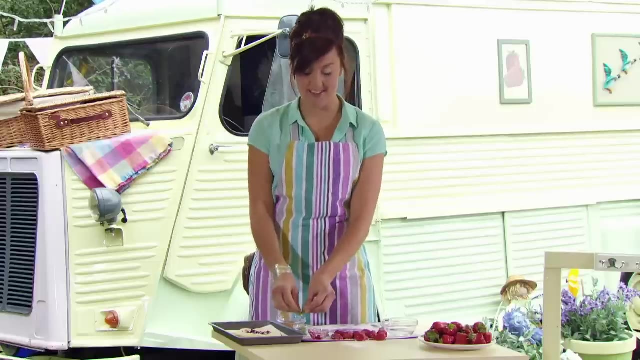 It smells really nice. I think it smells delicious, And we're going to tear and rip our basil leaves and put them onto our fruit crown. And you can join in with us too. You go like this, Tear and rip, Tear and rip. 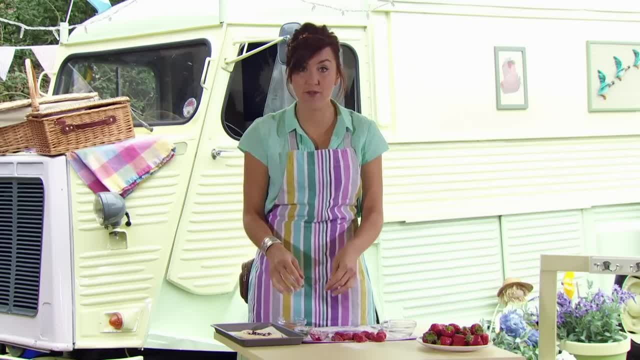 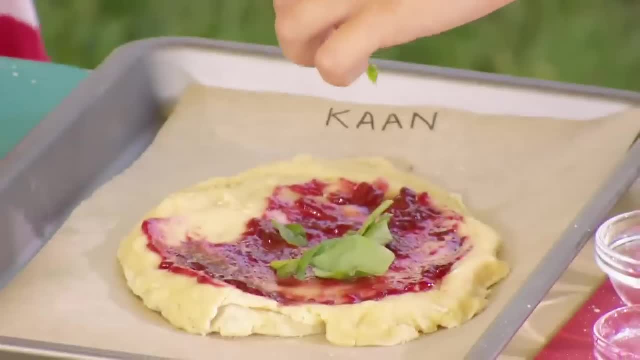 Now, we're not going to use all of these basil leaves just yet. We're going to use about half of them and we're going to sprinkle them onto our jam pond. It's time to add the crown jewels. OK, we've got all of our jewels. 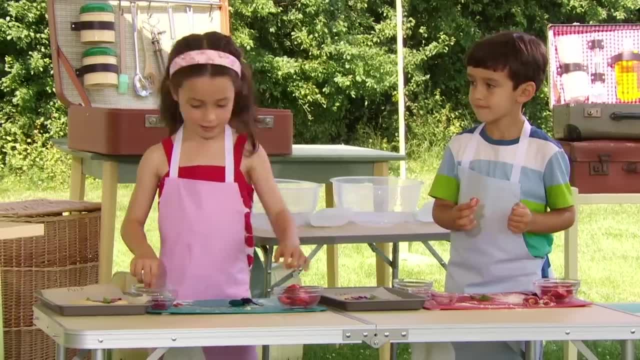 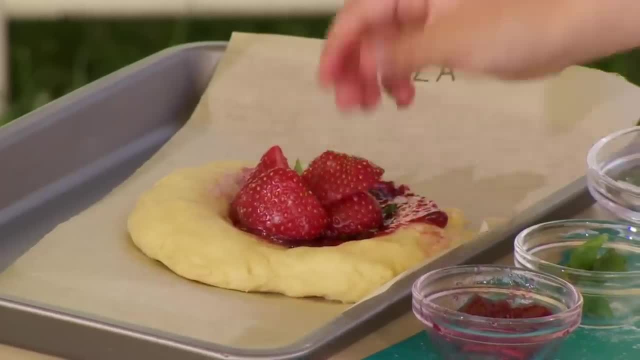 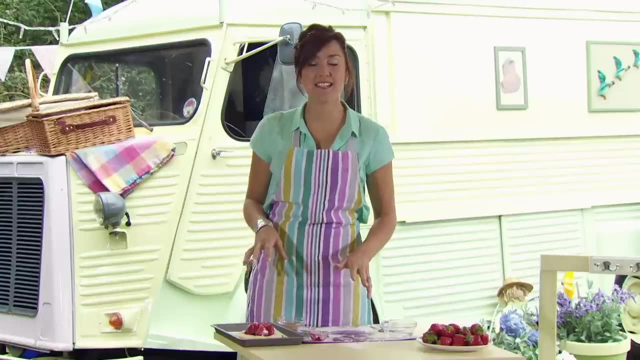 which are actually the strawberries in this bowl here, and we're going to arrange them onto our crown in whatever way we like, Somewhere outside of here, Somewhere outside and one in the middle. Yours is a crown fit for a king. Next, we need to sprinkle on the rest of our basil leaves. 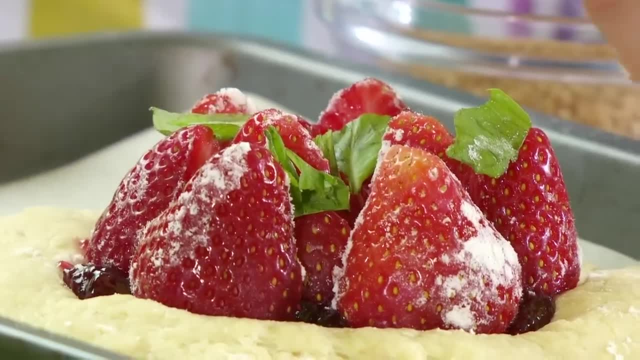 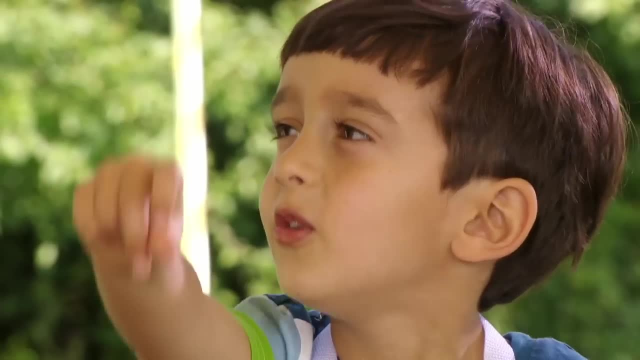 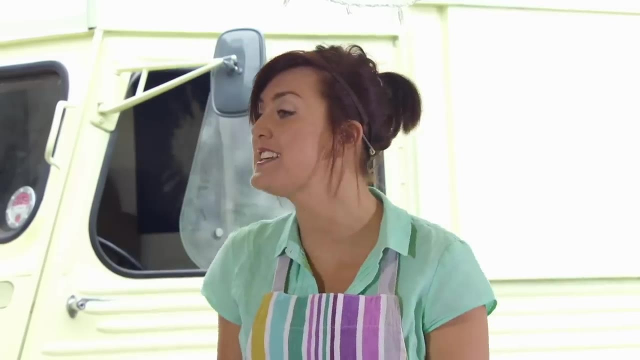 Sprinkle, sprinkle, sprinkle. There we go. Take a pinch of Demerara sugar and sprinkle it all over your strawberry crown. Demerara sugar, And that is it. You made it everyone. You put all the ingredients together for your strawberry crown. 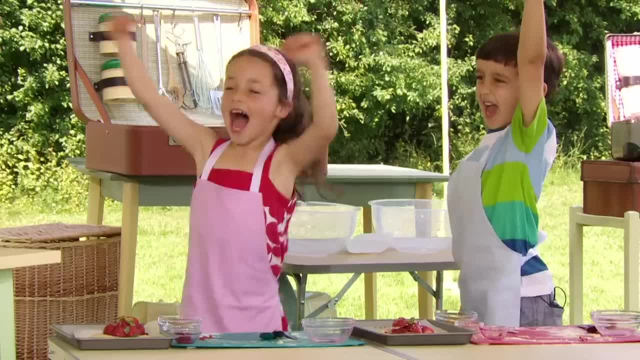 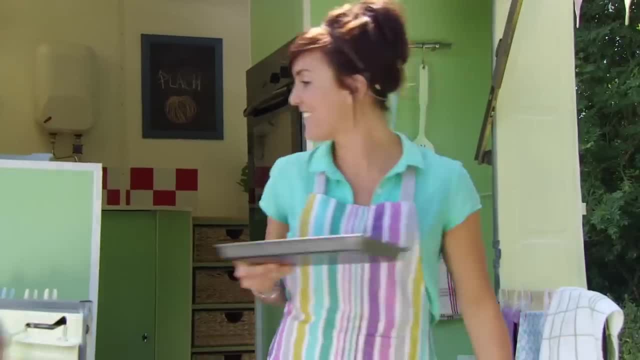 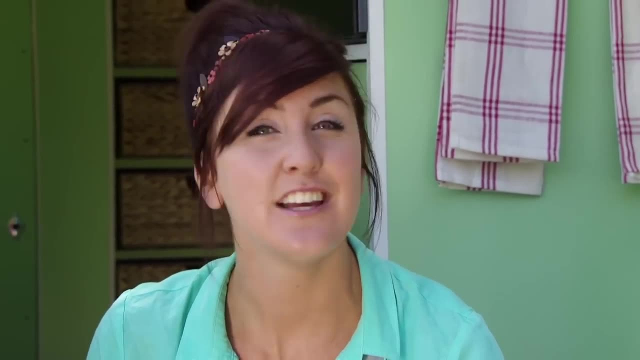 all by yourself. Yay, Yay, And now it's time to put them in the oven. Follow me Now. the food is about to go in the oven, But remember the oven is hot, so don't go near. You need to ask a grown-up to help you here. 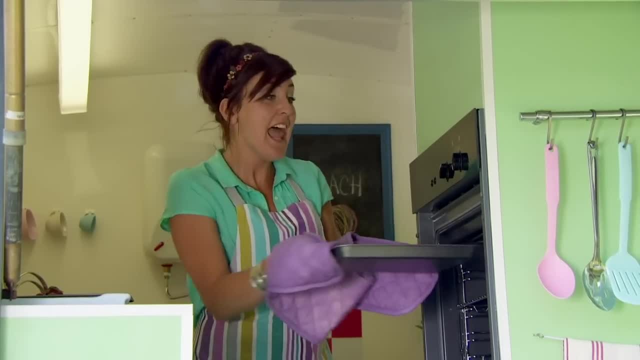 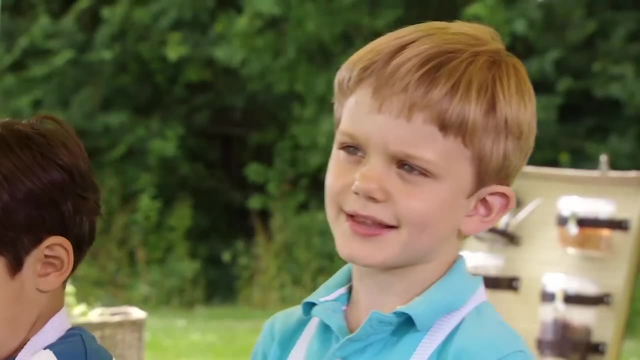 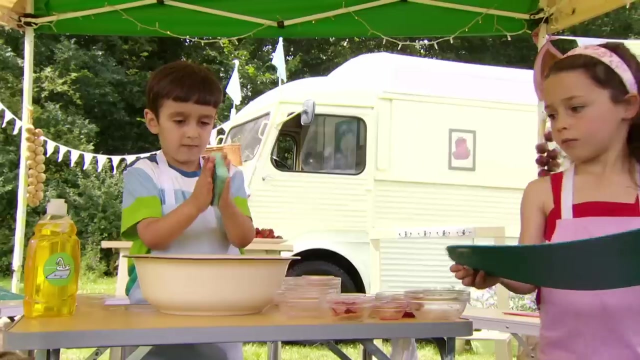 Now we've cooked with you and had lots of fun. Let's tidy up and think of all the things that we have done there: once Mix it, Pickling, Wedding Wearing, And now clearing any mess and putting things away is always fun to do at the end of the day. 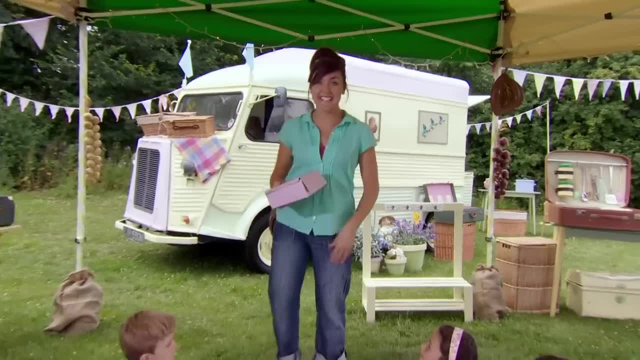 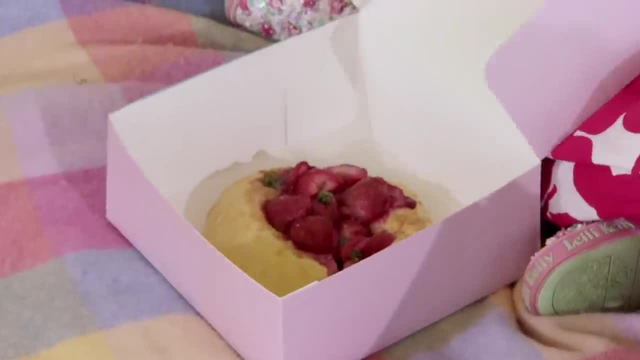 And here they are, all ready to eat. You've made your very own strawberry crowns Pula. let's have a look at yours. Wow, that looks scrumptious. What do you like most about the strawberry crown- Strawberries. 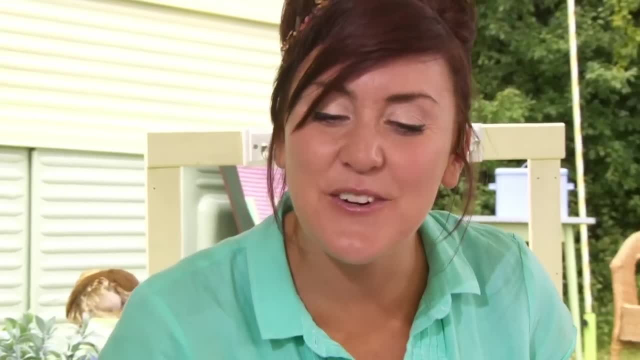 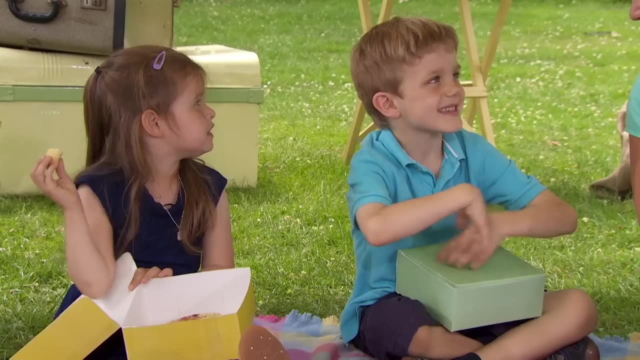 That's right. you love strawberries, don't you? Yeah, And Katie, let's have a look at yours. That half bit looks like a pizza coming out. Do you think your friends and family are going to like them? Yeah, Now let's put the lids on and save them for later. 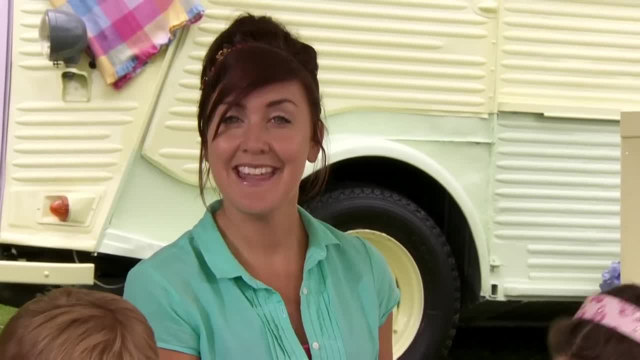 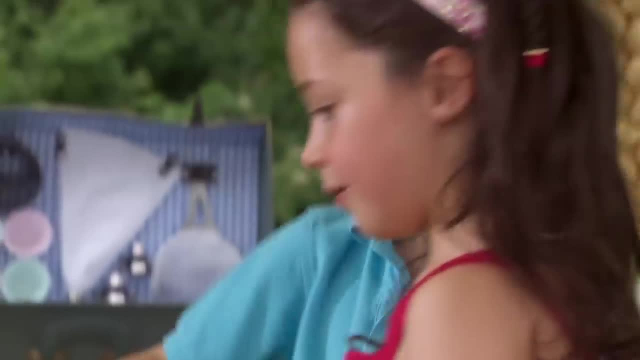 We've travelled to you, cooked and had fun. Now let's have a party with everyone. Yeah, Come on, everyone, follow me, And you can come too. Come on. Well, here we are by the castle, and I don't believe it. 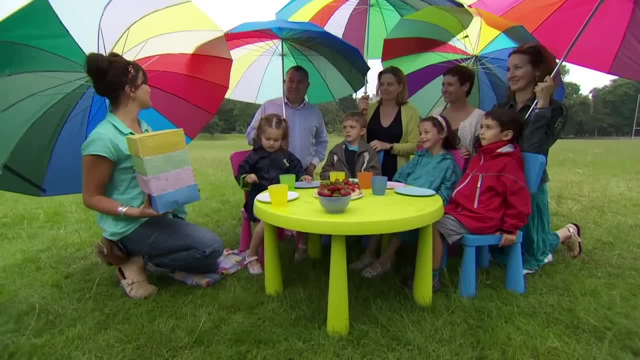 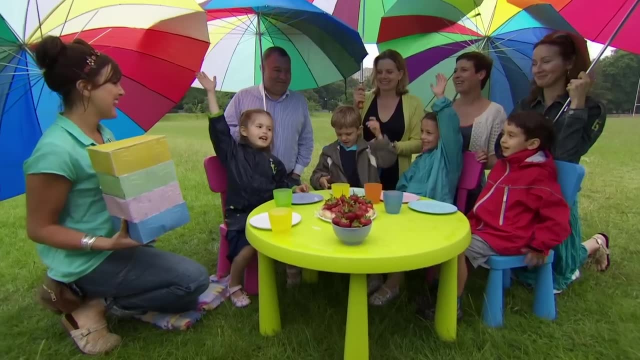 but it's raining again. But that is not going to stop us from having a picnic, is it everyone? No, I've got one question: Who is hungry? Me, Oh, me too. This is so funny, And we've made some extra for all your family too. 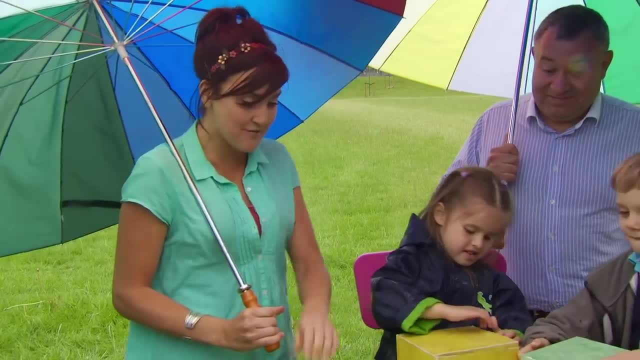 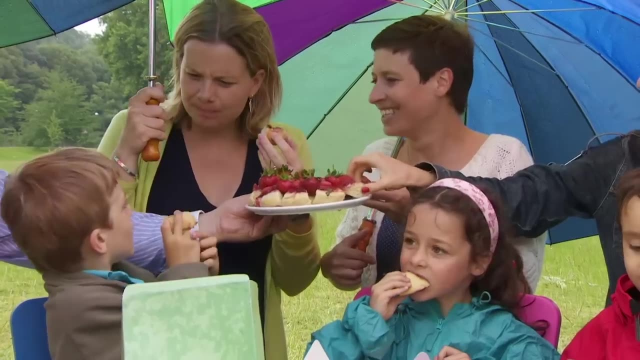 So let's dig in and eat our strawberry crowns. Here you go everyone A little bit soggy, but I'm sure it'll taste delicious. Mmm, Lovely Pula. what does it taste like? Sweet? Do you know what the best part of the day is for me? 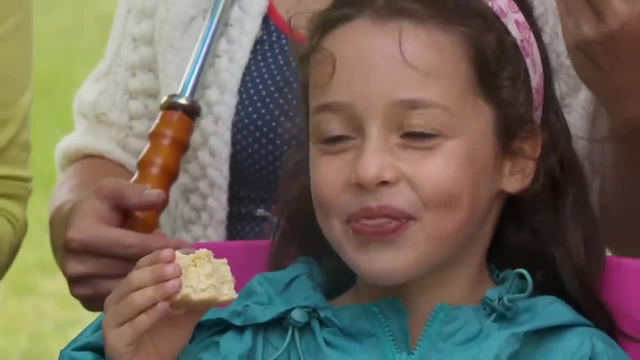 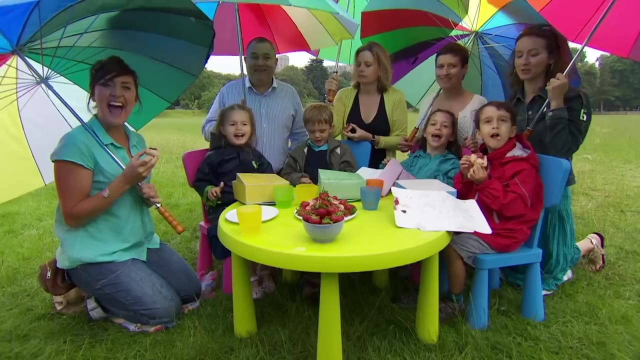 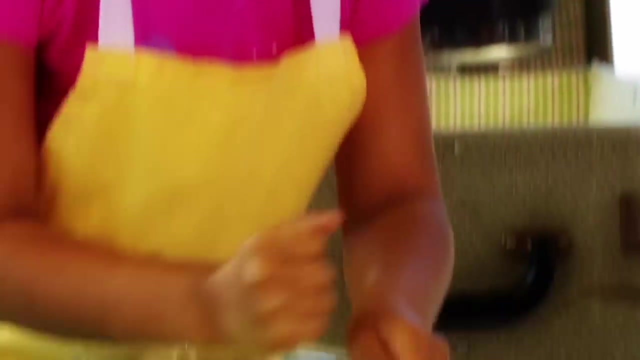 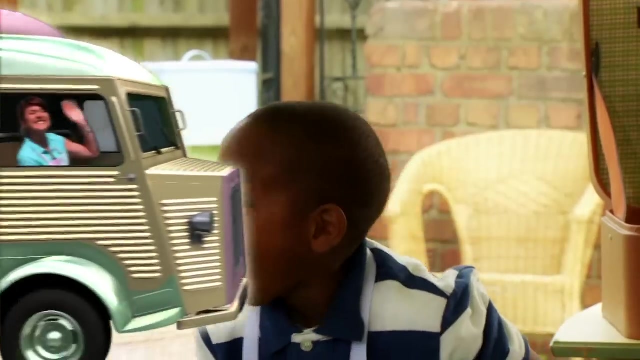 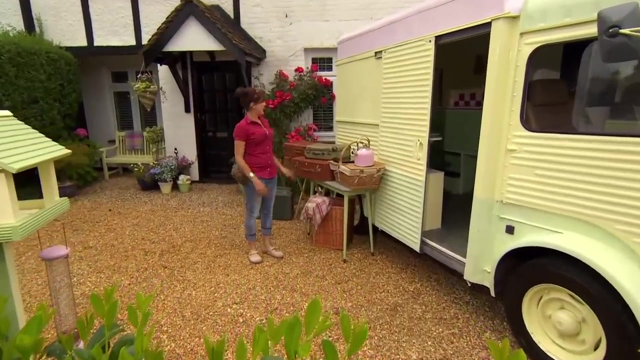 The rain. That's good. no, Mmm, That's delicious. So, everyone, what can you do? I can cook, I can cook, I can cook With you. Ah, hello, Lovely to see you. I've just got everything ready to go on a journey. 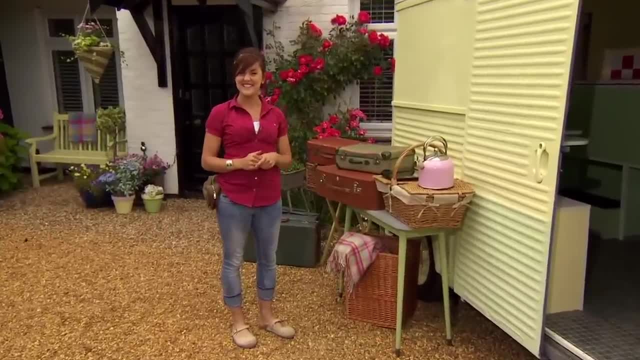 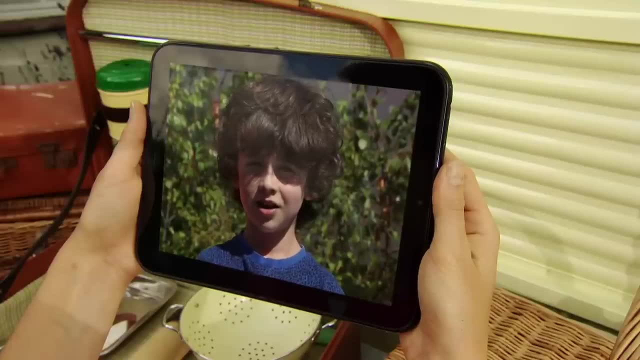 and I really hope that you're going to come with me and meet some new friends. Ah-ha, Hi, Katie. I love skateboarding with my friends. Can we make something yummy with courgettes? Definitely, That will be so much fun. 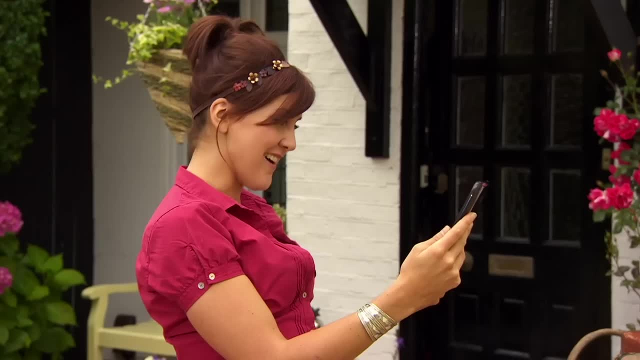 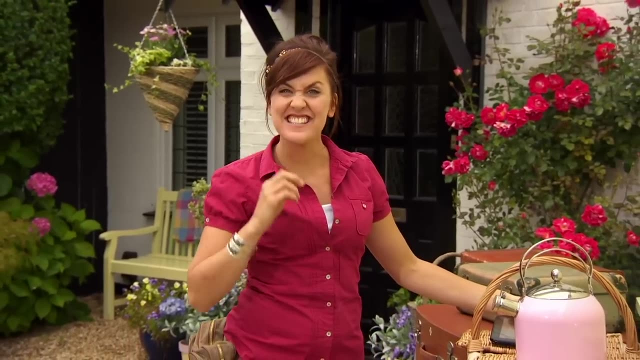 Katie, can you come with us? Katie, can you cook with me please? I can, Cosmo, And you can cook with me too. Oh, I wonder if I'll get to have a go at skateboarding. I've never tried it before. 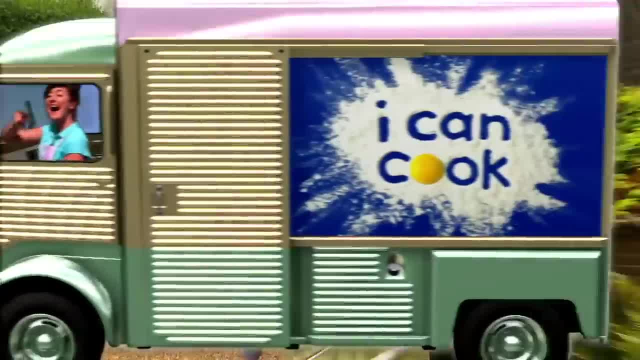 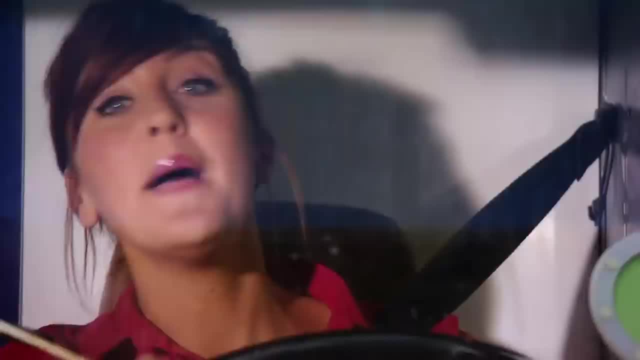 Right, let's get everything packed up and be on our way. I'm on a journey and I'm coming to you. It's going to be busy and there's lots to do. Get ready to help, join in and have fun. Let's cook a feast for everyone. 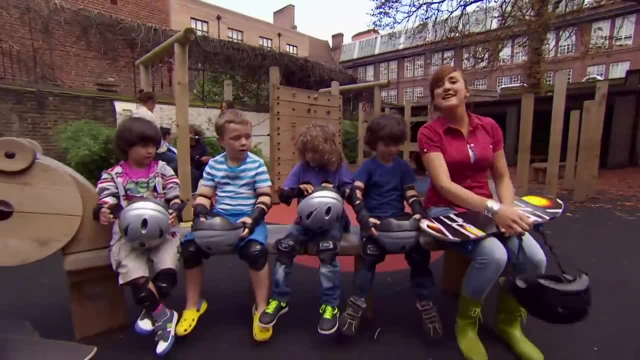 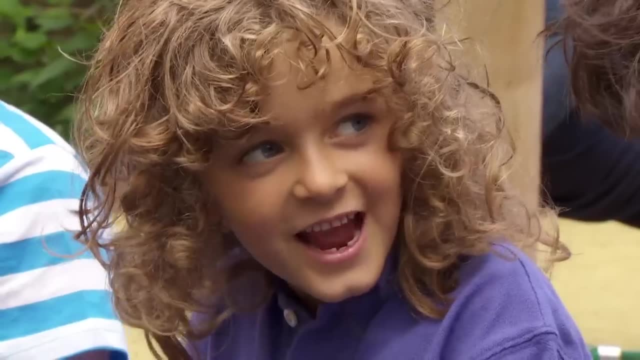 Well, I've got my skateboard and I'm ready to do some skating, and I just found Cosmo and all of his friends. Hey, Cosmo, Hello. So what's your name? Hey, I'm Paddy Nasa. 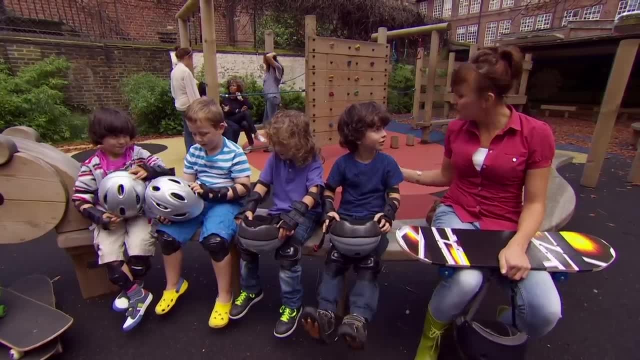 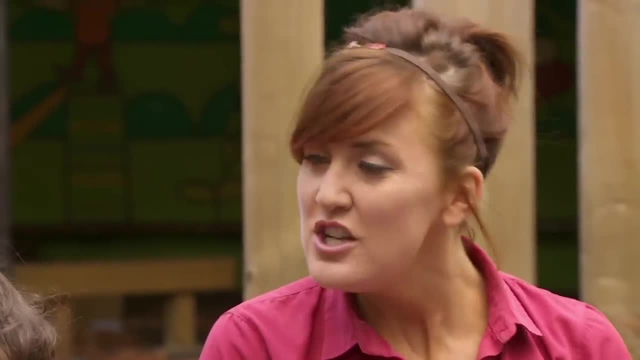 Cool. well, it's so good to meet all of you. I'm really excited. What are we going to do today, Cosmo? Can we make something with courgettes and go skating? You bet we can. Cosmo, Do you want to join in too, everyone? 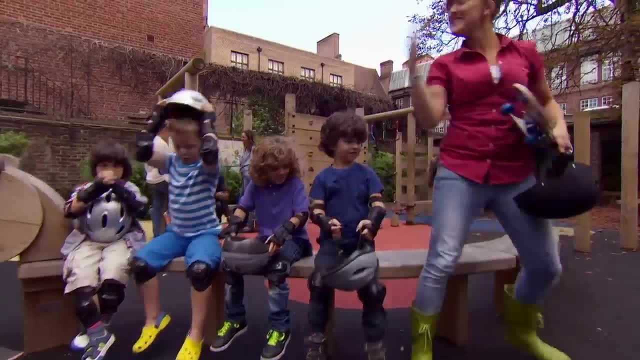 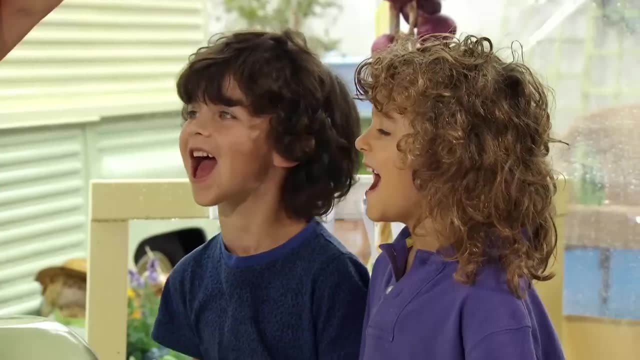 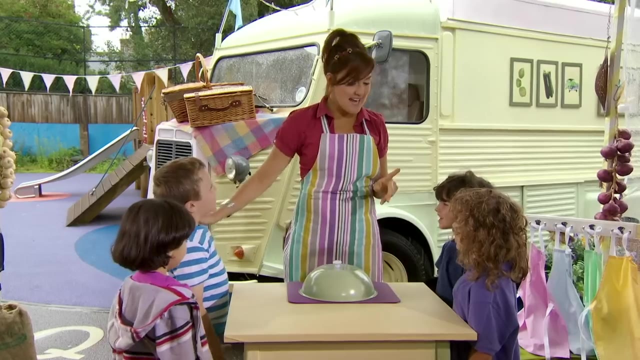 Yeah, Brilliant. OK, follow me, let's go This way. Welcome to my outdoor kitchen. Yay, Who wants to know what recipe we're going to cook today? Me All right. today's recipe is delicious: It's Katie's courgette cake. 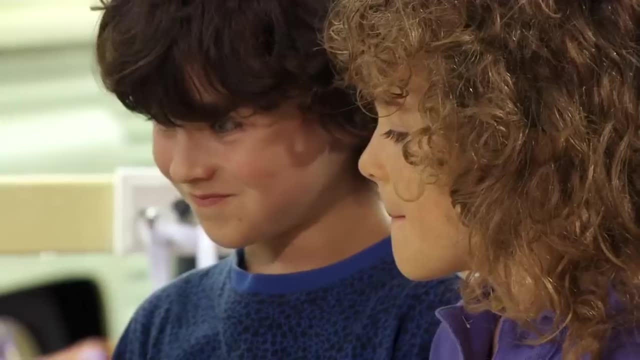 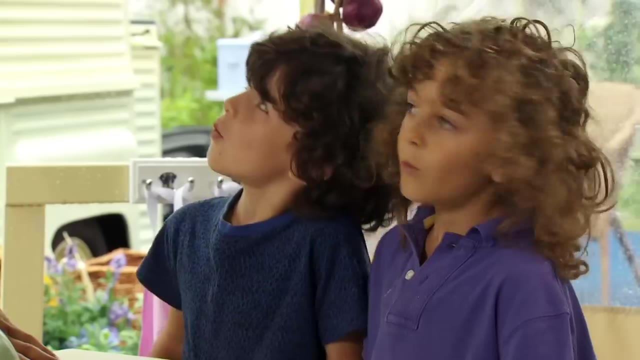 Look at this. But before we get started on the cooking, we've got to do something really important first. What do you think it is? Wash our hands. You've got it. We need to wash our hands. Come on, let's get going. 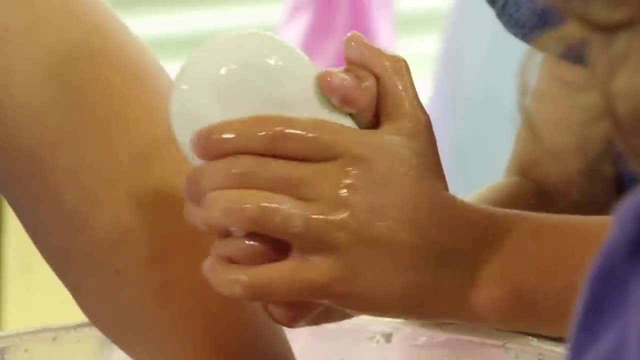 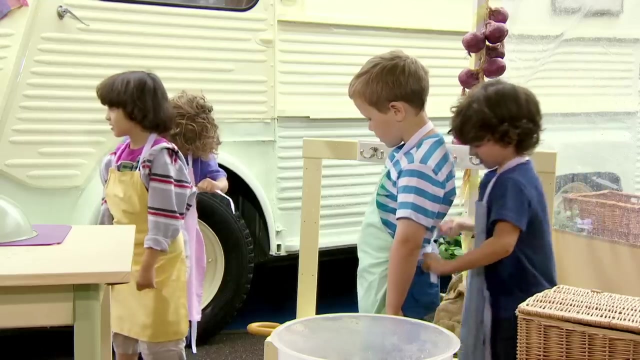 Roll up your sleeves. give your hands a wash with slippy-dippy soap, splish-splash-splosh. Have you done? your hands Washed and dried sleeves rolled up, apron tied. What can you do? I can cook. 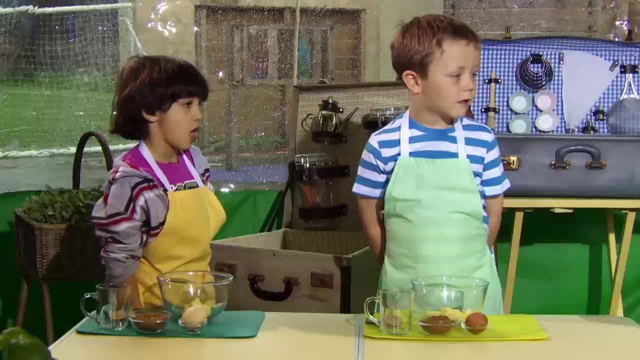 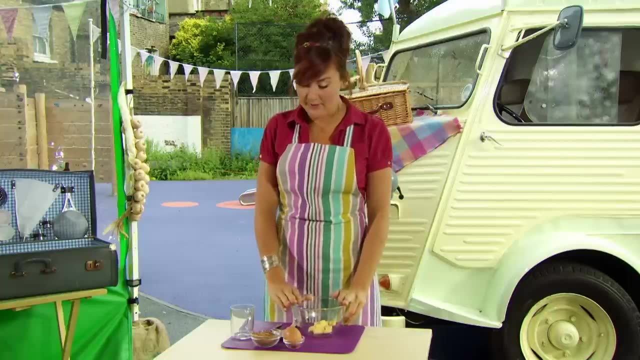 Right, let's get started on Katie's courgette cake. The first thing we're going to need is some soft butter in a bowl, And to our soft butter we're going to add some soft brown sugar, But this is a really special sugar actually. 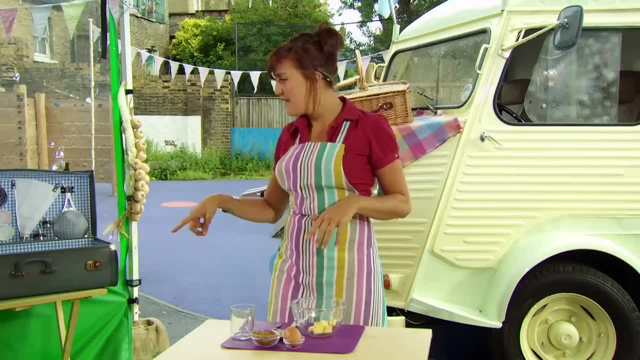 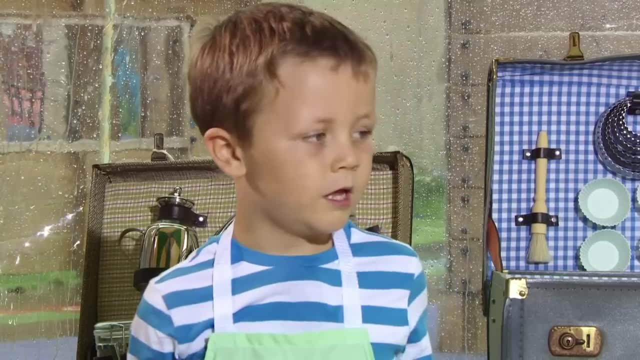 It's got a really nice smell. Why don't you smell the sugar and tell me what you think it smells like? It smells like raisins. Oh yeah, it is like raisins actually. Right, let's add the sugar to the butter in the bowl. 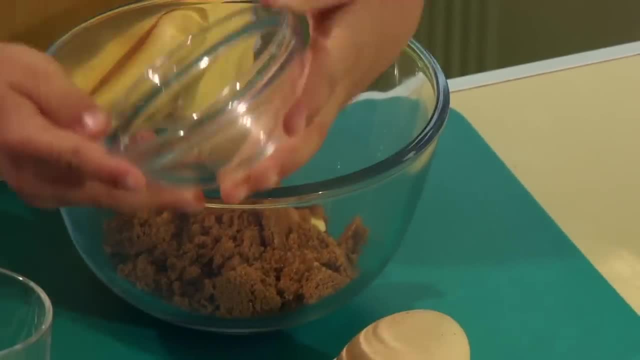 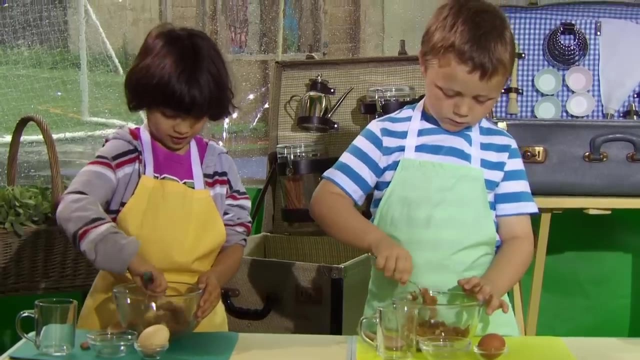 Mmm, And when you've added it, we're going to use our fork. We're going to use our fork to do some squishing. I knew it. Squish it up against the side of the bowl. Look, squish squash, squish squash. 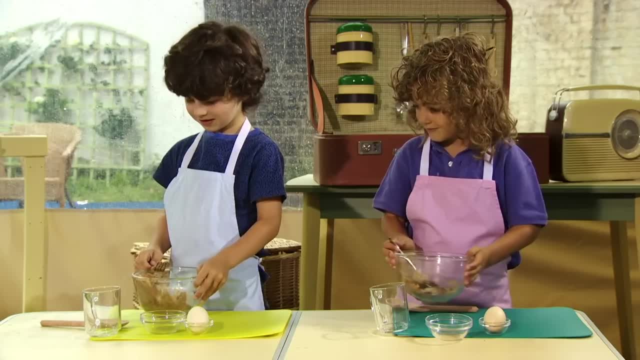 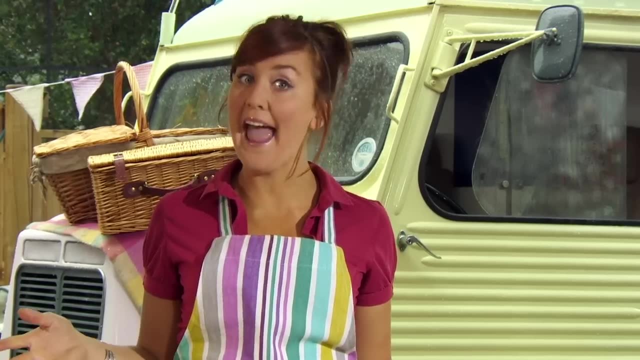 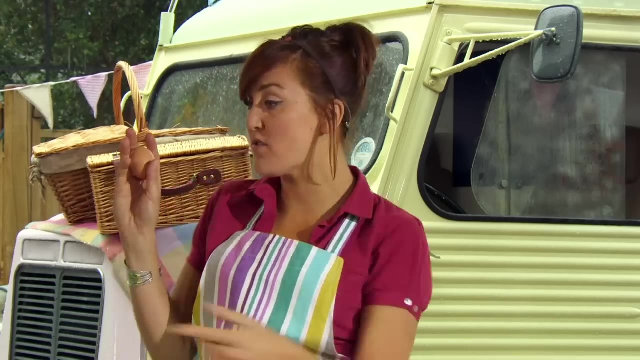 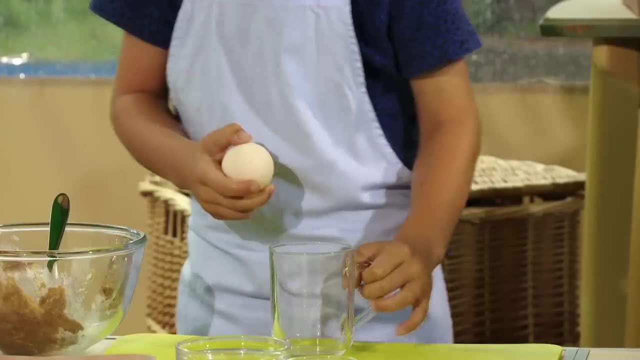 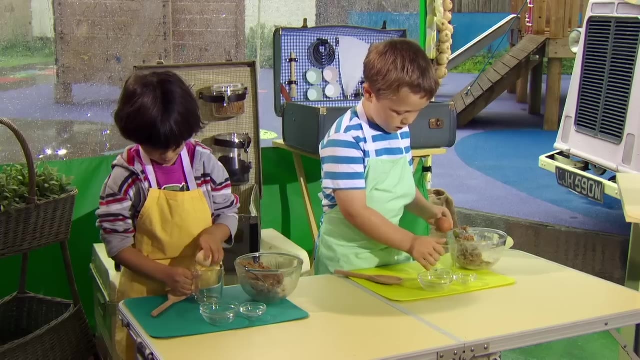 Come on, let's crack this egg. Okay, so we hold the handle of the cup And then we have to knock on the door. So knock, knock, knock, Make a crack, Knock, knock, knock, Then use your thumbs to open it up. 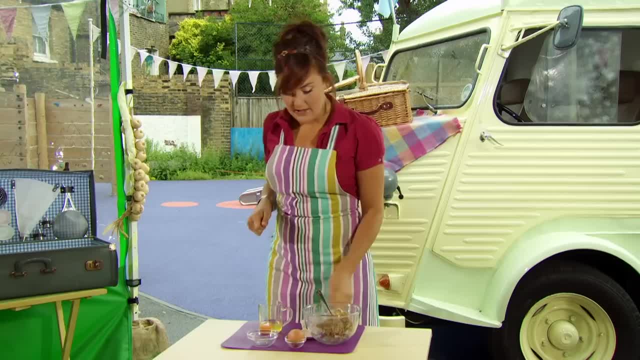 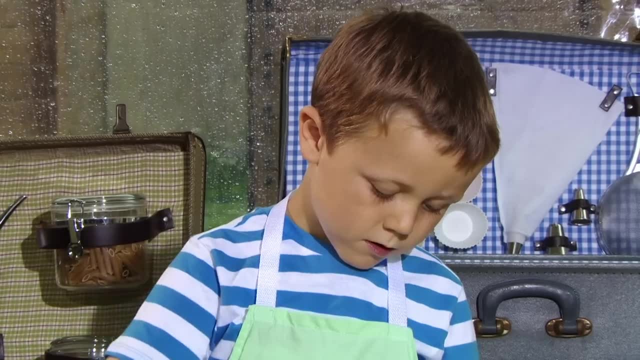 And open it up into the cup. That's it. Now we're going to use our fork again to whisk this egg up, So we just scrape off the sugar mixture. That's it. So you hold the handle and you can join in with this too. 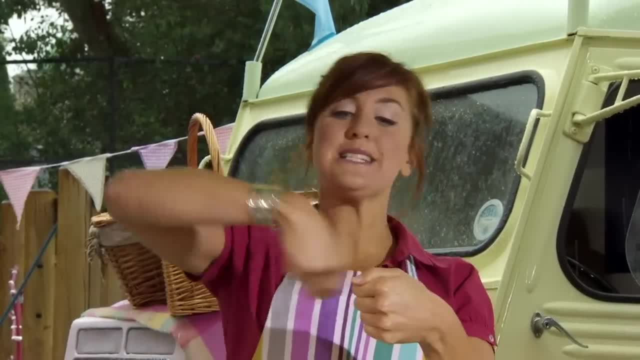 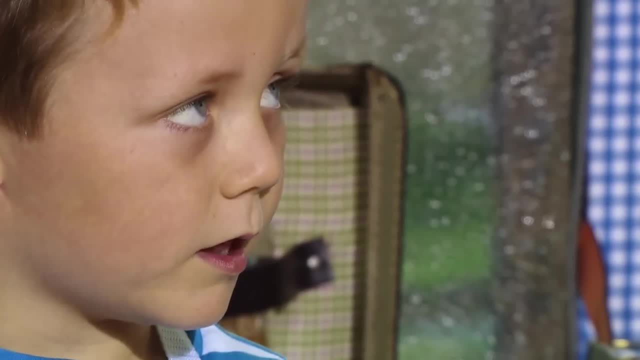 Get your cup and your fork and go like this: Whisp, whisp, whisp, whisp, whisp. What's happened to your egg? It's like orange juice, But we wouldn't want to drink this, would we? 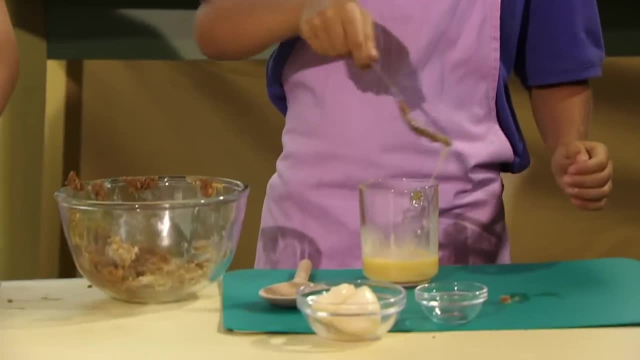 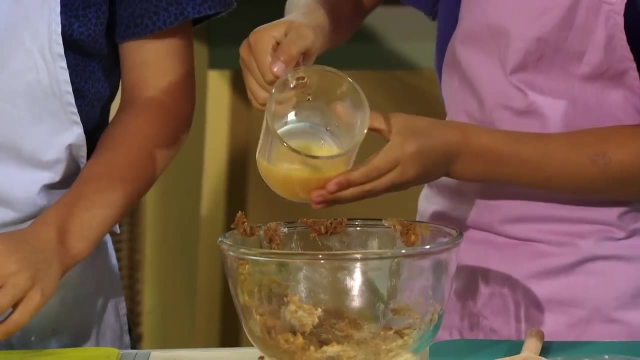 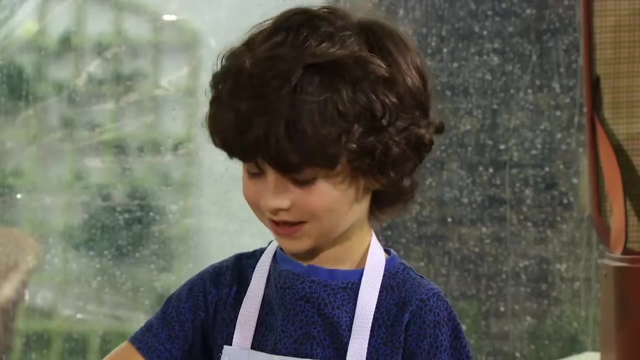 And put your forks down, because we're going to pour this eggy mixture into our sugary mixture. So let's whoosh it in after three, One, two, three, whoosh. Oh, the egg is swimming around the sugar. Let's use our wooden spoon to mix it together. 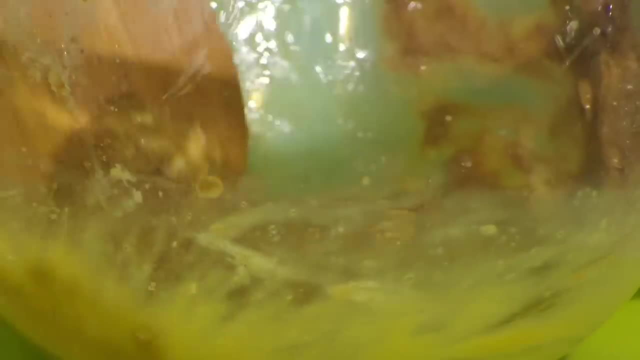 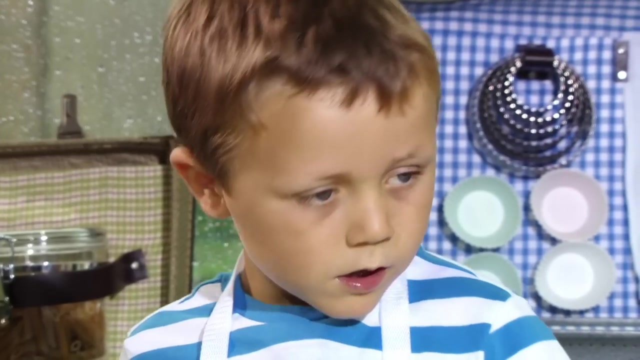 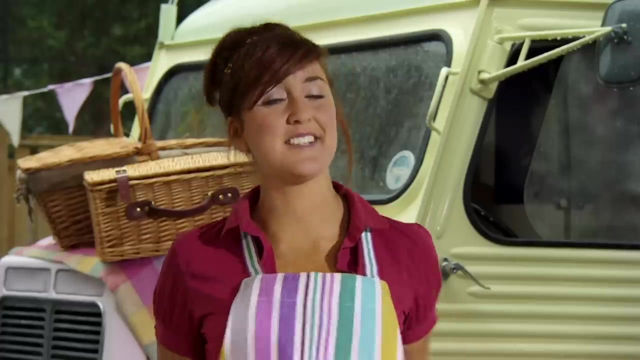 Keep mixing. everyone that's- it Is mine the muddiest, Yes, And everyone. stop mixing. I wonder what ingredient we're going to need next for Katie's courgette cake. What's next? Well, let us see if you can guess what it could be. 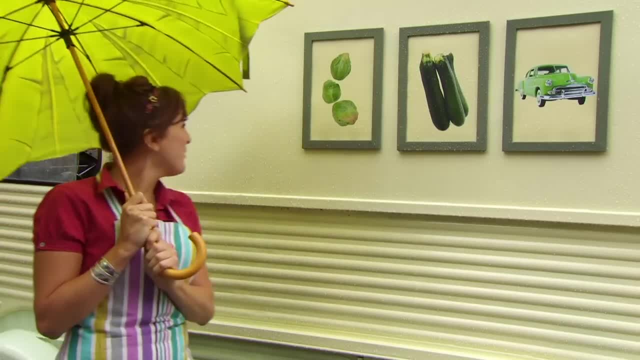 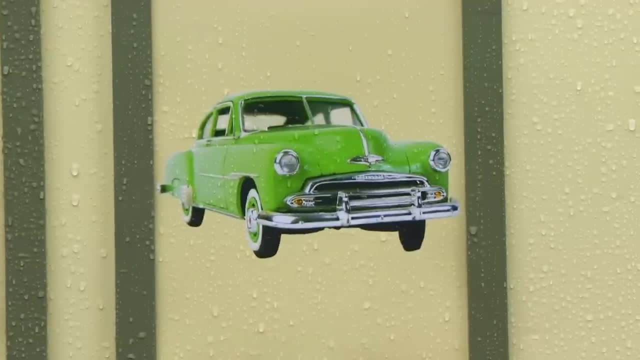 So what have we got? Some Brussels sprouts, some courgettes and- oh, a very nice green car. What would you choose for Katie's courgette cake? I know I'll give you some clues and then you can guess what it might be. 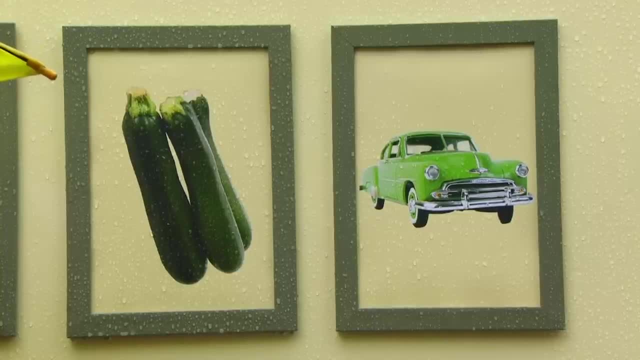 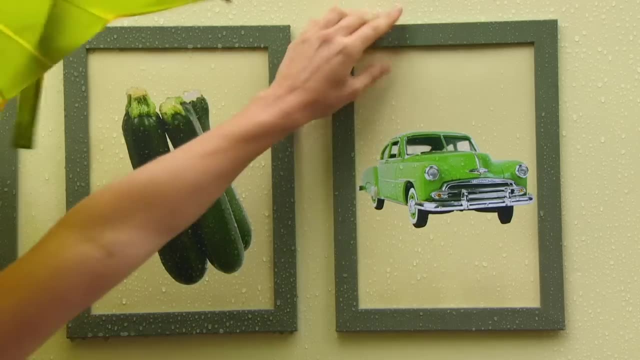 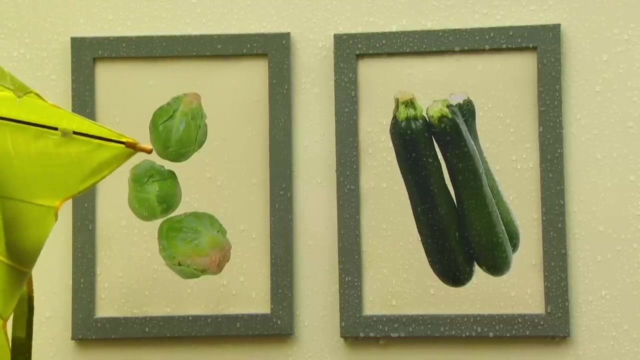 The special ingredient is green and it's a vegetable- A car. Well, that car's green, but it's certainly not a vegetable, is it? So we can take that one away. Here's another clue: The special ingredient is green and it's a vegetable, and it's long like a cucumber. 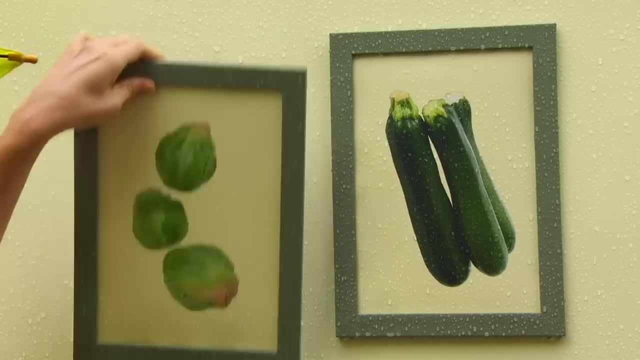 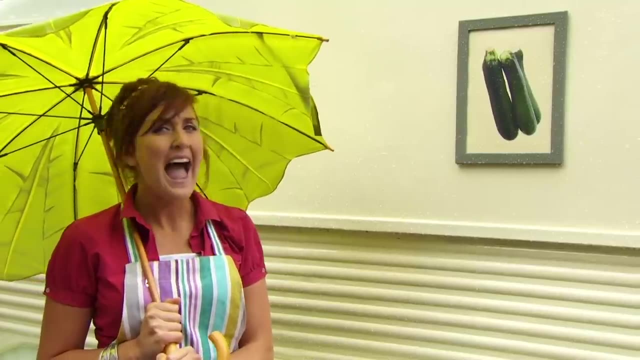 Well, Brussels sprouts are round, aren't they? So we can take that one away too, which leaves us with courgettes. We're going to need some courgettes- for Katie's courgette cake, of course, And I went to find some. 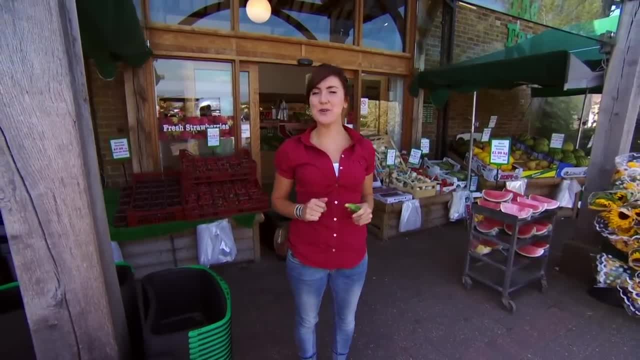 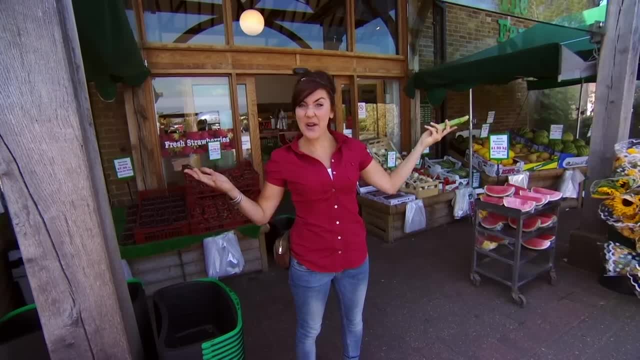 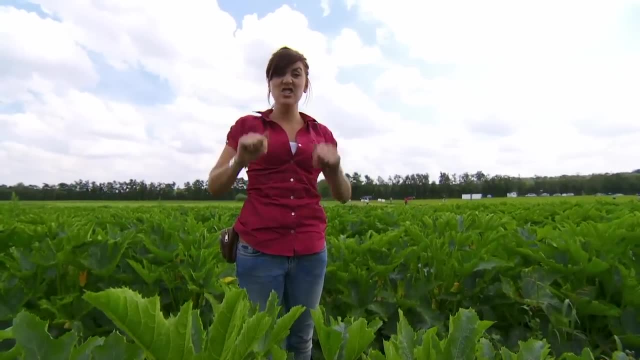 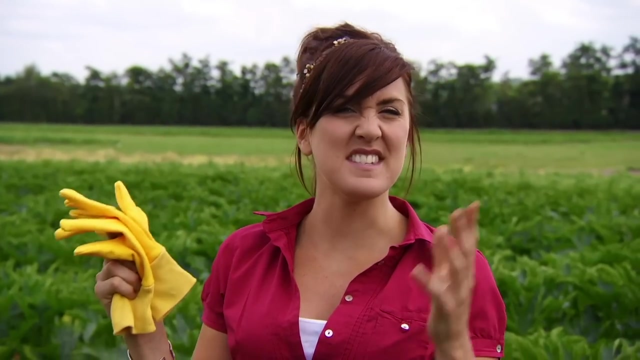 Now, this is what we're looking for, so let's go. And here they are, the courgette plants. and the courgettes are hiding just down here, So let's pick some. Now I'm going to wear some gloves, because the stems of the courgette plant have tiny little spikes on them. 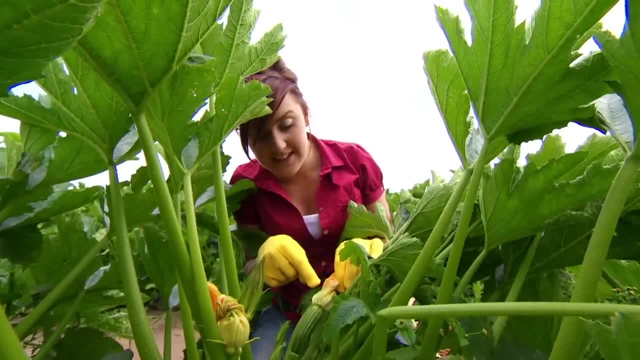 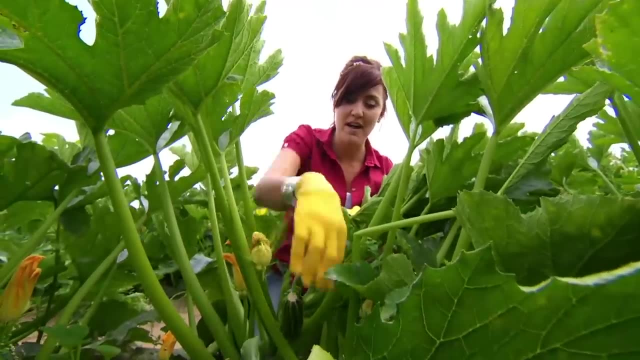 Look at this, This courgette. it's got a flower growing on the end of it, And actually you can eat that flower if you want to, but this one isn't quite ready to pick yet. Oh look, this one, on the other hand, is perfect. 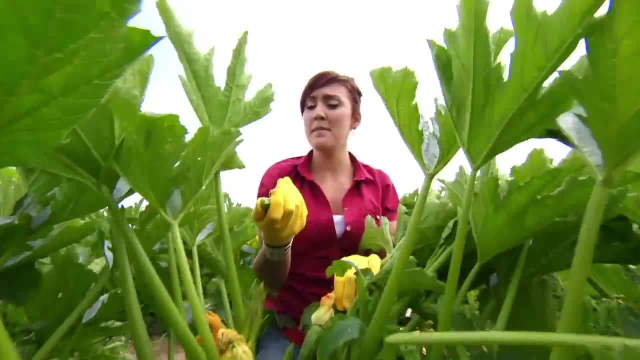 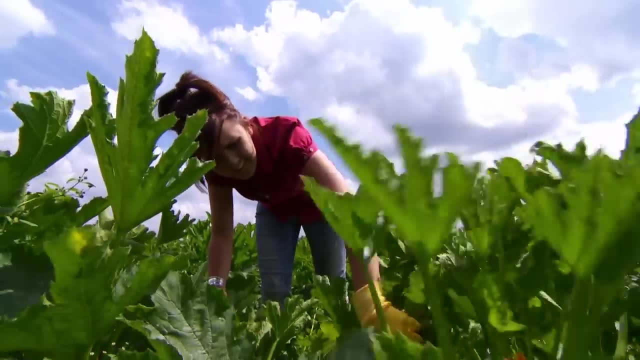 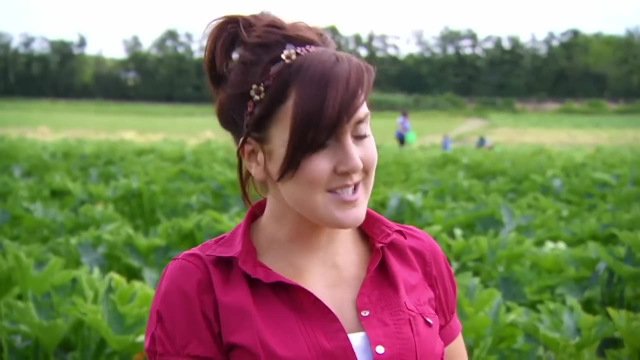 So I'll pick that one and put it in my basket. Yep, I think that'll be enough for everyone. Now I just need to give these a wash and they'll be perfect. They're ready for our courgette cake. 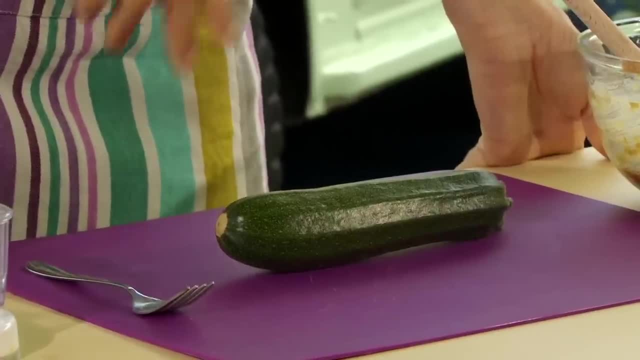 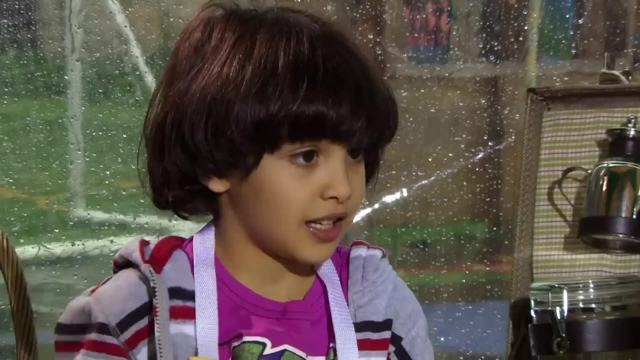 Those courgettes were actually quite hard to find, but we got some and they're here to use in our recipe right now. And the first thing we have to do with our courgettes is snap them. Hold on. snapping reminds me of an animal. 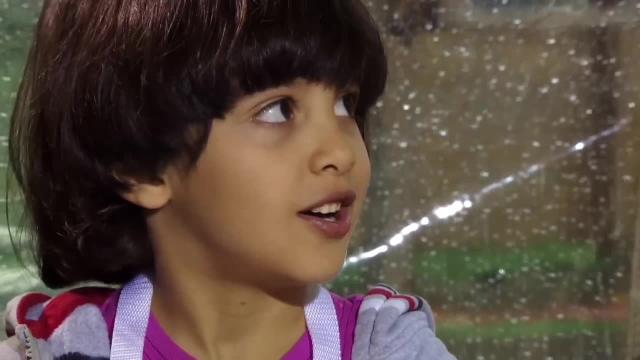 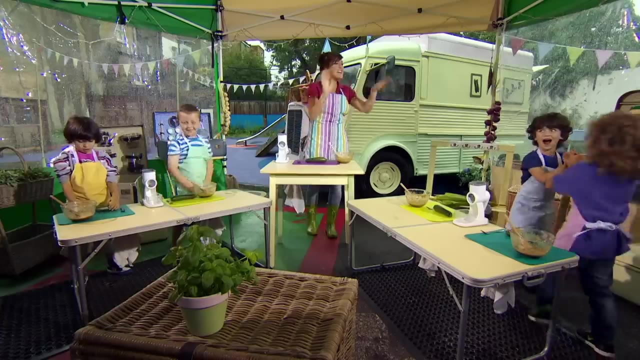 What animal goes snap, snap, snap. Crocodile, That's right. Hey, why don't we all pretend to be crocodiles? Put your arms like this and go snap, snap, snap, snap. Okay, let's snap our courgette. 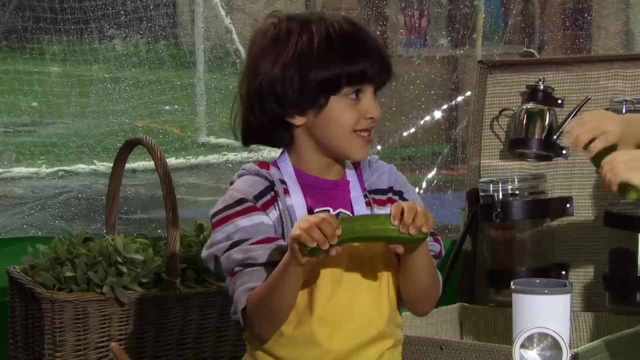 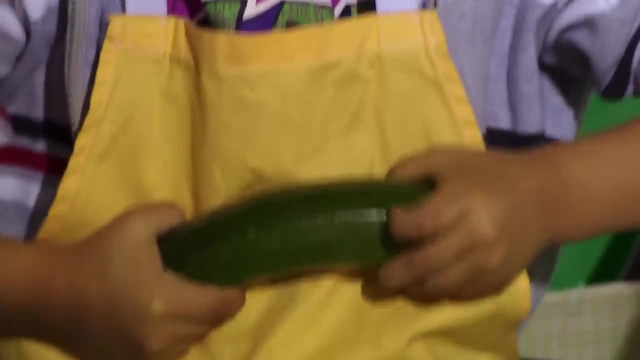 Okay, hold the courgette Out in front, Out in front of us, like this, like a pair of bicycle handlebars, And then we're going to snap it in half like this Snap, And if you put it like this, it looks like a crocodile. 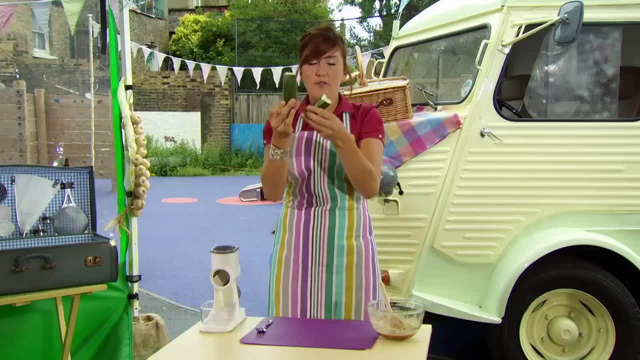 Snap, snap, snap, snap, snap, snap, snap. Now we have got to grate these bits of courgette, And to do that, we're going to use our grater and we're going to work in pairs. 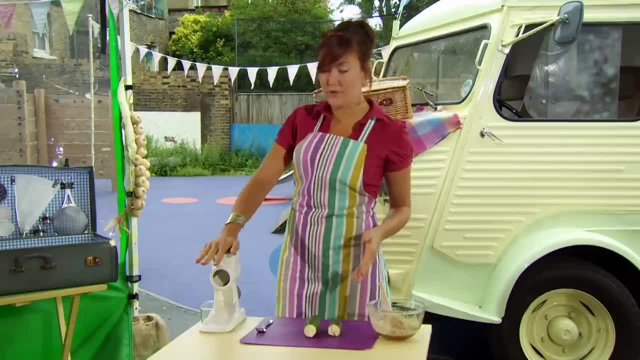 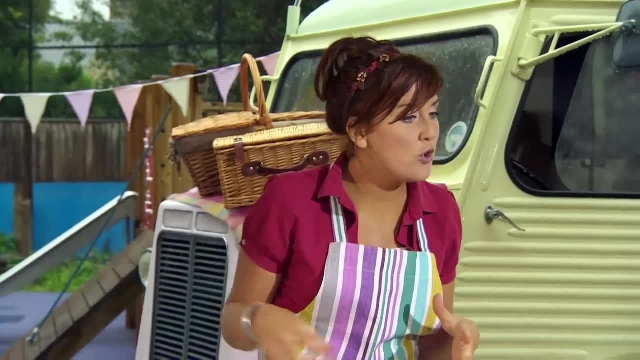 So one person is going to push the courgettes down at the top of the grater and then the other person is going to turn the handle, So you all need to put your courgette into the top of the grater. 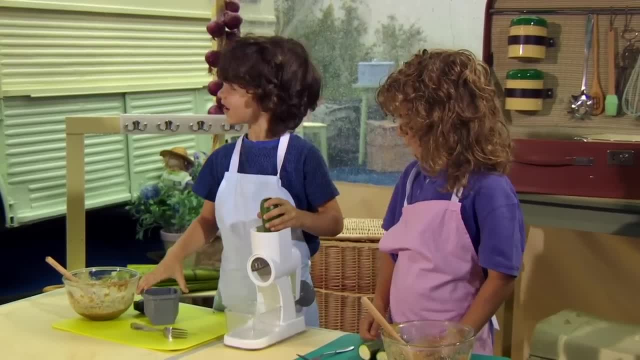 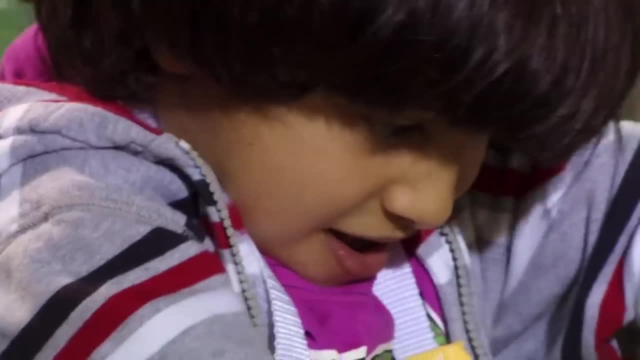 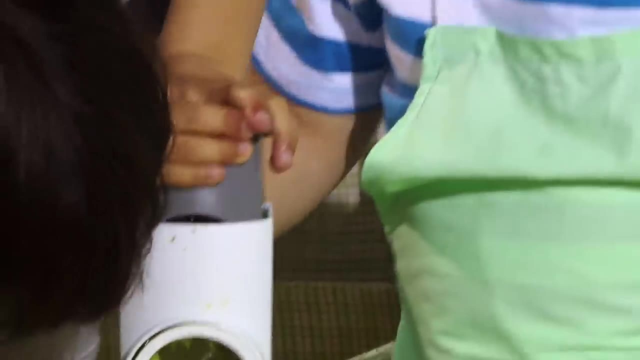 And then get that grey lid and push down on it like this And grate- Push down really hard, Nasa, You can do it. And when you've grated all the courgette, you need to use your fork to scrape out the rest. that's in the round bit. 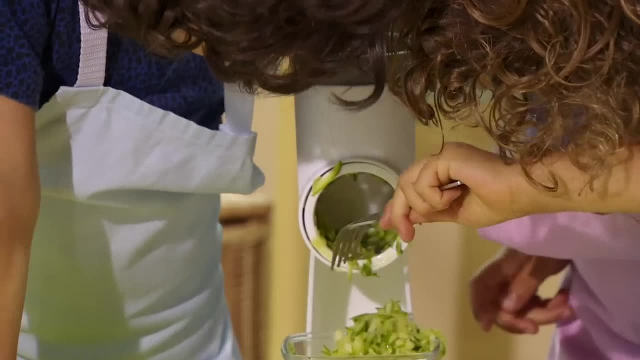 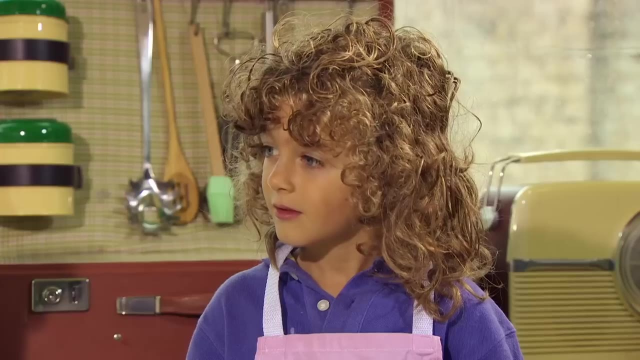 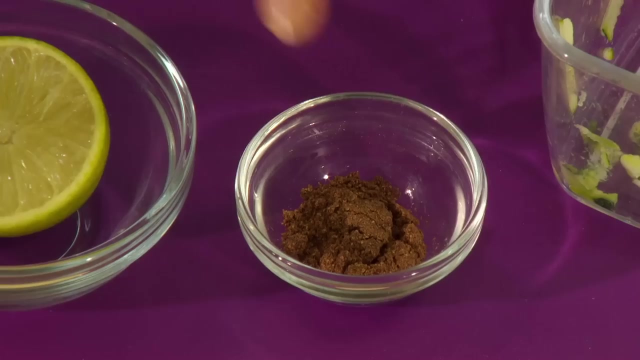 But it's very sharp in there, so really be careful with your fork. Okay, Be careful with your fingers. everybody, Everyone, finished. Yeah Right, let's add our grated courgette to our bowl, And the next ingredient is this: 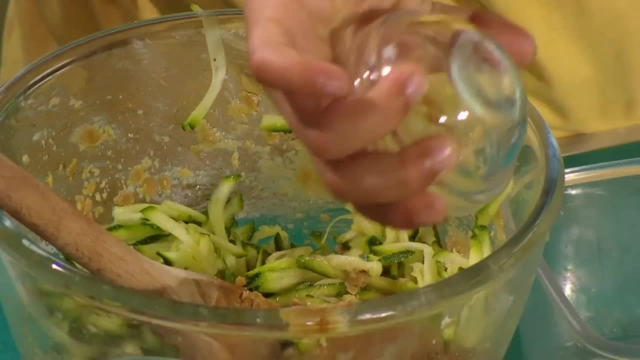 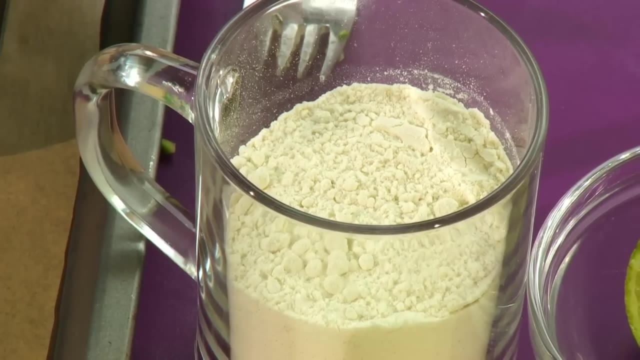 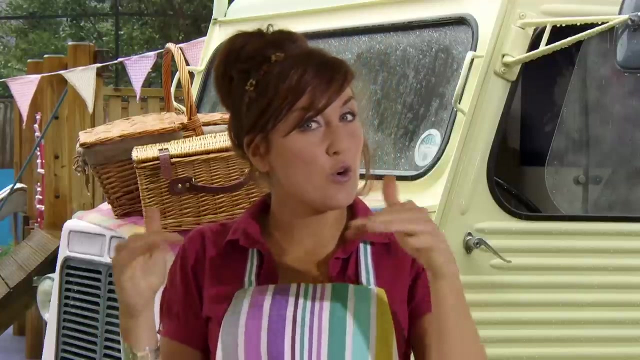 It's called mixed spice. Let's add that to our bowl, Sprinkle, sprinkle. And the next thing we're going to add is some of this: It's self-raising flour. And guess what? It's magic, Because when you add self-raising flour to your recipe, it makes everything rise up when it goes in the oven. 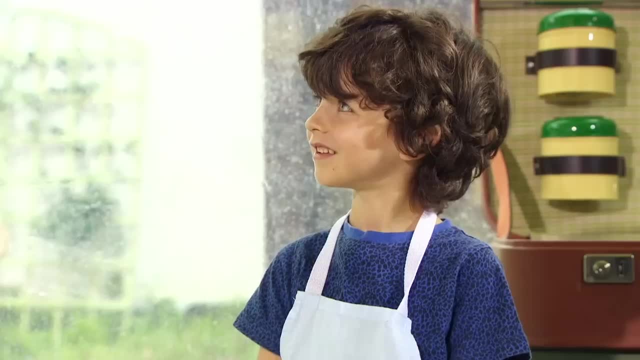 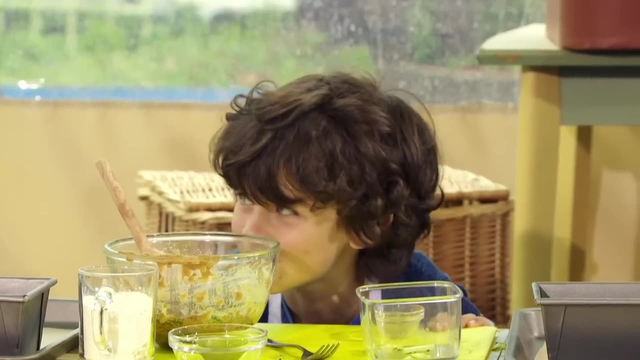 So shall we pretend to be the courgette cake rising up in the oven? Okay so we start down really small, like this. Then when we cook in the oven, we go like this: Okay so, let's add some flour to our bowl. 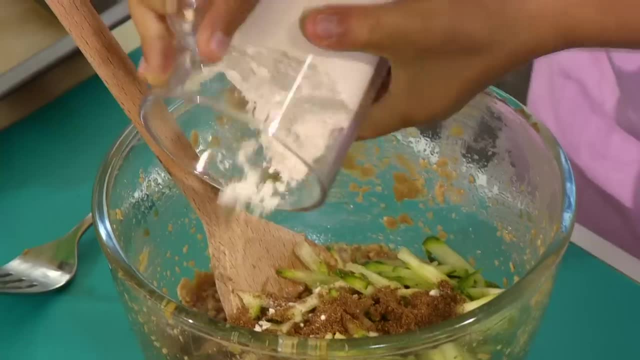 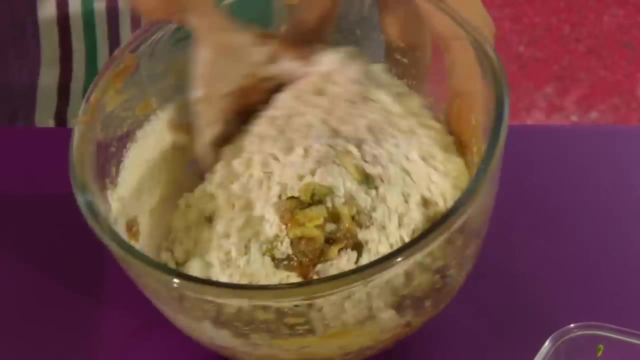 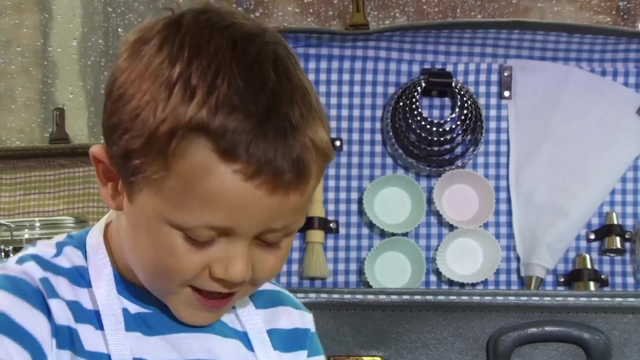 Snowstorm, Snowstorm, Snowstorm. And then we're going to mix everything up using our wooden spoon And then you've got to keep mixing it until all of that flour completely disappears. And this is hard work, I know, Paddy. 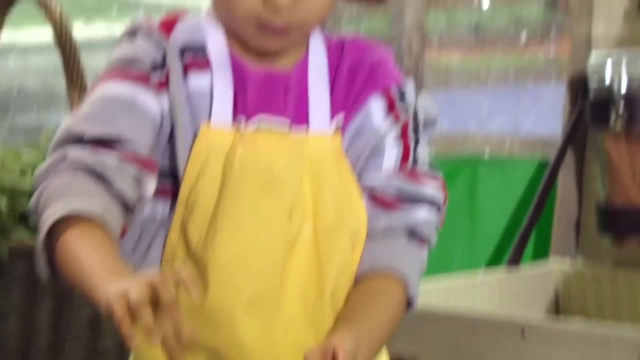 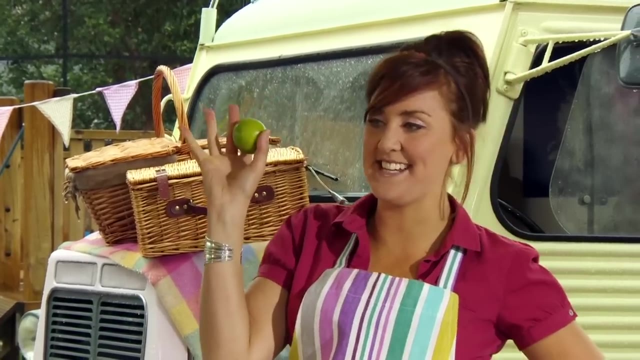 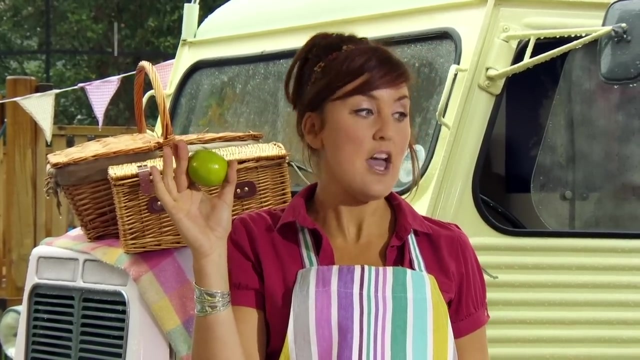 Tell me about it. My arm's aching And stop mixing. Our next ingredient we're going to use is this: What do you think? this is? Lime. That's it Lime, And limes are very, very tangy. Who wants to do a lime face Ready? 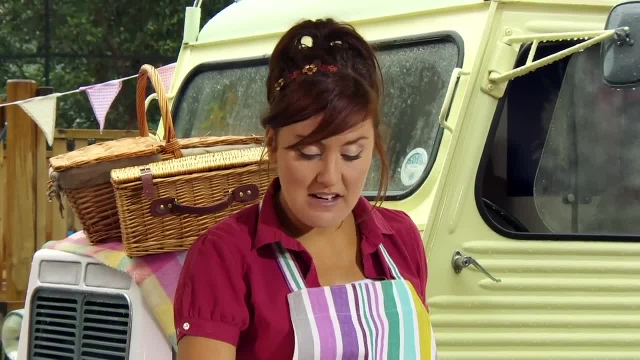 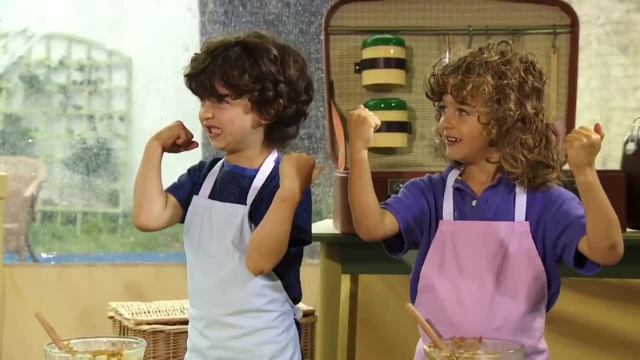 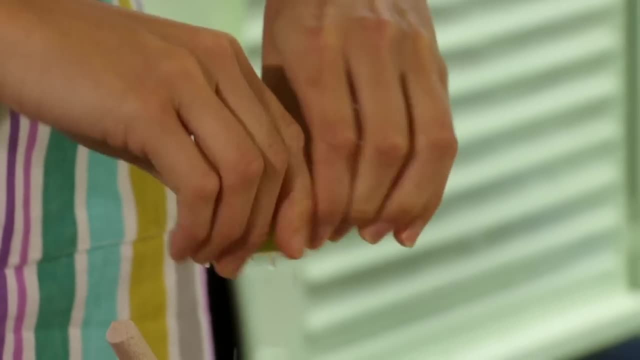 Okay, we're only going to use half a lime, but we've got to be very strong to squeeze all the lime out. So, boys, let's see your muscles. Ah, Take your lime and squeeze it into the bowl like this Squeeze. 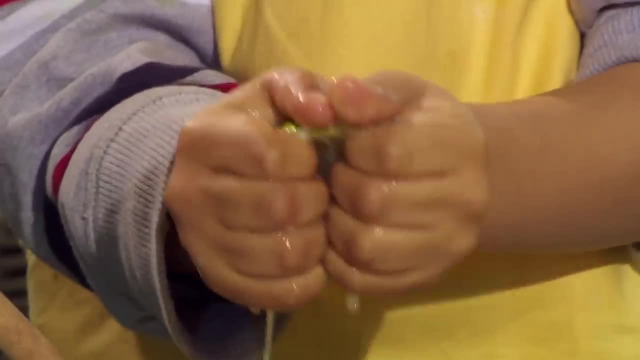 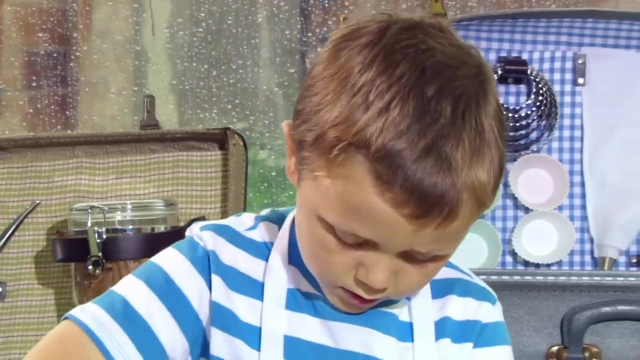 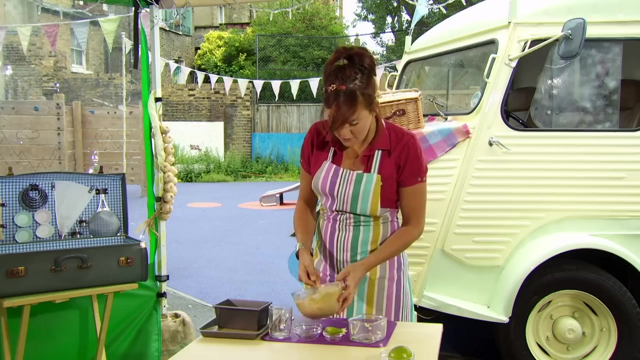 Get all the lime juice out, And then, of course, we have to mix it all up again, And finally, we're going to spoon the mixture into the loaf tin, which I've already oiled for you, And to do that, we're just going to gloop it. 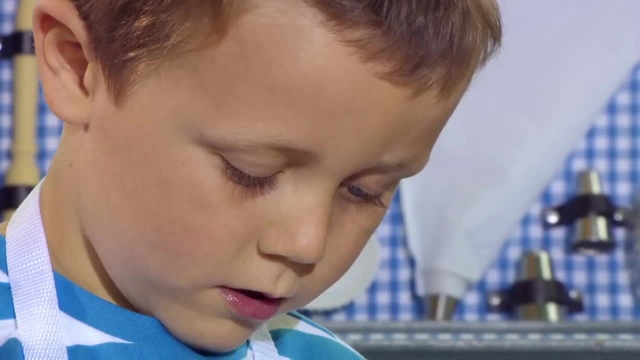 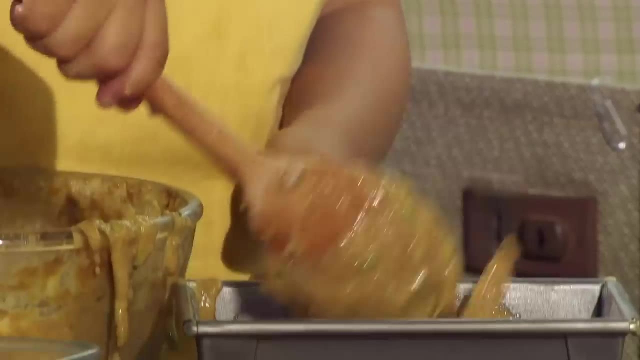 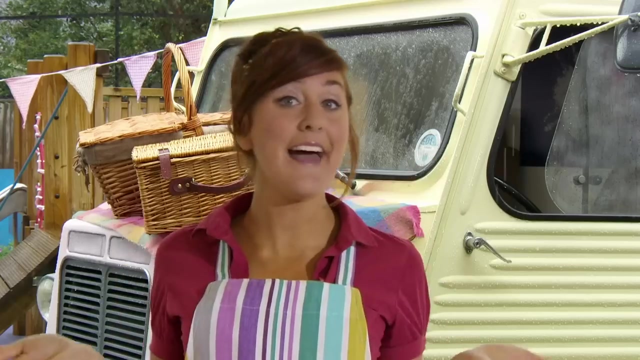 And then we're going to put it in like this: Gloop, Try and get really big mountain fulls of the mixture, That's it, And put your wooden spoon into your bowl And that is it. You have done it everyone. 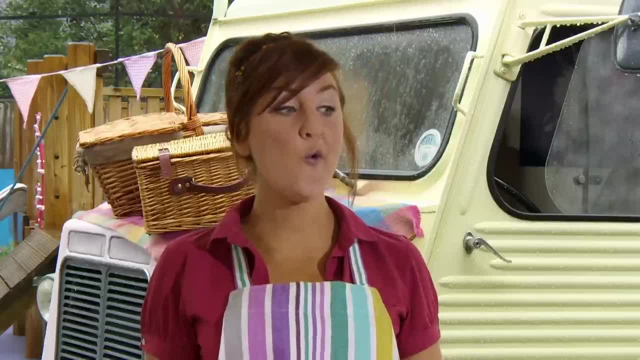 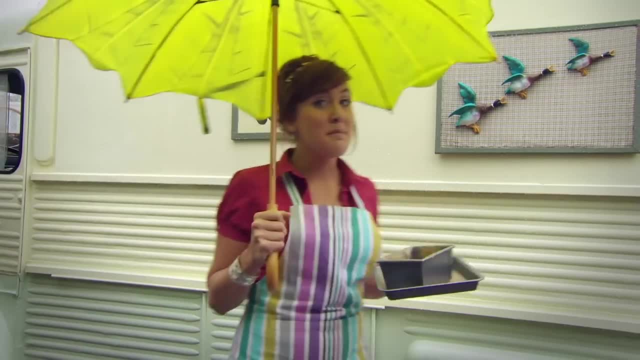 You've put all the ingredients together for Katie's courgette cake all by yourself, And now it's time to put them in the oven to cook. But remember ovens are hot, so don't go near. Ask a grown-up to help you here. 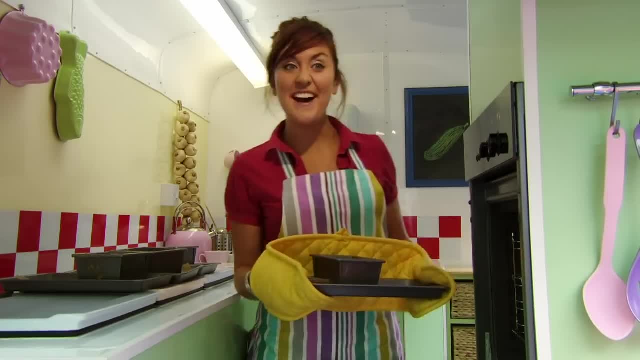 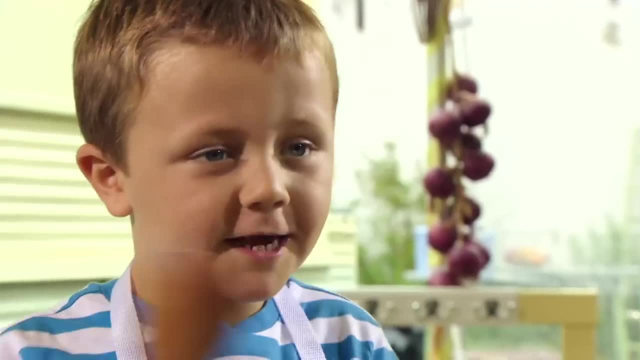 Now we've cooked with you and had lots of fun. Let's tidy up and think of all the things that we have done. There was Cracking, Breaking, Squeezing, Mixing, Clearing any mess and putting things away. 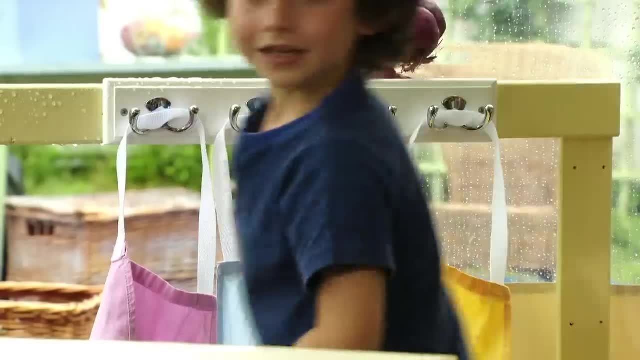 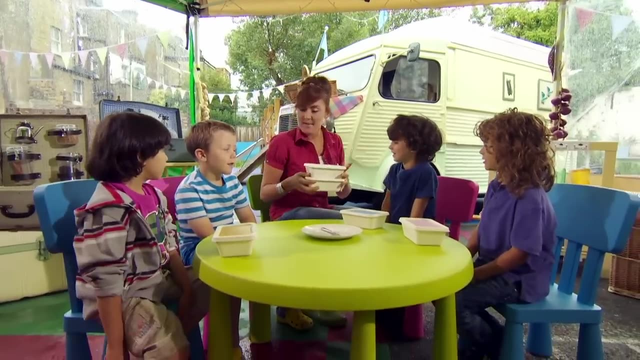 It's always fun to do at the end of the day. And here are the courgette cakes boys. They've all cooked. They smell absolutely amazing. Shall we have a look at what they look like? Yes, Okay, let's have a look at Cosmo's. 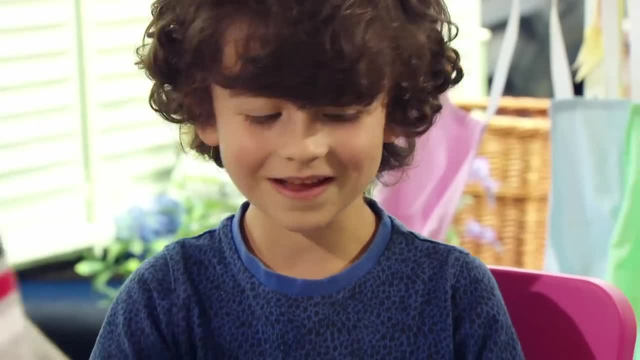 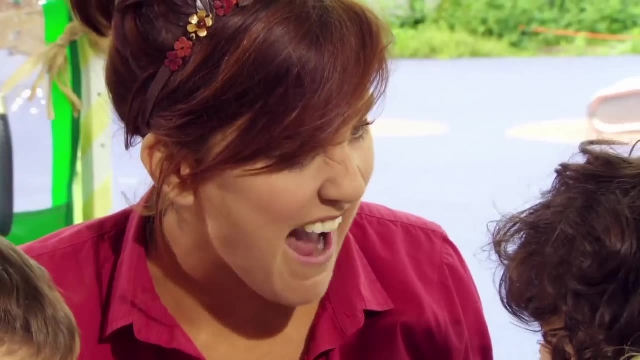 Open up Cosmo. Ooh, What's happened to yours? It's soft, Look, It's soft. And what's this bit here? Crack A big crack. Yeah, So, because it was rising too much. then it got a crack in the middle. 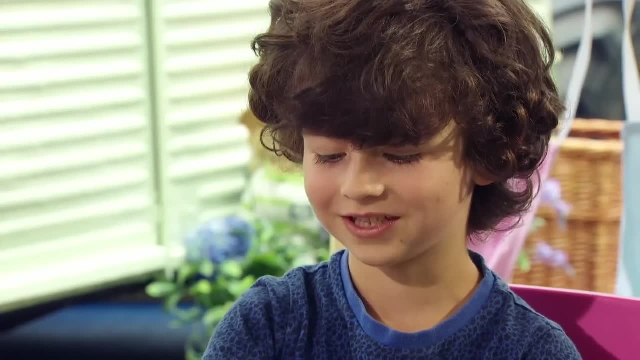 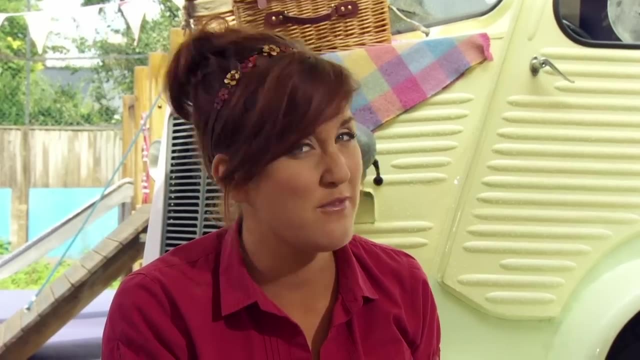 Do you remember what made it rise up? The self-raising flour. You've got it. Okay, everyone, let's put the lids on top and we'll save it for later. We've travelled to you, We've cooked and had fun. 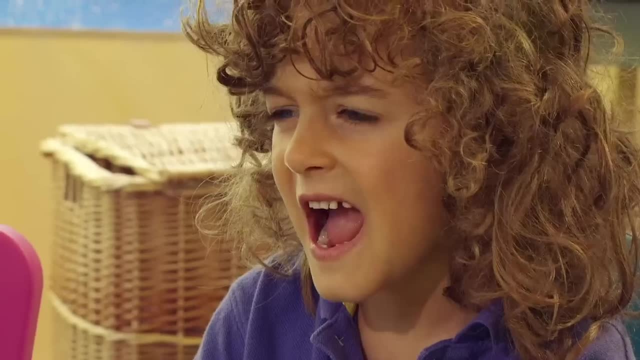 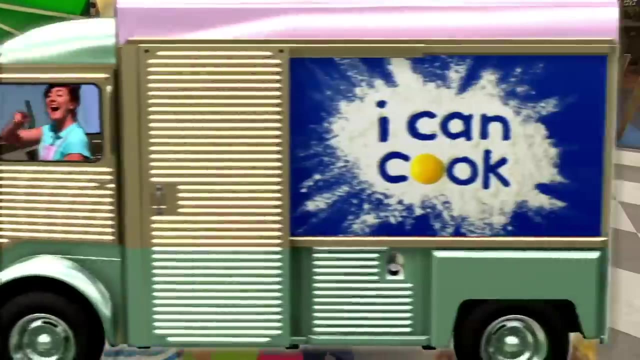 Now let's have a party with everyone. Yay, Come on, boys, let's go, And you can come with us. Look, there's everyone waiting for us. Shall we go and share our food? Yeah, Come on, let's go. 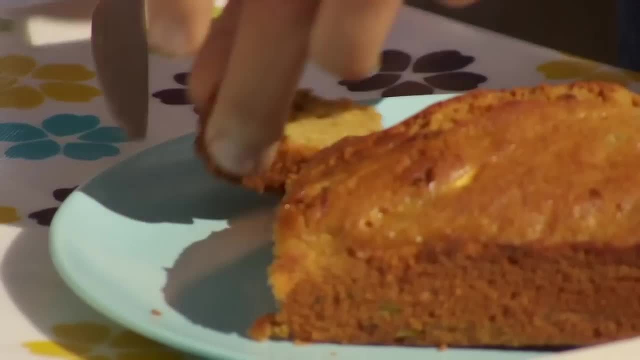 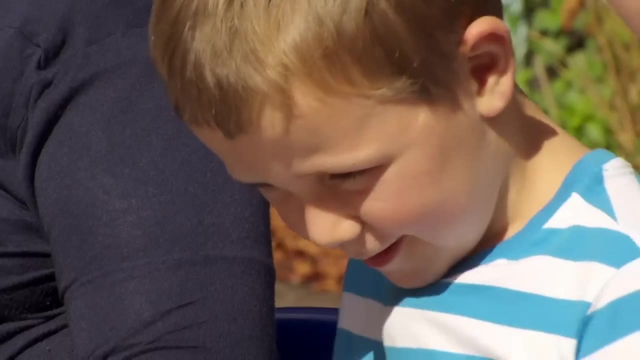 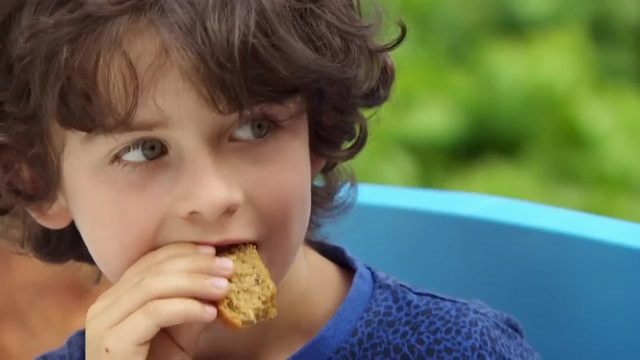 Yeah, Yeah, Mmm, Mmm, Yummy Pads. What was your best part? Cracking the egg? Oh wow, Mmm. Oh, it smells gorgeous, Is it yummy? Shall I try some Mmm. 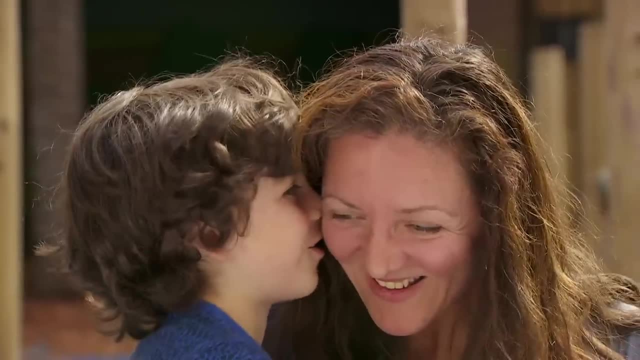 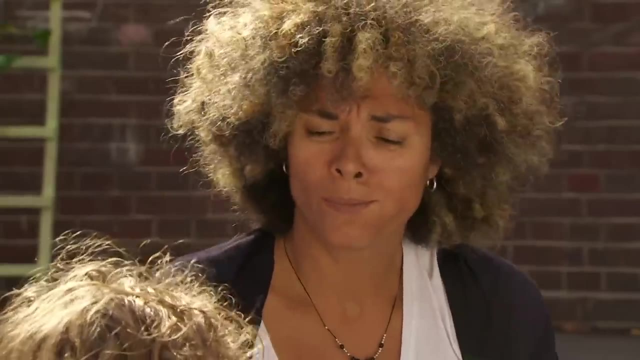 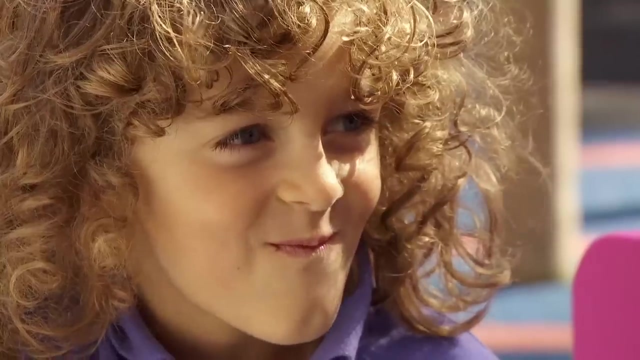 This is really yummy. Okay, We'll make it at home. yeah, Mmm, Mmm, It's delicious. And did you make this all by yourself? That's amazing, Taya. Congratulations, Paddy. we've used courgettes in this cake, but what other vegetables do you think we? 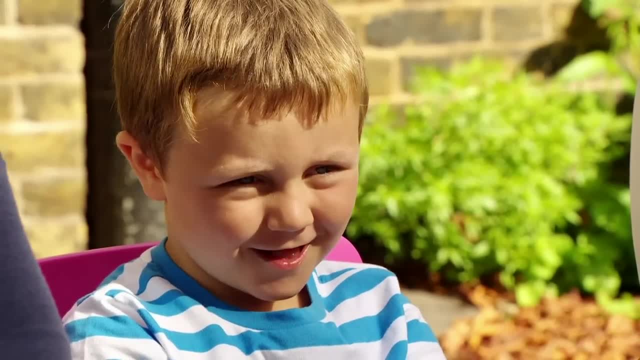 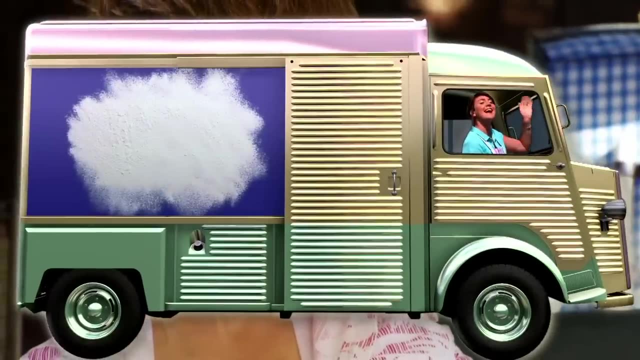 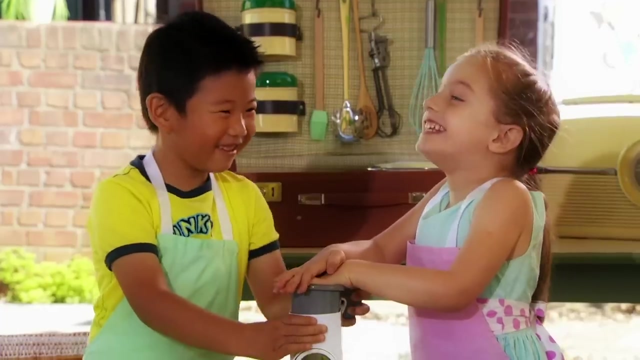 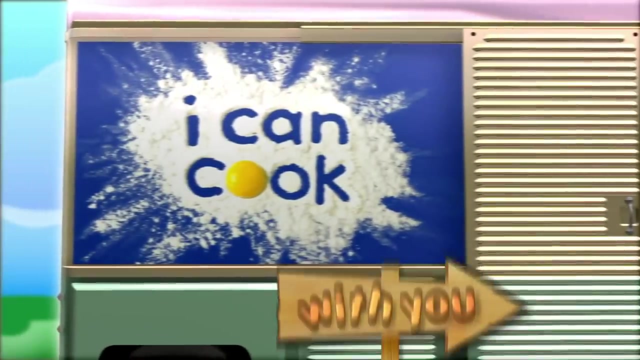 could use if we made it again. Um, carrot, Mmm, Definitely carrot. So what can you do? I can cook, I can cook. You could have cooked it in the oven. You could have cooked it with a little bit of salt and sugar. 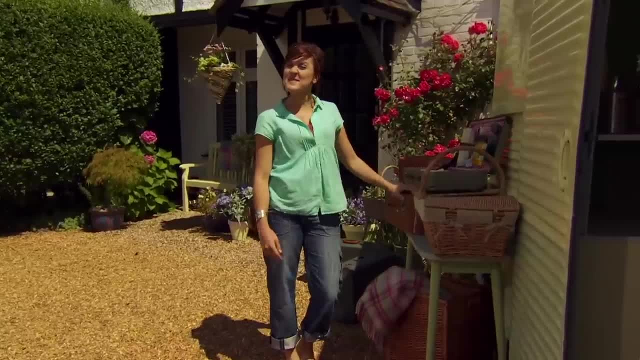 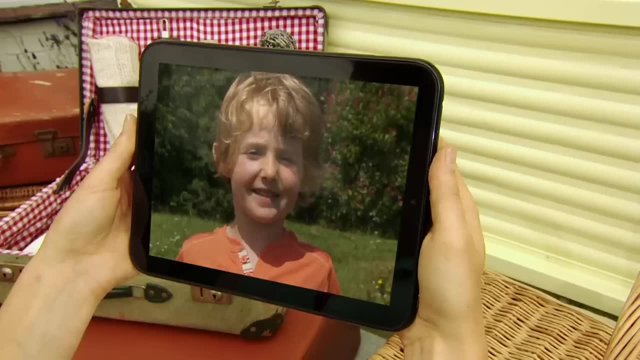 I can do everything. Don't worry, I'll do the work. Oh wow, Are there any carrots in the oven? I'm sure they are, Kate, I'd like some. Do you like carrots? No, Katie, can you cook with me please? 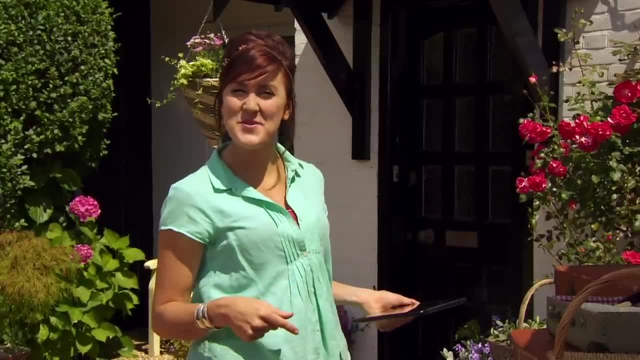 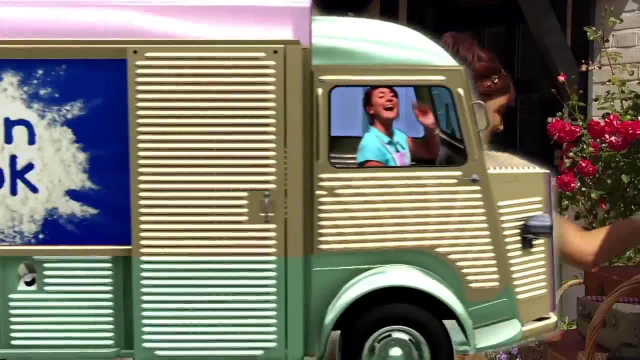 I can, and you can cook with me too. Oh, I do love fudge. That's really exciting. Come on, then, let's pack everything up and we'll be on our way Off on a journey, and I'm coming to you. 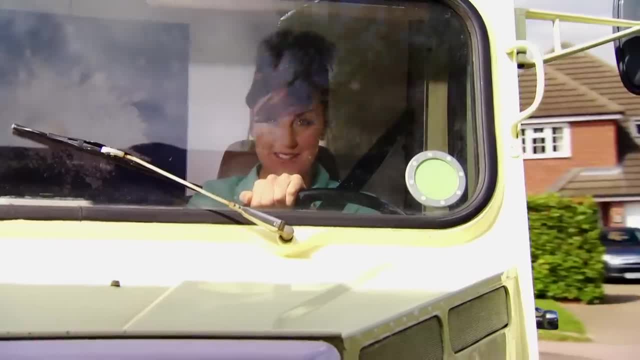 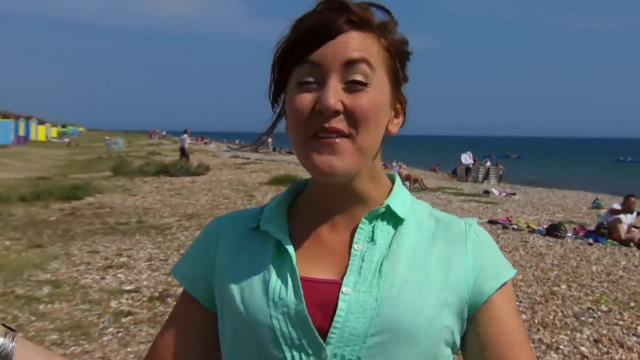 It's going to be busy and there's lots to do. Get ready to help, join in and have fun. Let's cook a feast for everyone. Well, here we are at the beach and it is a beautiful day, But I don't know where Owen is. who invited me here? 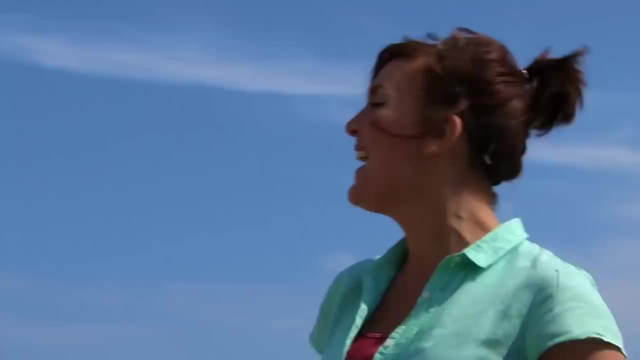 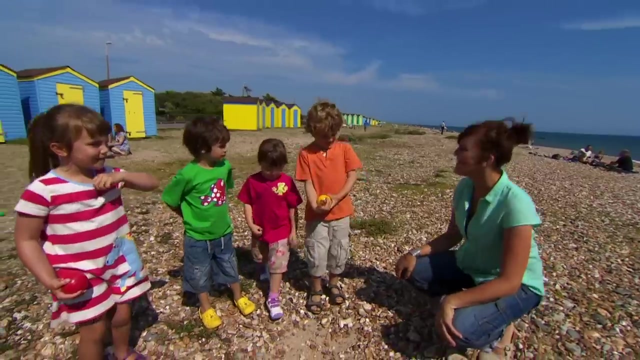 Where, Oh, he's over there with his friends playing a game. Hi Owen, Hi, Katie Owen, are these all of your friends? Yes, And what's your name? Lexi? Hello, Lexi, And what's your name? 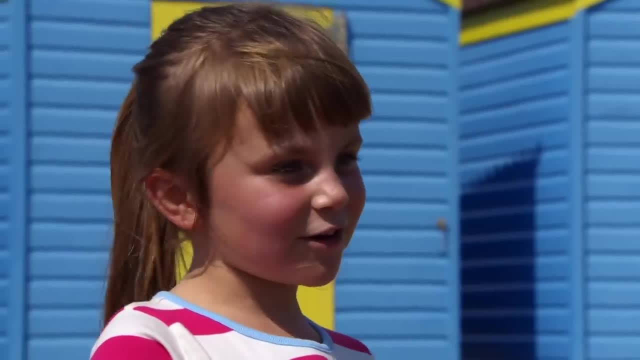 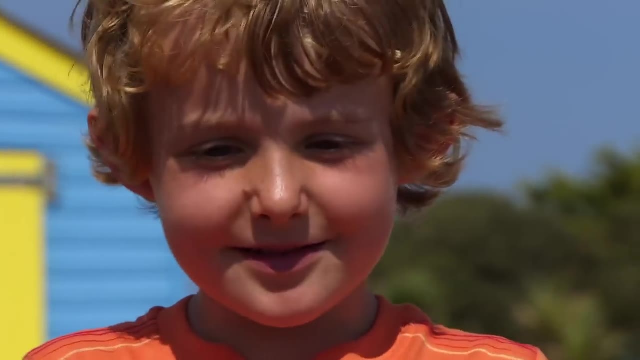 Toby- Hey, Toby, And what's your name? Avery, It's so fantastic to meet all of you. Now, Owen, Are we actually going to go kayaking? Yeah, And we're going to have a picnic too. I have got such a delicious recipe that we could cook together. 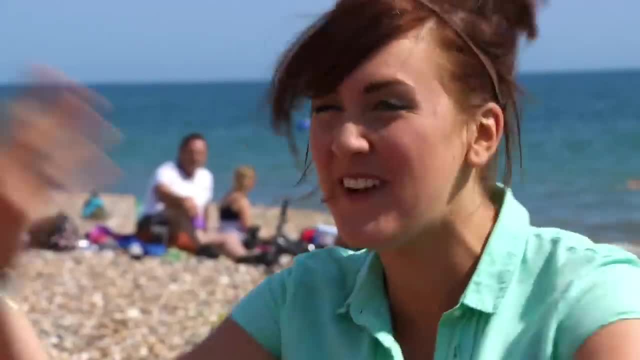 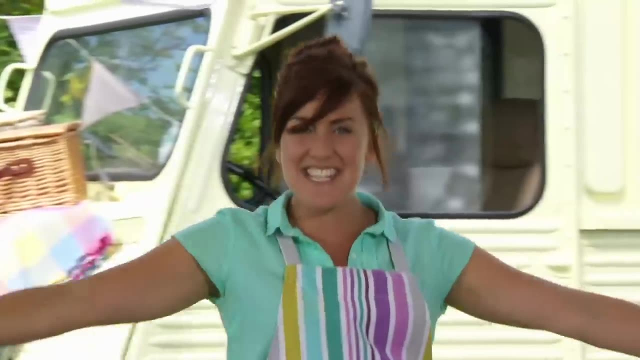 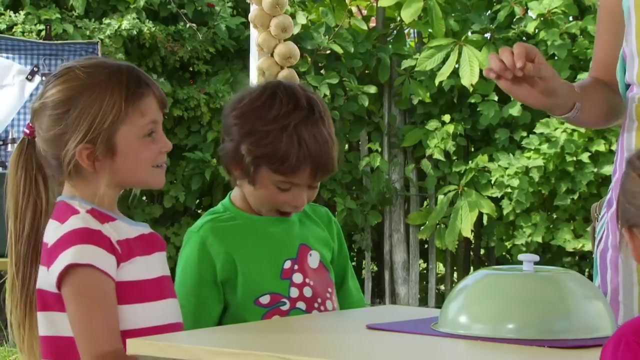 Do you want to make it? Yeah, Oh, brilliant. Come on, follow me, I'll show you. Welcome to my outdoor kitchen. everybody Who's excited Me. Are you ready to do some cooking? Yeah Well, I'll tell you what today's recipe is. 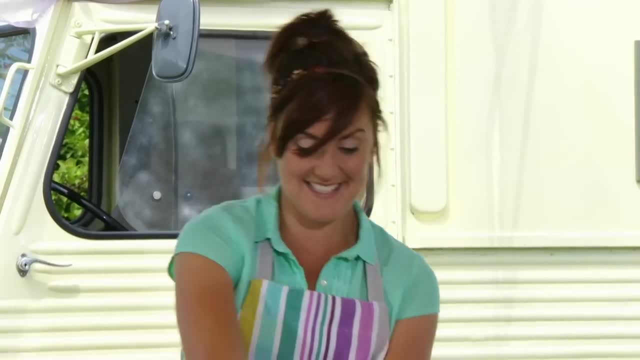 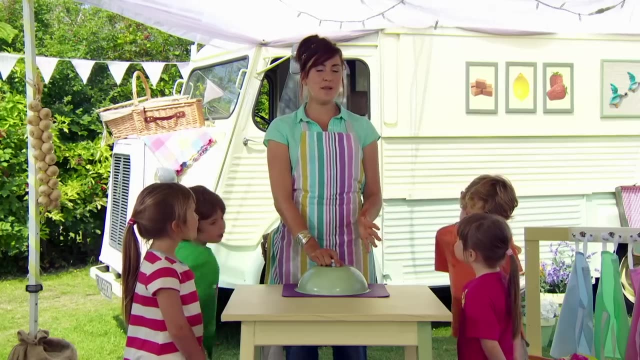 It is fig and fudge biscuit. Fudge biscuits- Ooh, They look good. But before we get started on the cooking, we've got to do something really important. Do you know what it is? Wash your hands, That's it. 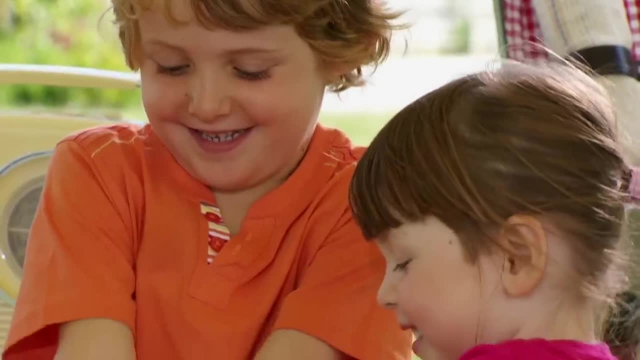 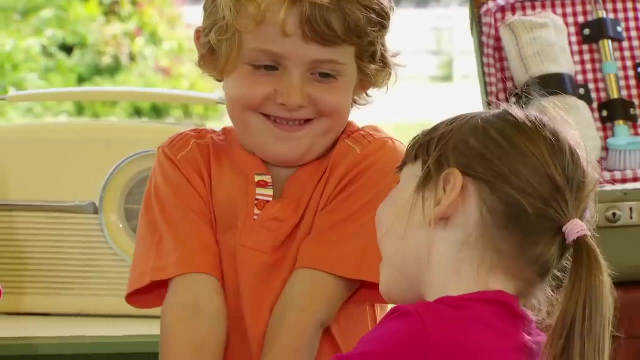 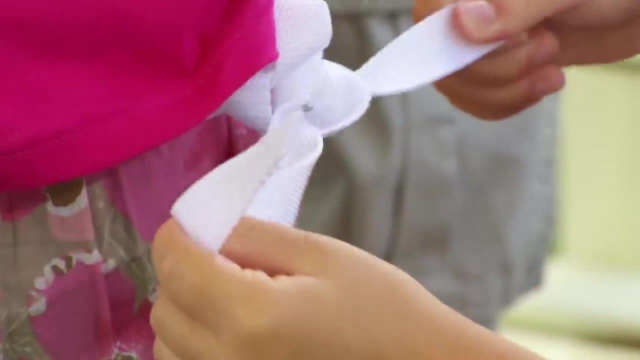 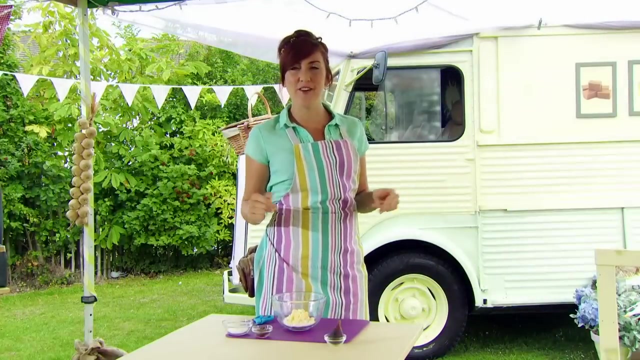 Let's get going, team. Roll up your sleeves, Give your hands a wash with slippy, dippy soap. Splish, splash, blush. Have you done your hands washed and dried? Sleeves rolled up, rolled up apron time. what can you do? I can cook. well, let's get started on our. 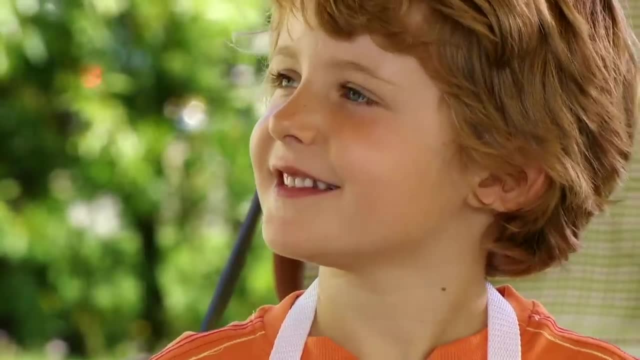 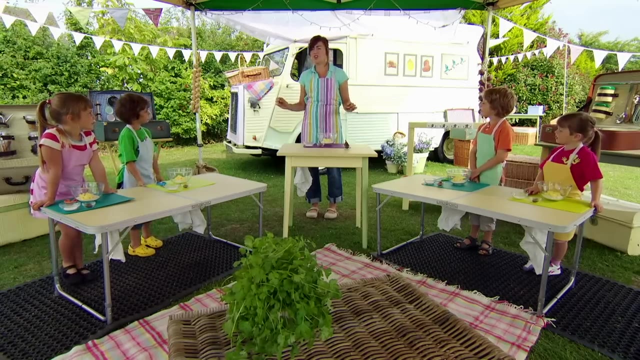 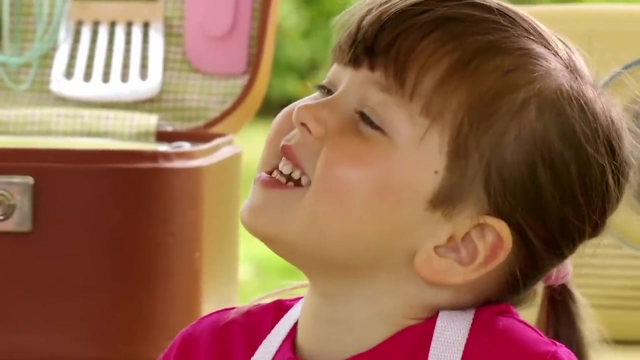 fig and fudge biscuits. that's quite hard to say, isn't it? fig and fudge, can you say that? but can you say fig and fudge quite quickly, like this: fig and fudge, fig and fudge, fig and fudge. go on then. fig and fudge. oh, that was. 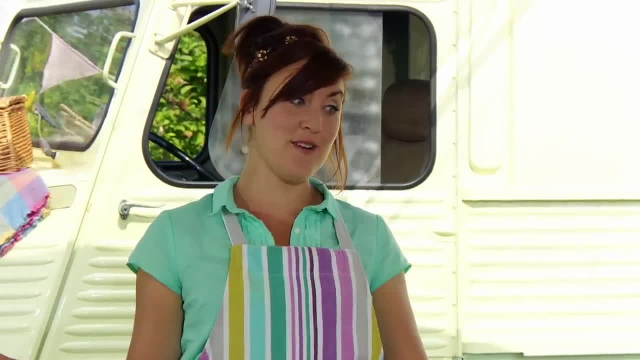 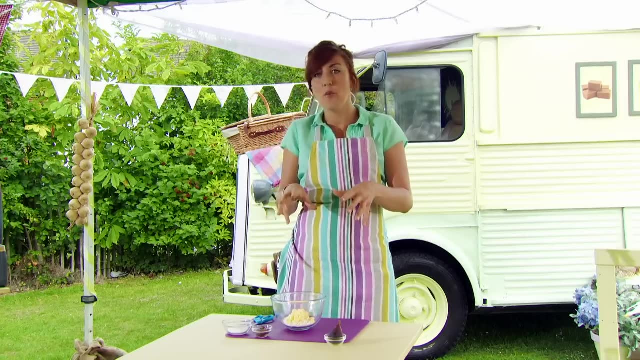 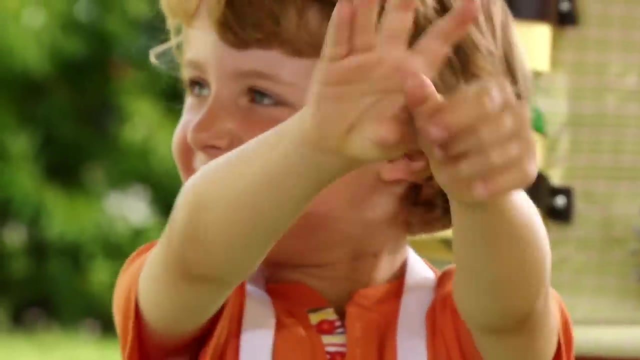 really good. now the first thing we're going to do- and I know that you, like it- is tickling, so do I. now, to tickle, we need to get out our tickle fingers. so put your fingers in front of you and go tickle, tickle, tickle, tickle, tickle. 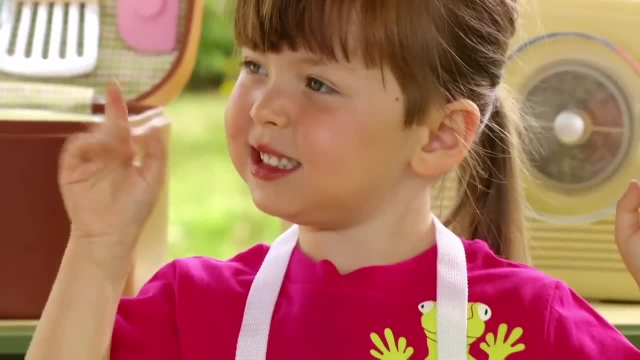 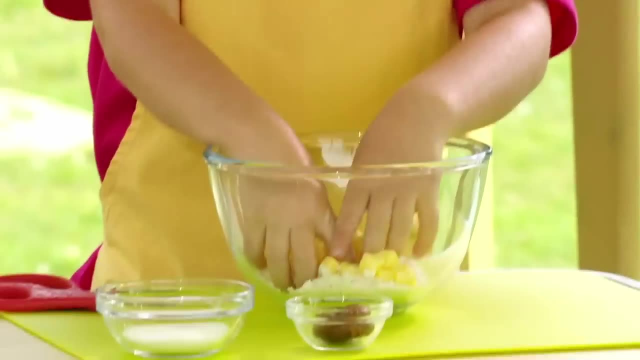 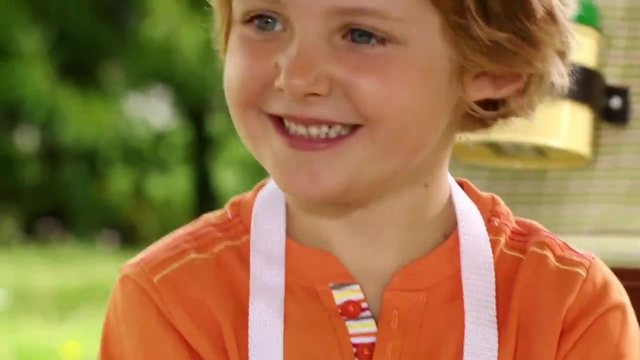 fantastic. okay, get your tickly fingers out fingers. get them tickling and we're going to dive our tickly fingers into this bowl with butter and flour- Ready, That's it- and get right down to the bottom. So dig down deep. Can you feel the bottom of the bowl? Yeah, Now I want you to squeeze everything. 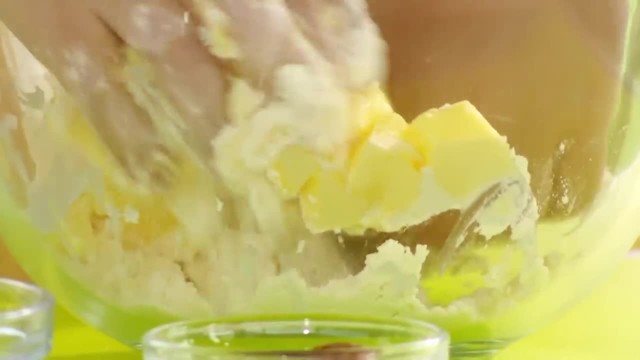 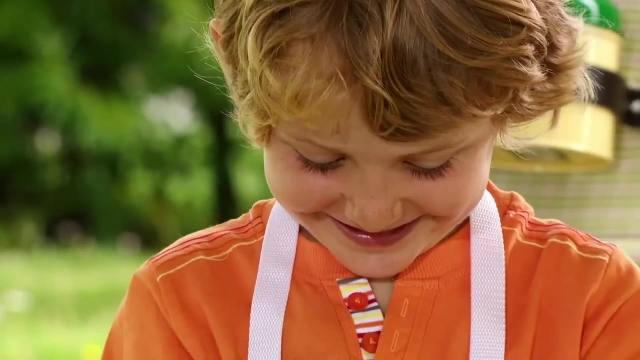 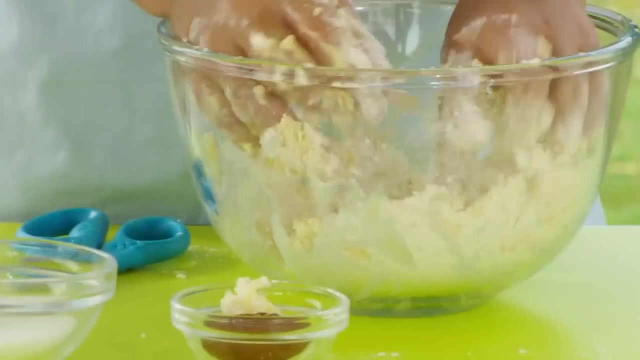 with your fingers as tightly as you can, Go, squeeze, And then we need to keep squeezing and keep tickling until everything is mixed together. Everyone go, tickle, tickle, tickle, Tickle, tickle, tickle. Don't forget to tickle with us at home. Have you got your tickle? 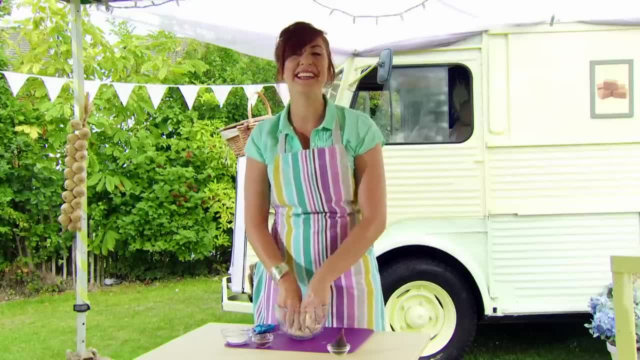 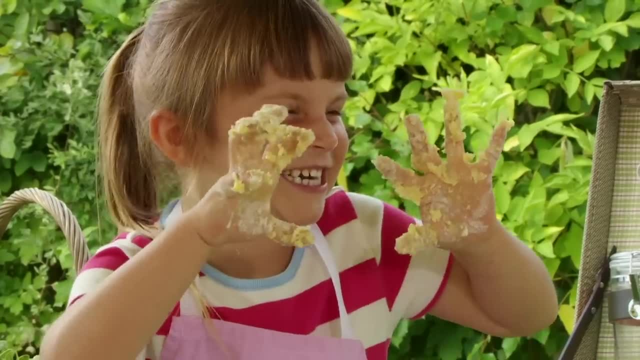 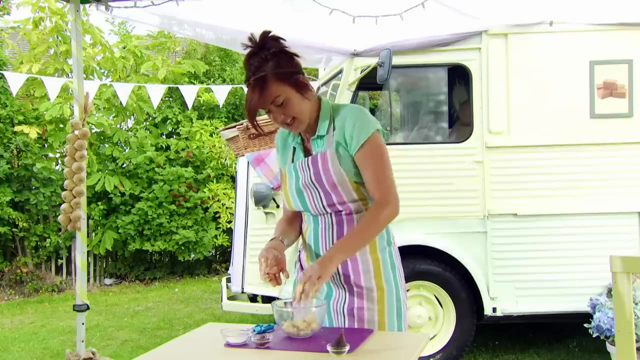 fingers, That's it, and tickle away. I'm a big monster Ready, There we go. That's just in the middle. Enough tickling. Next ingredient we need is a fig, because we couldn't have fig and fudge. 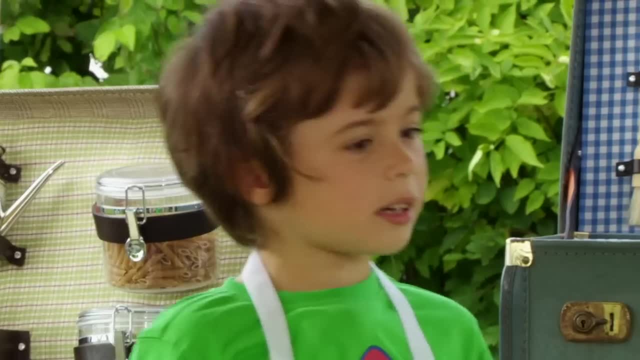 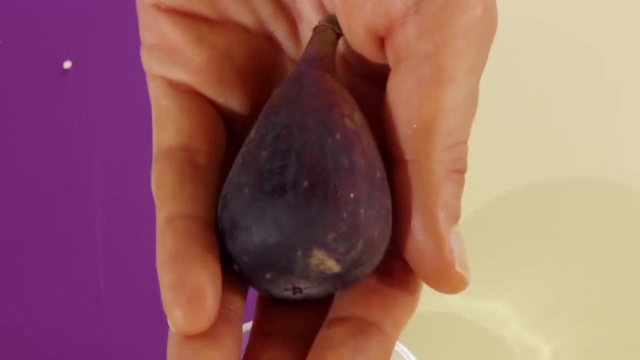 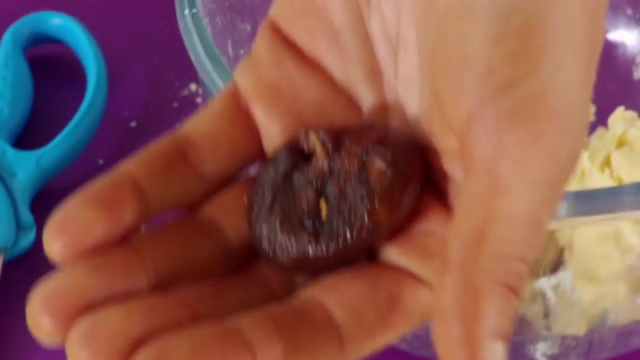 biscuits without a fig? could we No, because then it would just be fudge biscuits. That's right, it would just be fudge biscuits. Now, a fresh fig looks like this. It's really yummy. The fig can be dried, and a dried fig looks like this. It looks like it's been out in. 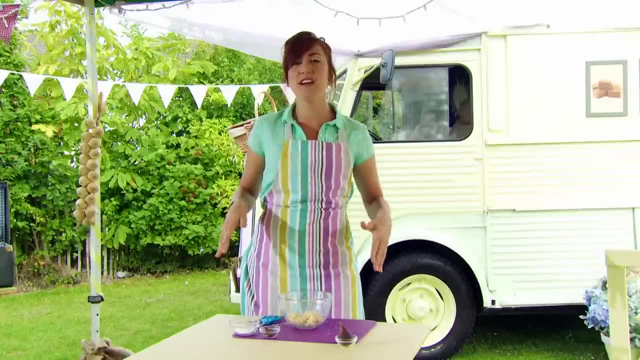 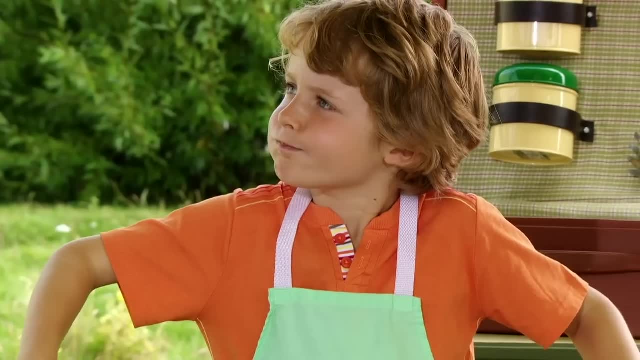 the sun for too long and it's gone all wrinkly. Can you pretend to be a fresh fig turning into a dried fig? Hey, why don't we do that? Yeah, Why don't we do it all together? So let's be a fresh fig and then we dry up in the 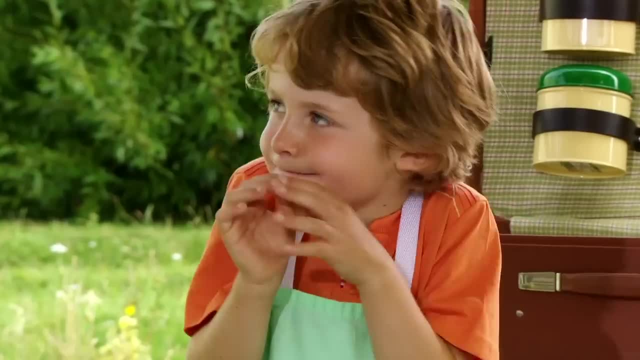 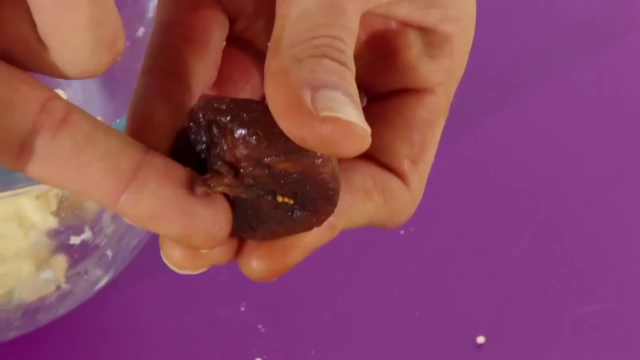 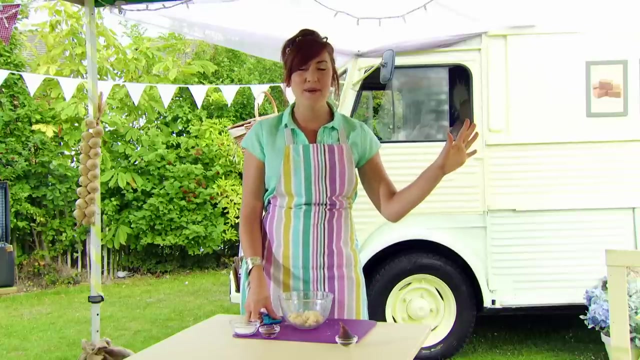 sun like this. You're like a little bunny rabbit. We need to snip the stalk off our fig and to do that we need to use our scissors. But remember, be safe with scissors. Everybody knows that you point them down towards your 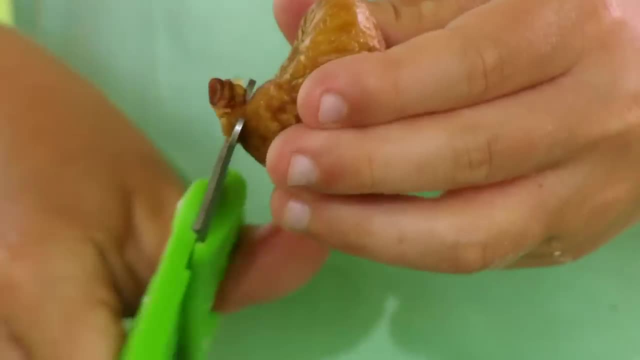 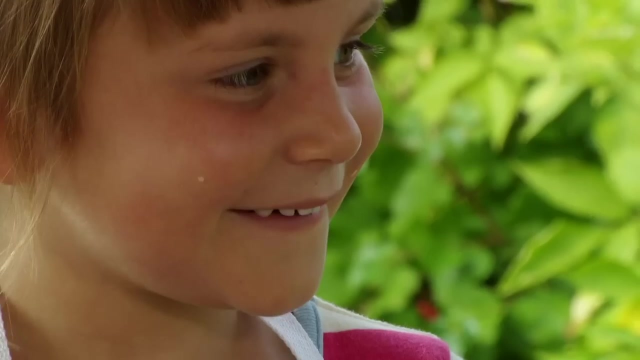 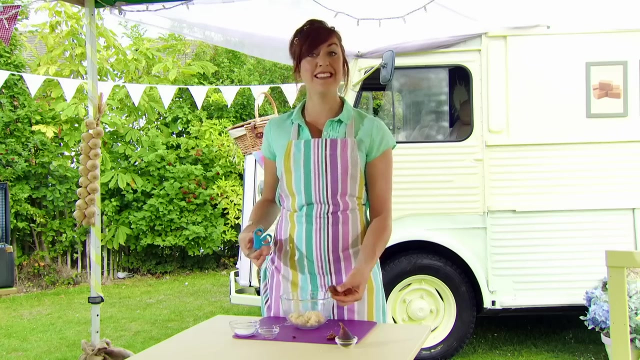 Tide, You've got it, team, So let's snip off the stalk. Snip Next. we're going to rip this fig in half. Rip, I don't miss it. Then we just need to snip these two bits with our scissors into small pieces. So let's get. 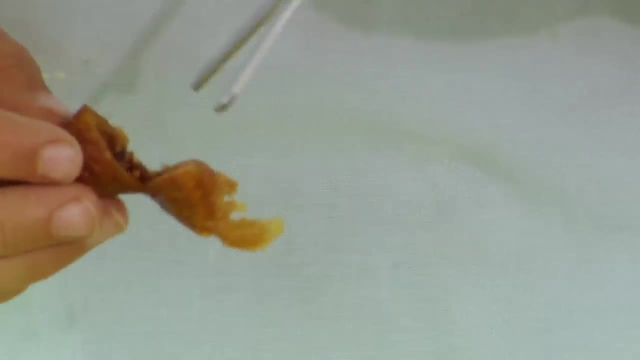 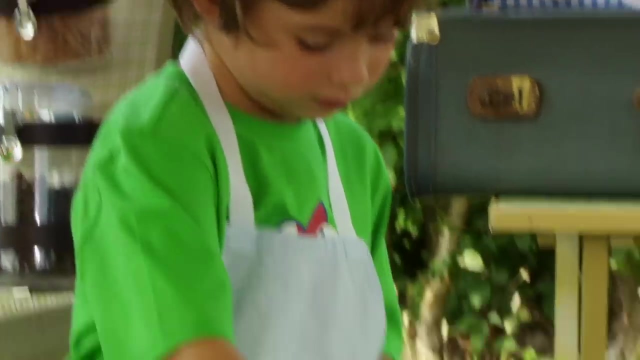 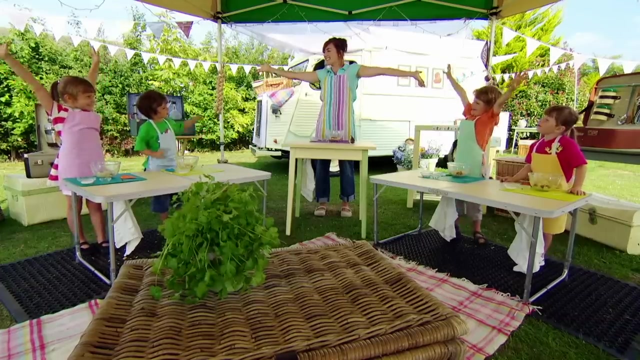 snipping. There we go, And then put your scissors down once you've finished snipping. OK, now sprinkle the fig into the bowl. Ready Woo-hoo. Who likes sweet figs? Me, Me, Oh, I love them, which is why we're going to add some sugar to our recipe. So watch. 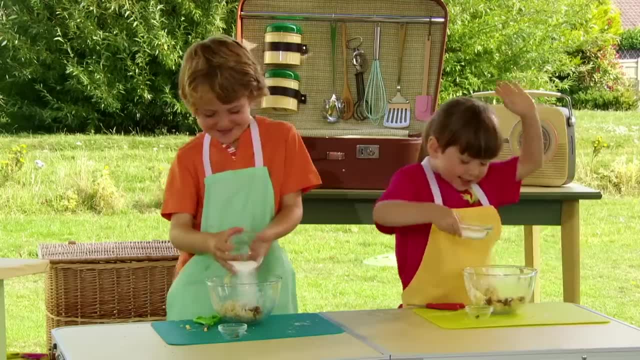 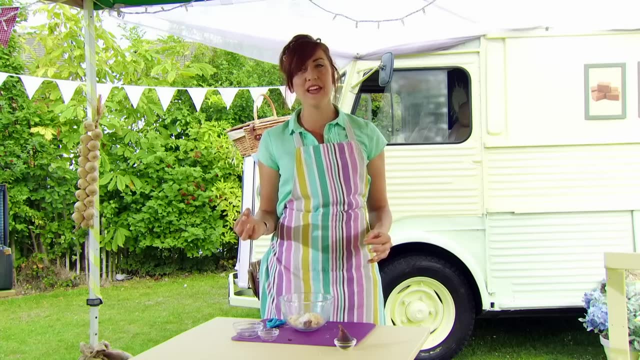 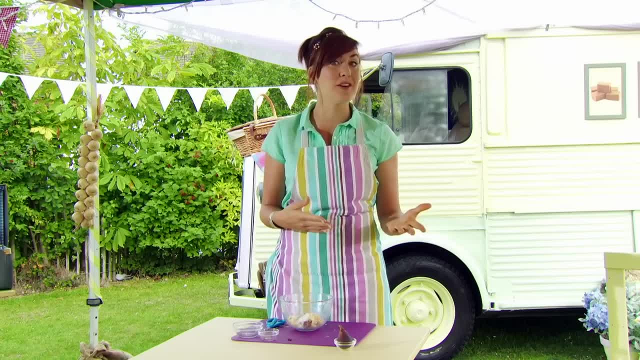 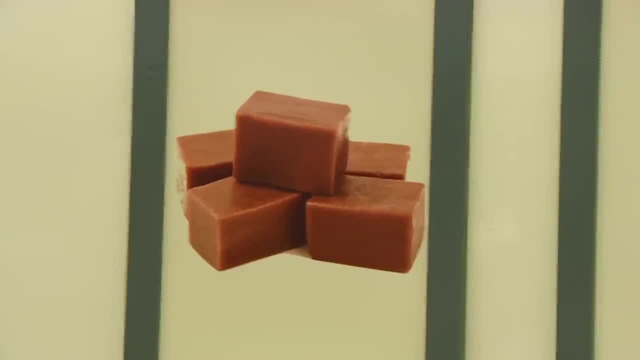 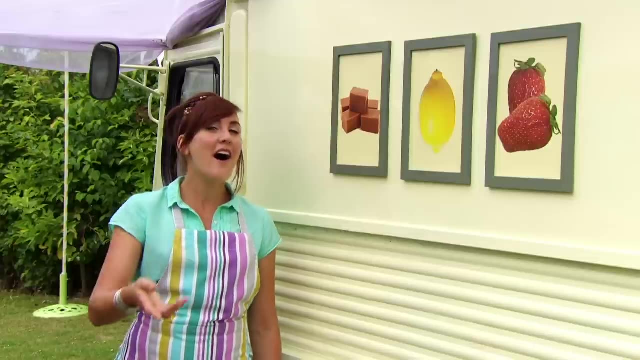 What's next? Well, let us see if you can guess what it could be. What would you choose for our fig and fudge biscuits? We've got some fudge, a lemon and some strawberries. I know I'll give you some clues, and then 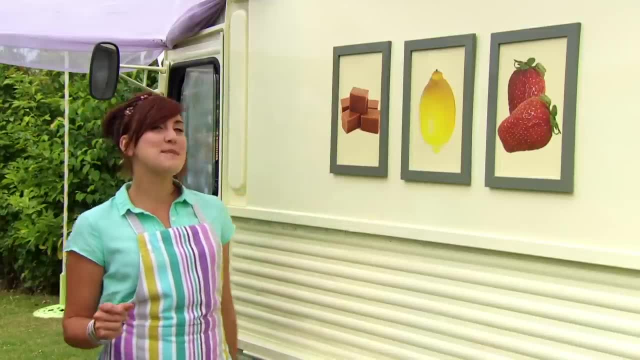 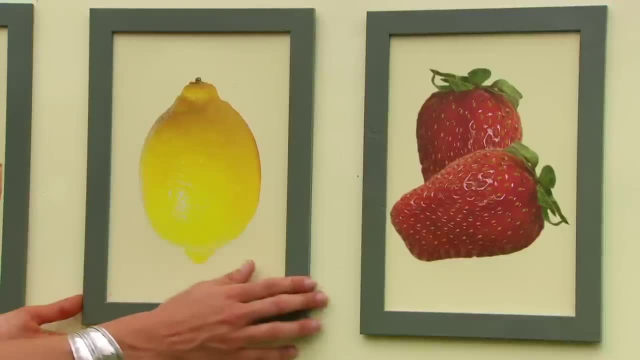 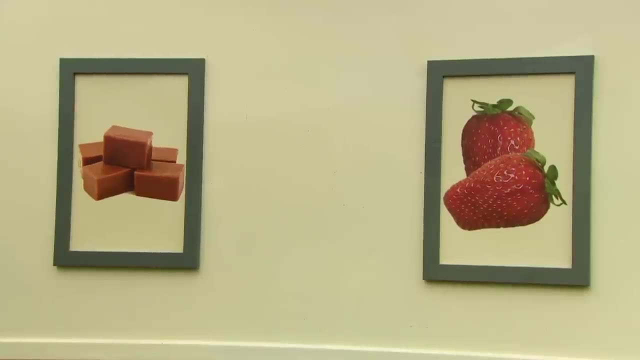 you can try and guess what it might be OK, here's one. The special ingredient is sweet. Well, lemons are really sour, aren't they? So we can definitely take lemons away. OK, here's another clue. The special ingredient is sweet and it's not a fruit. Well, strawberries. 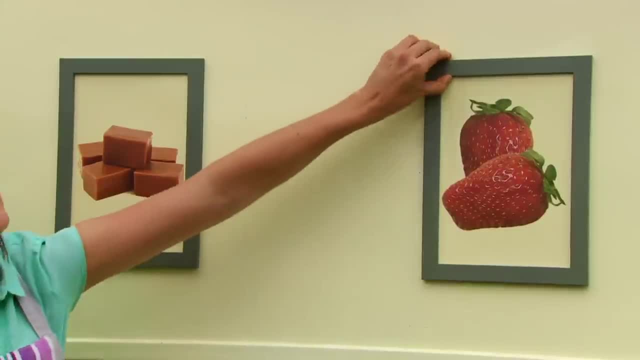 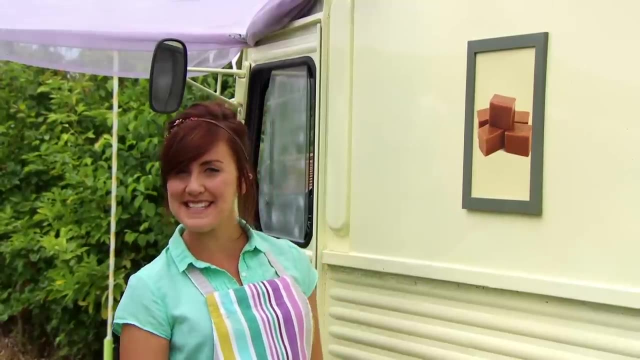 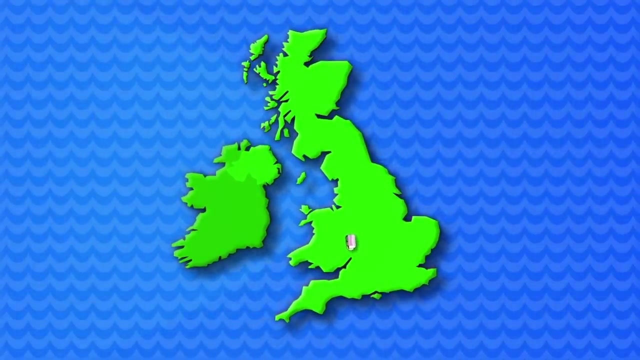 are definitely a fruit, aren't they? So let's take that one away too. There we go, Which leaves us with fudge. We're going to need some fudge for our fig and fudge biscuits, and I went to make some. 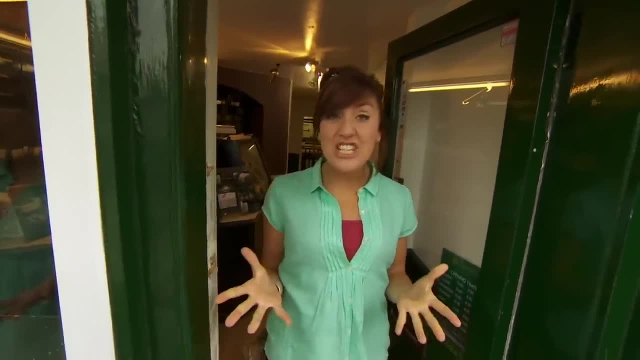 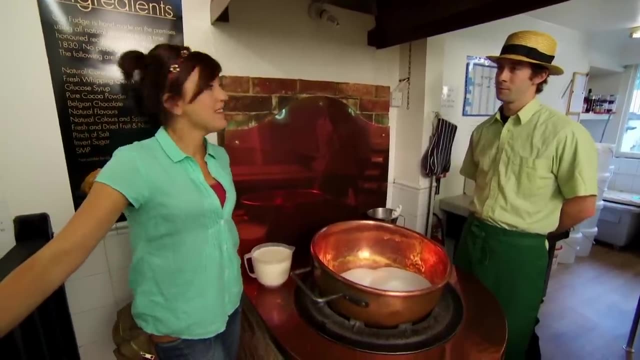 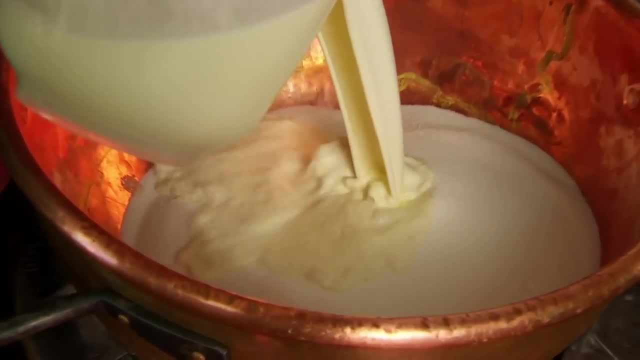 I've come to a shop in Windsor to find out how fudge is made, So let's go inside and have a look. Come on, OK, This is my friend, Patch, who's going to help me. Hello, Patch. Hiya, Fudge, Katie, is made of sugar and cream. They melt together to give fudge its 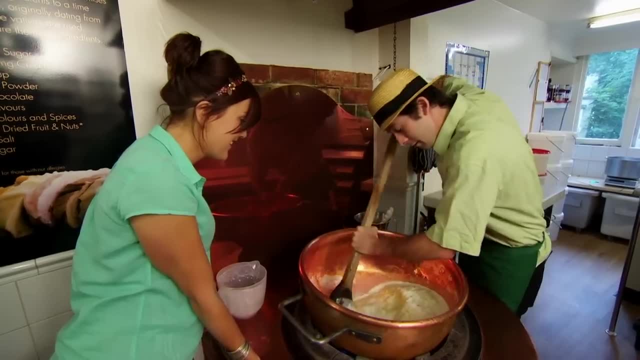 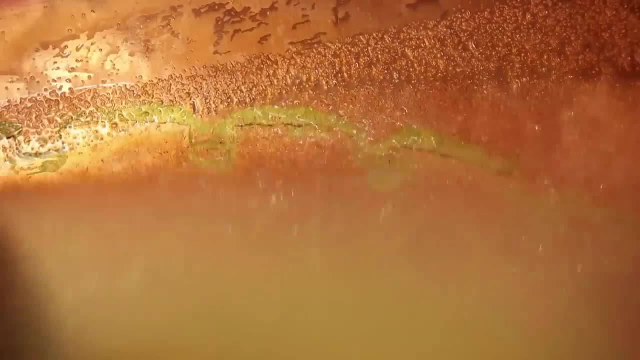 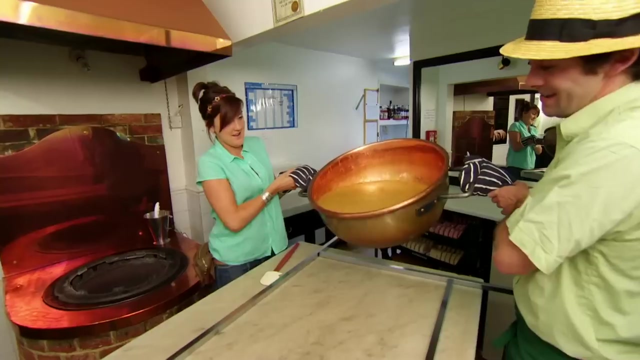 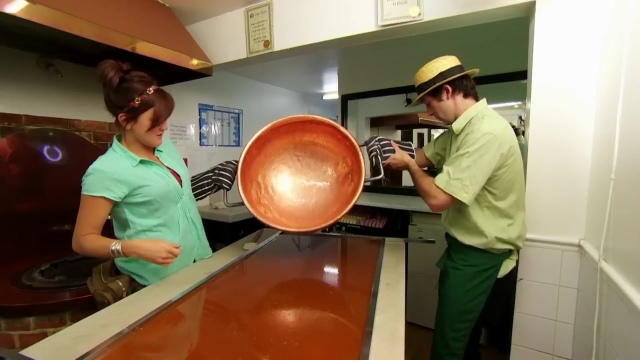 lovely creamy taste. Can I have a go Patch? Of course you can. It's very hot, Very, very hot. now Fudge has to be at just the right temperature before we can pour it out. Wow, that is amazing. As the fudge cools down, it changes colour and it becomes more like 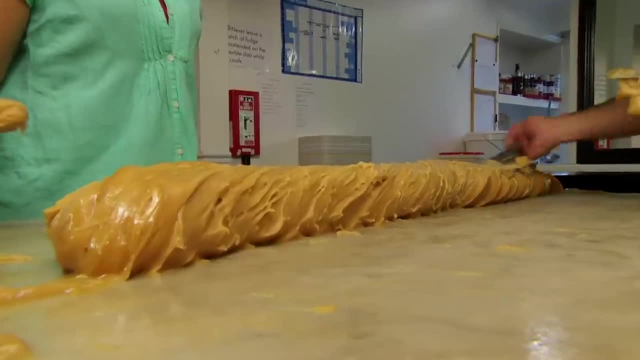 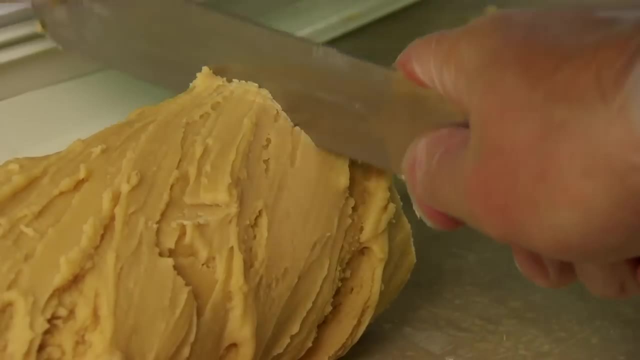 modelling clay. We have to shape it into a big, long loaf And we're nearly done And all we need to do now is slice it. There you go. Thanks, Patch. So here it is our lovely fudge, all ready to use in our fudge. 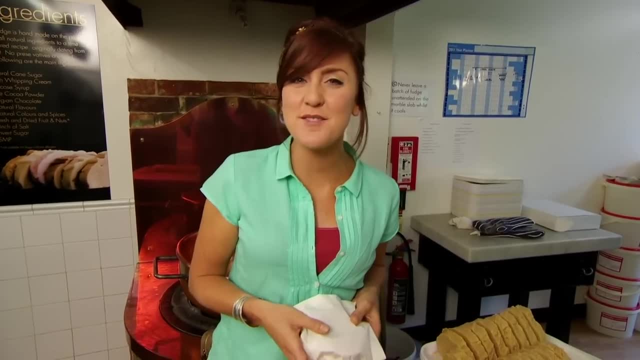 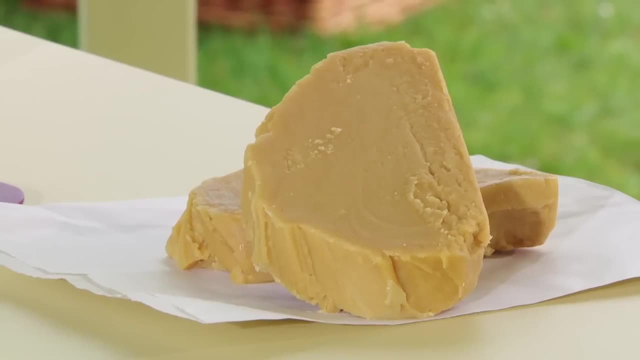 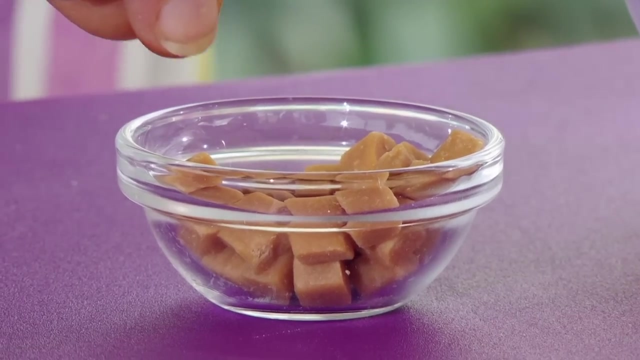 Wow, Our lovely fudge, all ready to use in our fig and fudge biscuit. Can't wait. I really enjoyed making this fudge. It was really interesting, wasn't it? Now you've got some fudge on your tables too. They look like little fudge building blocks. What do they? 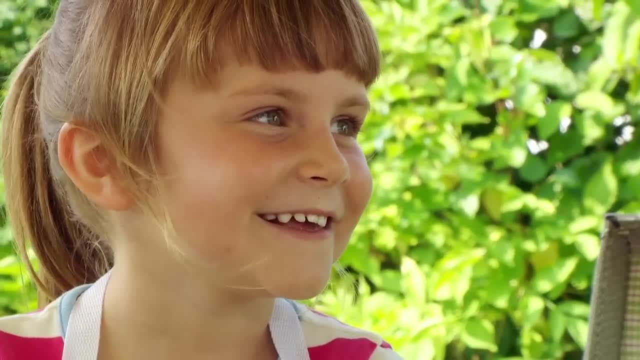 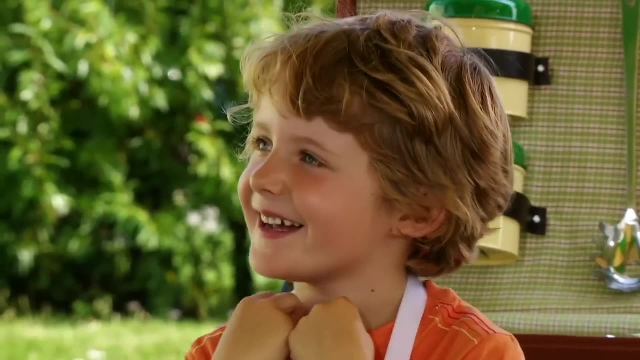 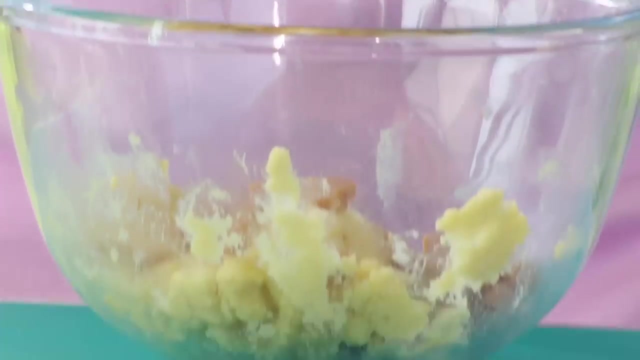 feel like They're really squishy. Can you imagine if you had a house made out of fudge? I'd eat it. You'd eat your house. Oh, that would be delicious, wouldn't it? Yeah, OK, let's put this fudge into our bowl with our other ingredients. There we go, OK, next. 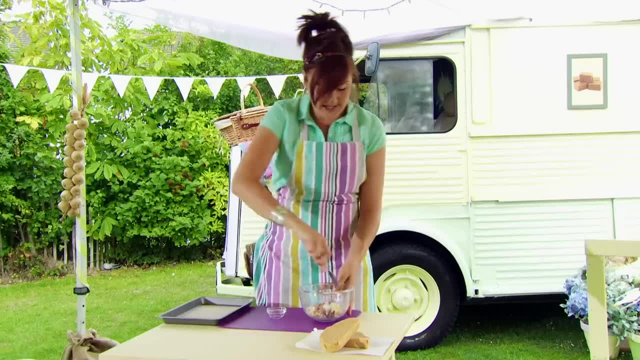 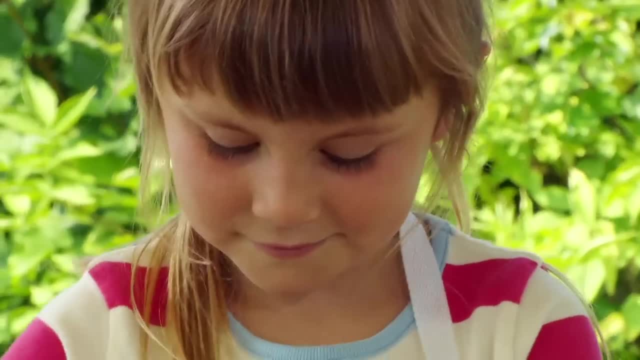 we need to give everything in this bowl a good mix using our spoon. There we go. What are we going to do? everybody Dig down deep And you can mix with us too. You just need to get your bowl and then you need to get. 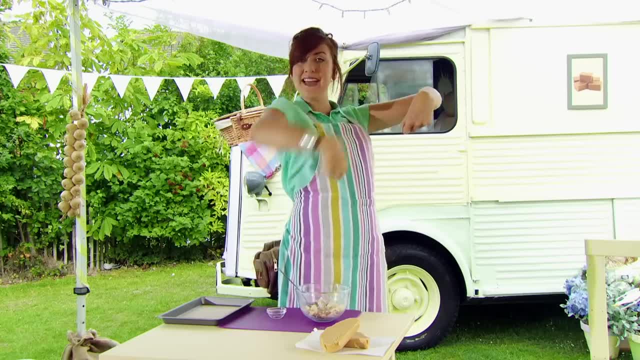 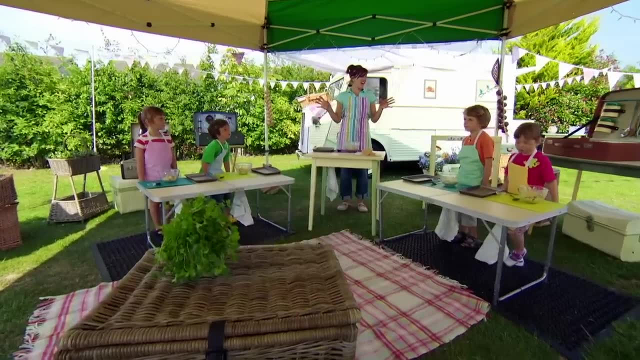 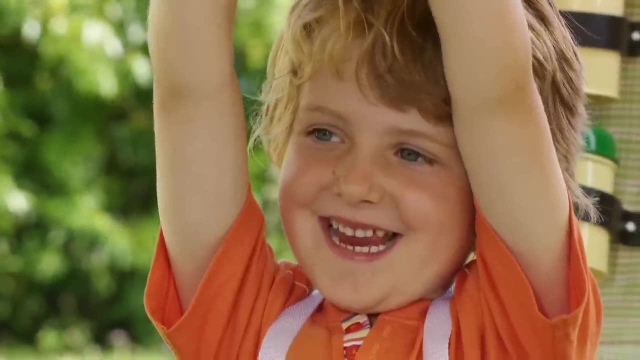 your spoon and you go: mix, mix, mix. And now it's time to get our hands really messy. Yay, Who likes getting messy? We? We're going to make a fig and fudge mountain and I'll show you how to do it. You need to. 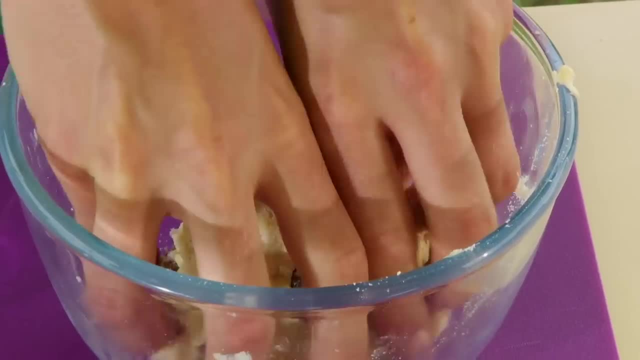 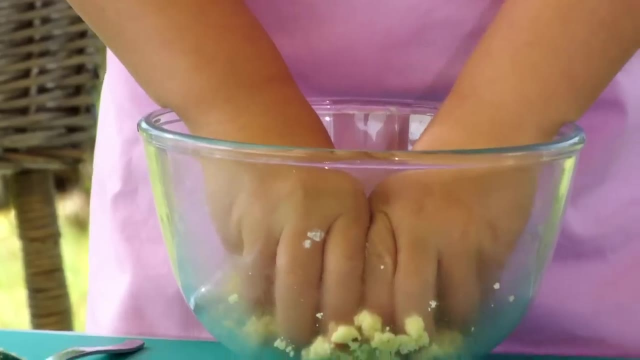 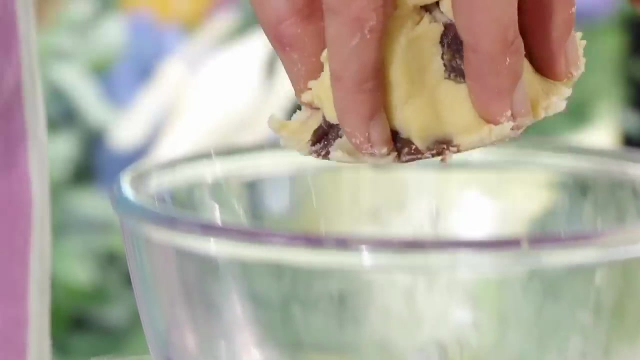 put your hands into the bowl and squeeze the mixture together so you make a mountain at the bottom of it. Look at this. Look at my mountain, Toby, that's fantastic. Pick the mountain up, Look at that And put it on your mat. 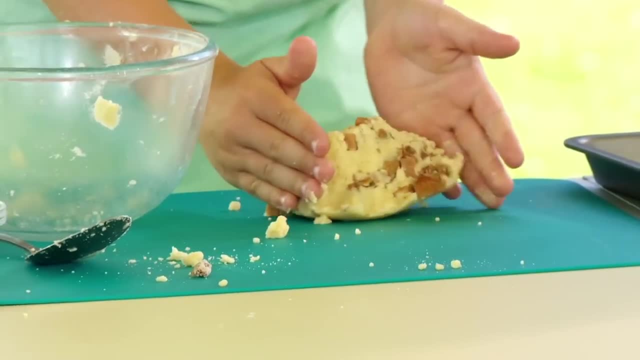 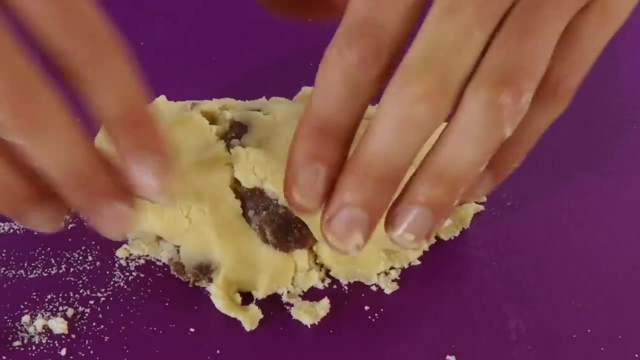 Pick it up really carefully- I've done it- And then, once you've got your mountain on your mat, we're going to make it into a long sausage, Push it down flat and make it into a sausage shape. It looks like a caterpillar actually. 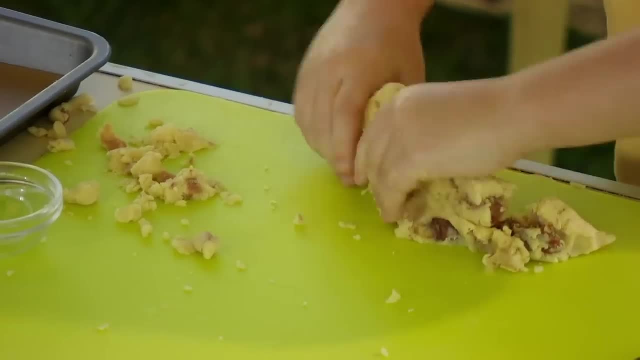 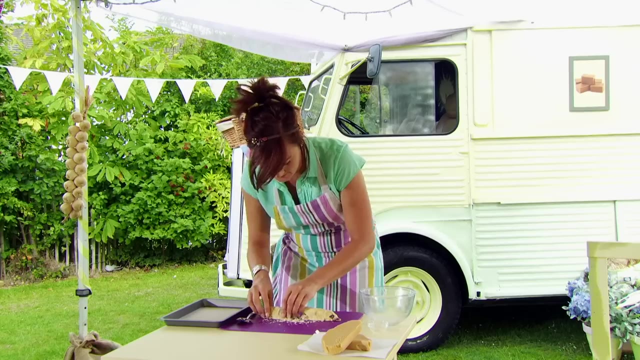 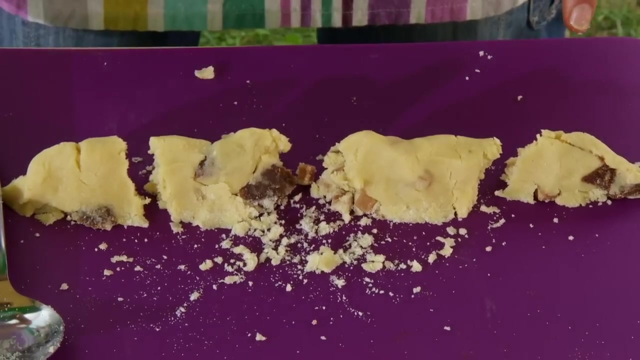 A fig and fudge caterpillar. OK, now we need to split everything into eight pieces. So split it in half, and then we split these two pieces in half, like this, and then we split each of these pieces in half. So let's count all of our pieces. 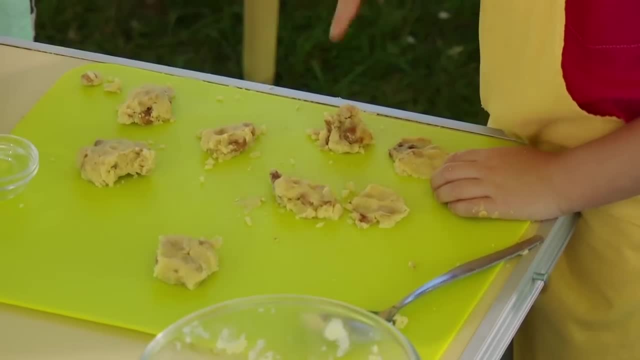 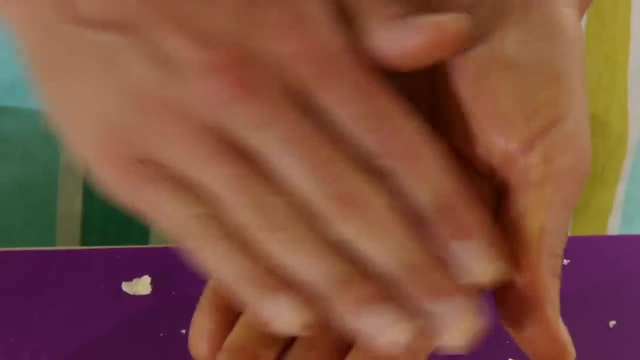 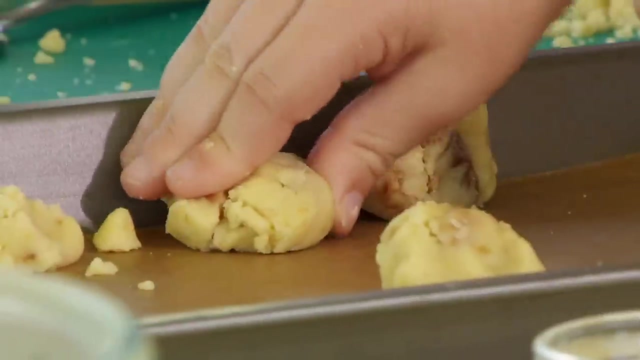 One, two, three, four, five, six, seven, eight Beautiful. Pick up each piece and put it in your hand, and then we're going to roll it like this, Make it into a ball and then put that there. Katie, look how Ivy made it. 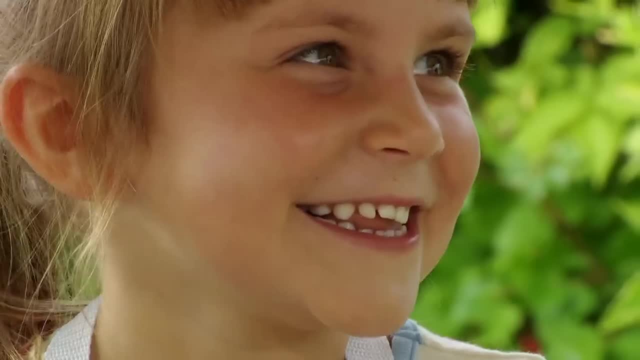 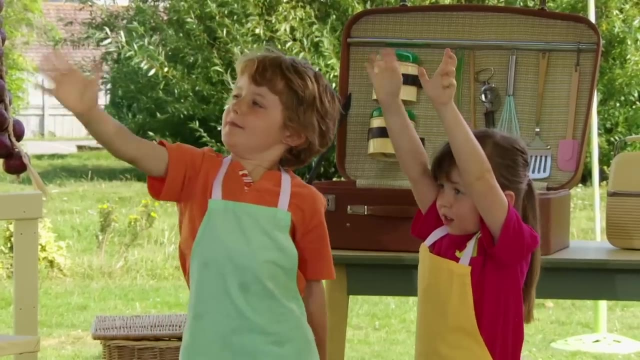 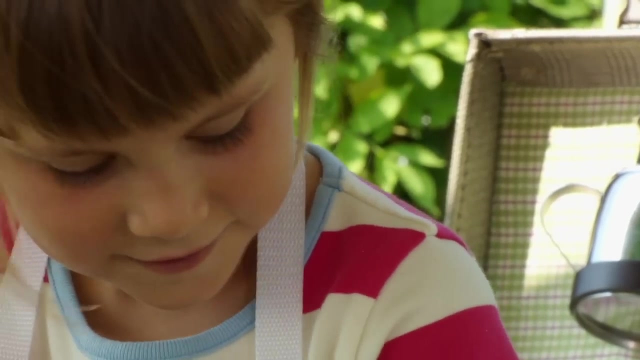 Ivy rude. That looks absolutely perfect. OK, everyone show me your hand like this and then give it a wave, because we're going to use this hand to flatten our fig and fudge balls. Squash, Squish, Squash. 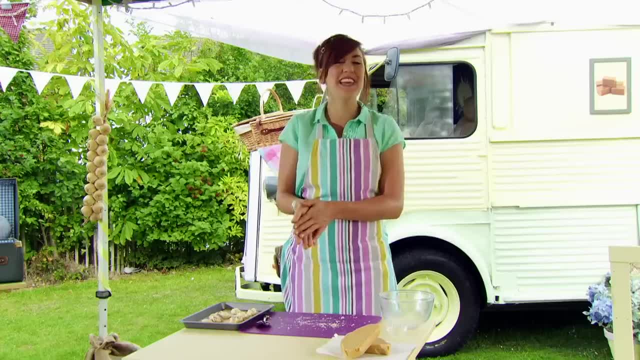 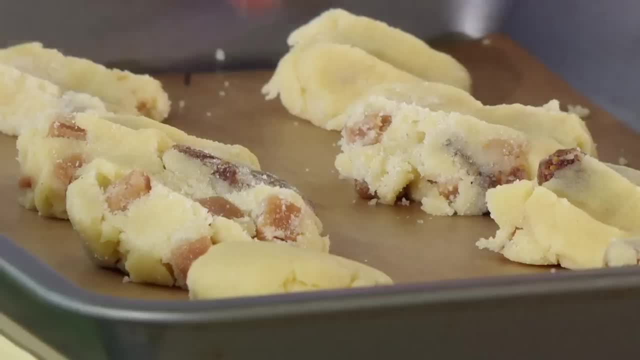 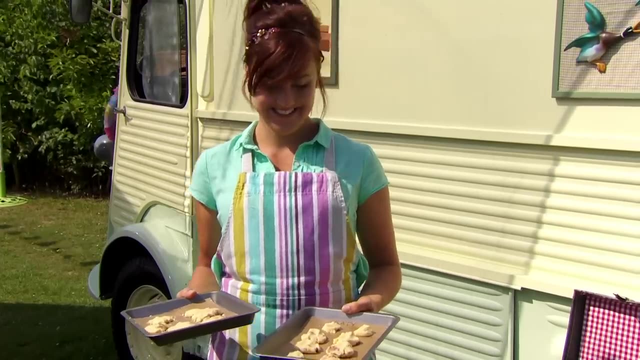 And that is it. You did it. You put all the ingredients together for your fig and fudge biscuits all by yourself. Well done, And now we just need to put them in the oven. But remember, ovens are hot, so don't go near. Ask a grown-up to help you here. 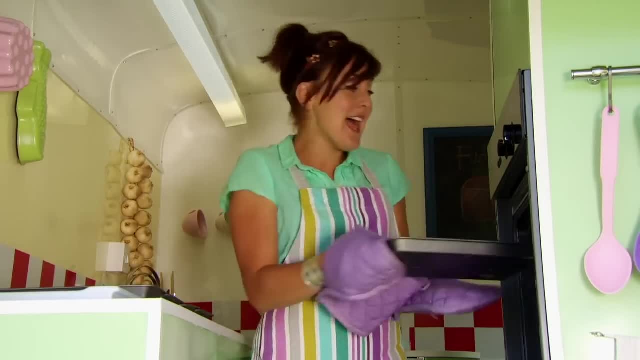 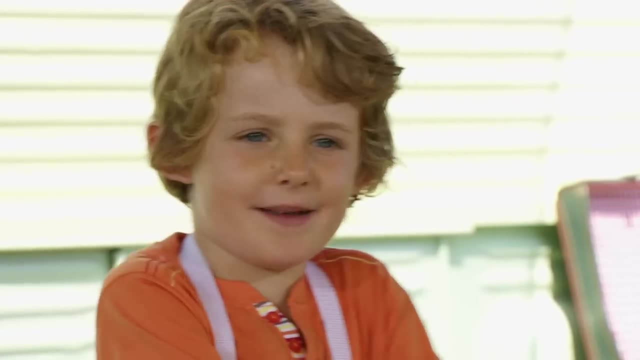 Now we've cooked with you and had lots of fun. Let's tidy up and think of all the things that we have done. There was: Mix it, Scrape, Scrape, Scoop, Scoop, Scoop, Scoop. 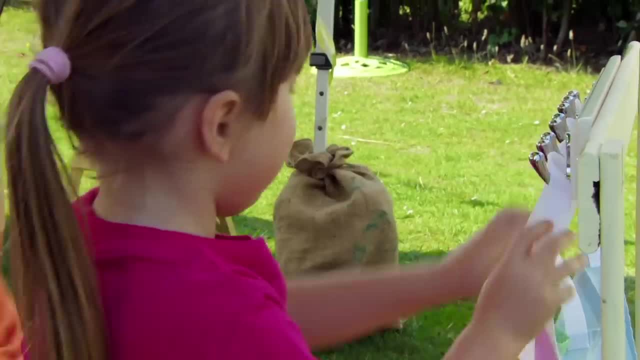 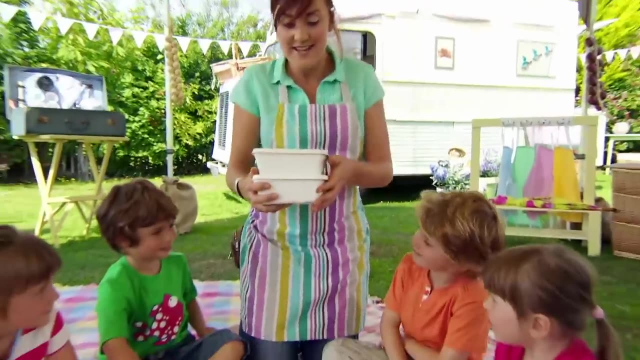 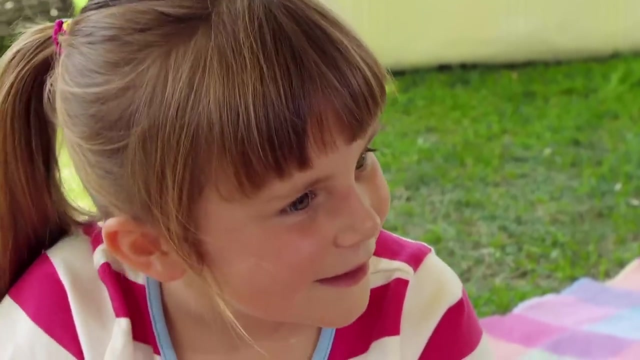 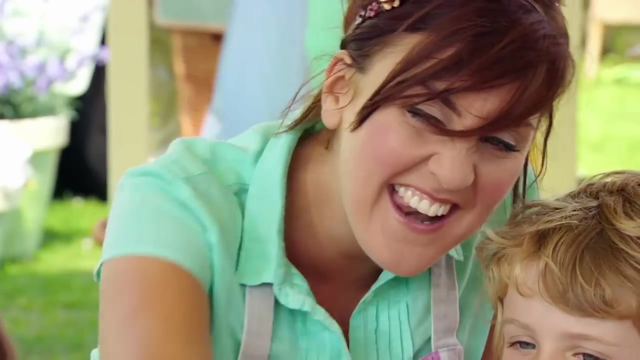 Scoop, Scoop, Scoop, немножко Scoop, Scoop, Scoop, Scoop, Scoop, Scoop. So here it is, We're getting there. Oh yeah, look, it looks like a duck foot. 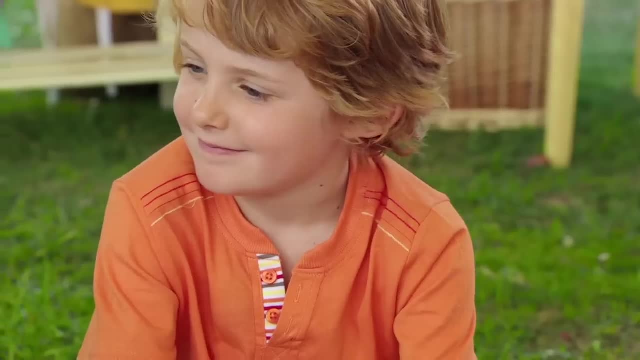 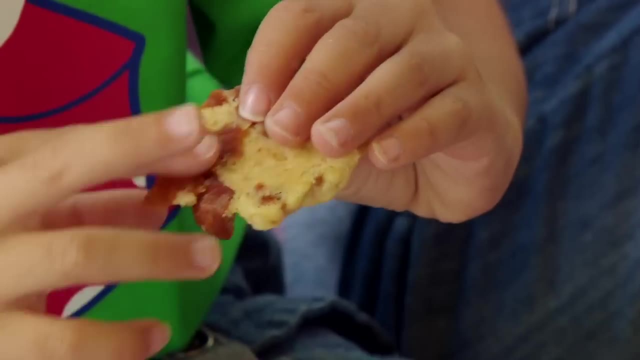 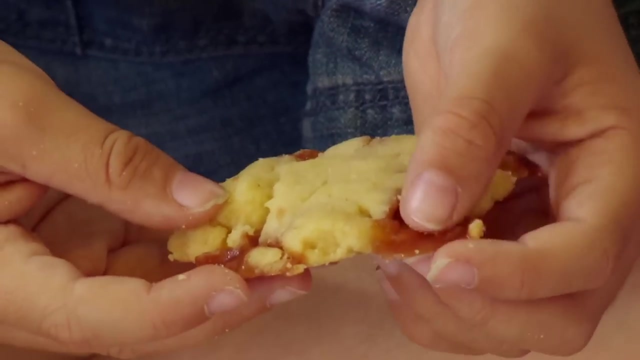 Because that bit looks like the toe bits. OK, let's have a look at Toby's next. Hey Toby, what do you think of your biscuits? It's gone smooth on this side and bumpy on this side. It looks like a treasure island and all these melted fudge bits look like exploding volcanoes. 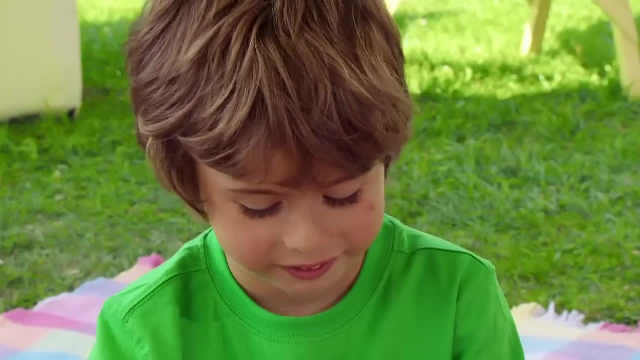 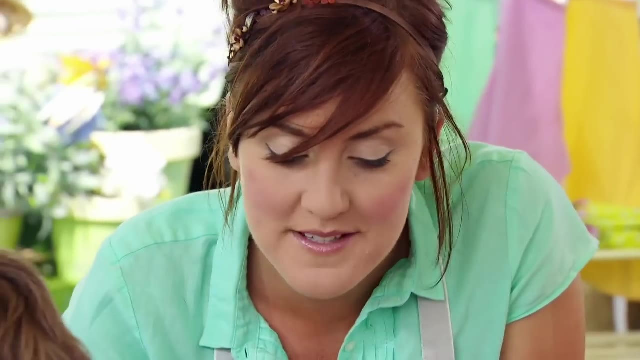 Yeah, and that bit looks like a cannon. Do they smell good, Toby? Yeah, I just had two, Toby, I think your biscuits look absolutely fantastic. OK, everyone, let's put the lids back on top. We've travelled to you, cooked and had fun. 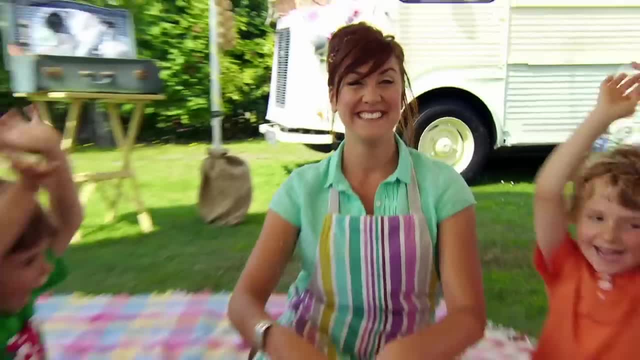 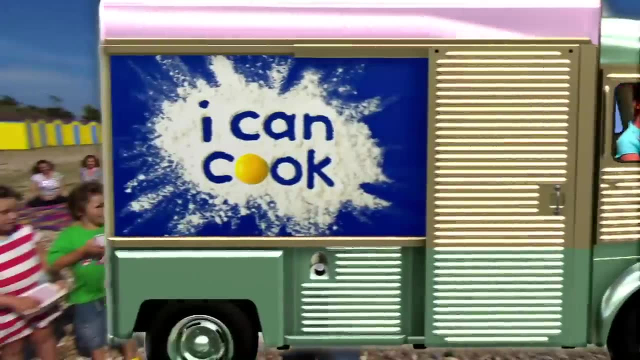 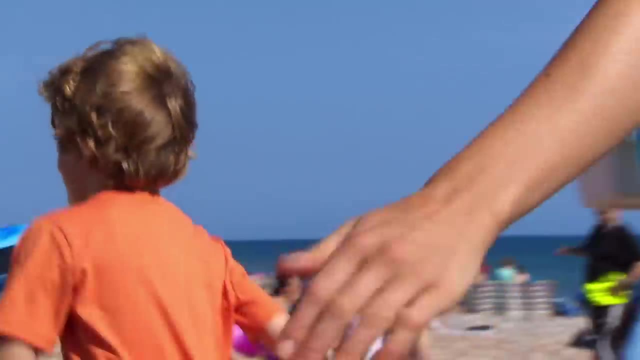 Now let's have a party with everyone. Yay, Come on, you can come too. Follow me. We're at the beach and we've got our delicious food to share with everybody. Come on, everyone. I'm so excited. Look what I made, Mum. 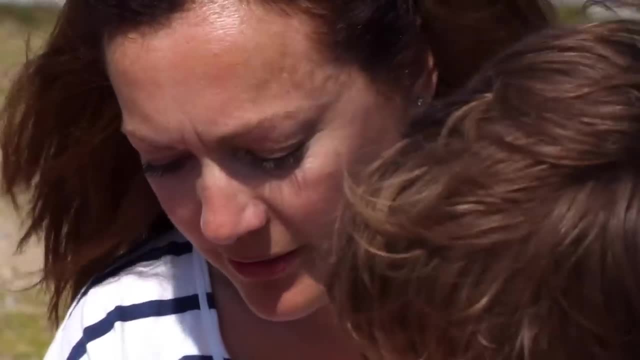 What are these then? Big and fun Fudge biscuits- Oh, they look delicious. What's in them? Fudge? Oh, that's nice. Mmm, Mmm, they're really nice. So what do you think of the biscuits? 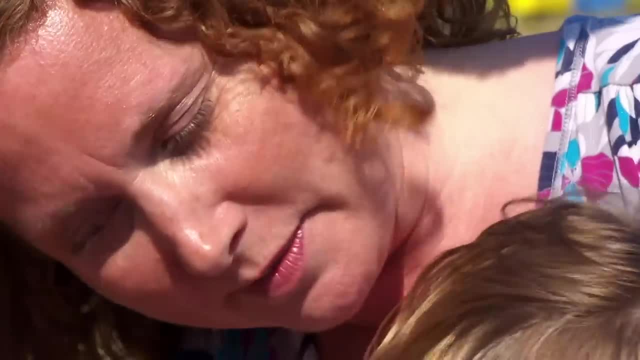 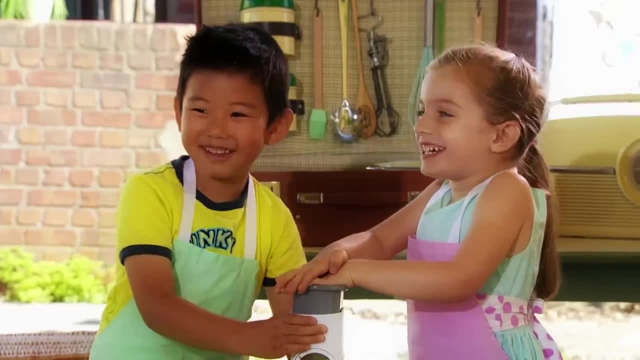 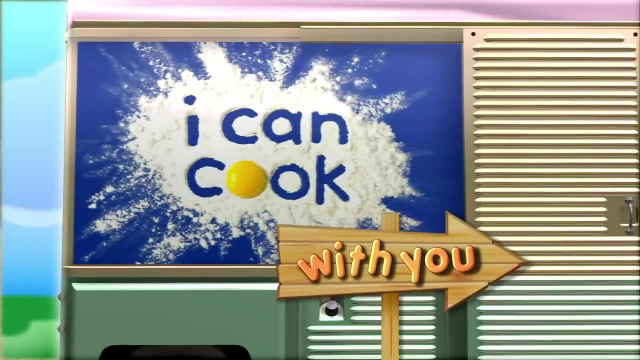 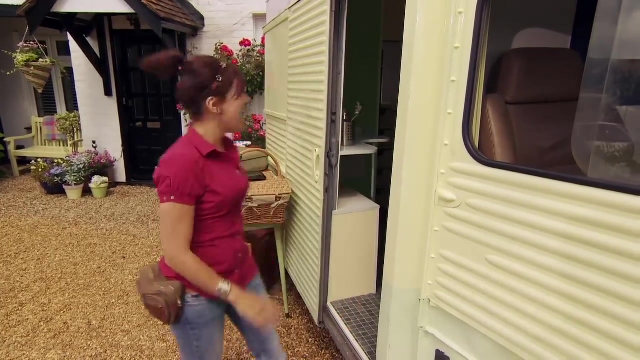 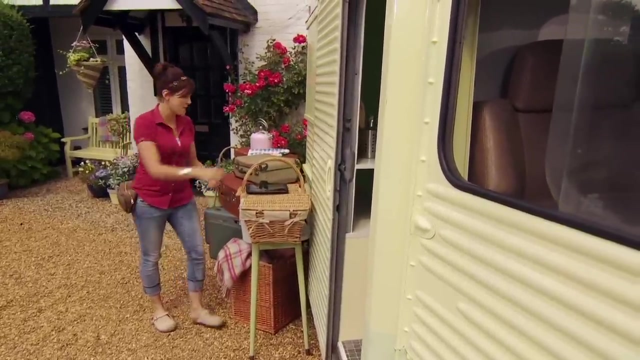 I can cook ges 10 With you. Ah, fantastic, I was hoping you would come along. I've just been getting everything ready to go on a journey and I just hope you're going to come too and meet some new friends. 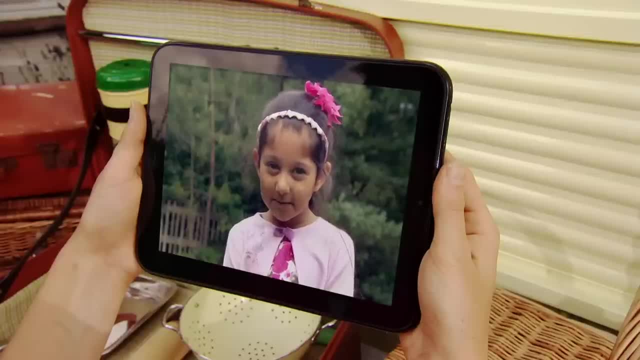 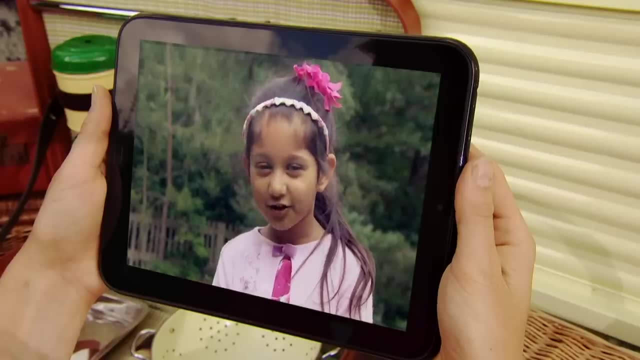 Ah, brilliant, Katy. I like having teddy bears too. I like having teddy bear picnics in the forest, and I like cheese. Oh, that sounds fantastic. Katie, can you cook with me please? I can Just Jot And you can cook with me too. 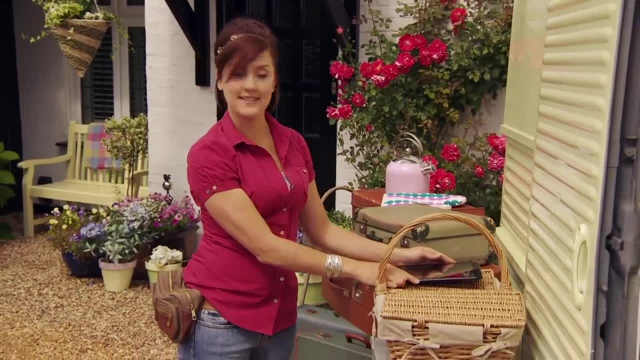 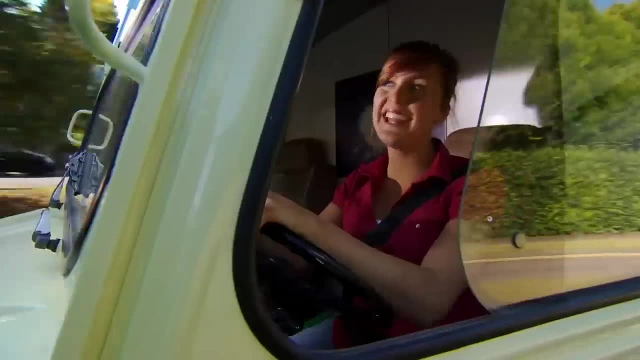 Oh, I haven't been on a teddy bear's picnic in ages. Right, let's get everything packed up as quick as we can and get on our way. All on a journey, and I'm coming to you. It's going to be busy and there's lots to do. 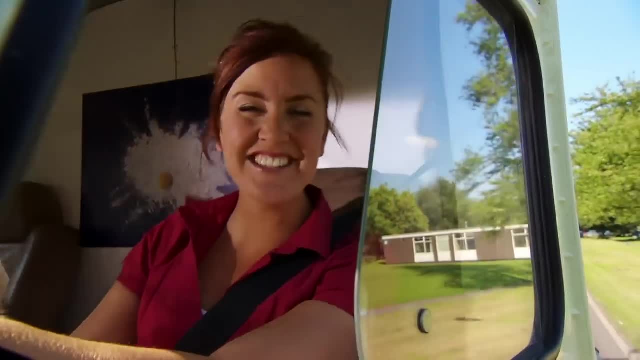 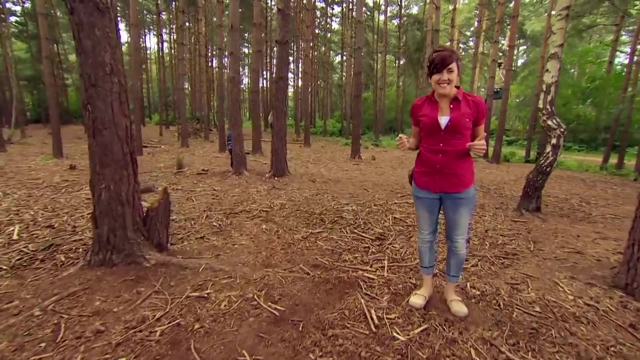 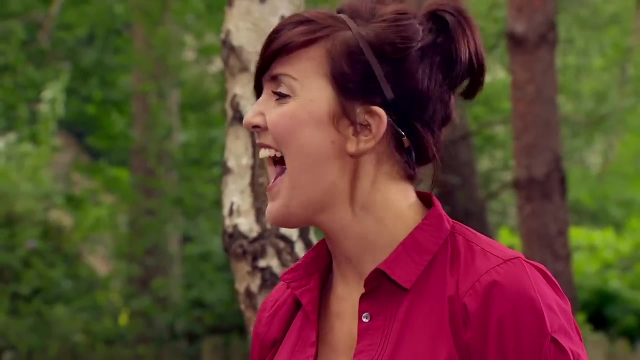 Get ready to help, join in and have fun. Let's cook a feast for everyone. Well, here we are in the forest where I've been invited by Just Jot. But where is she, Katie? There you are, Just Jot. 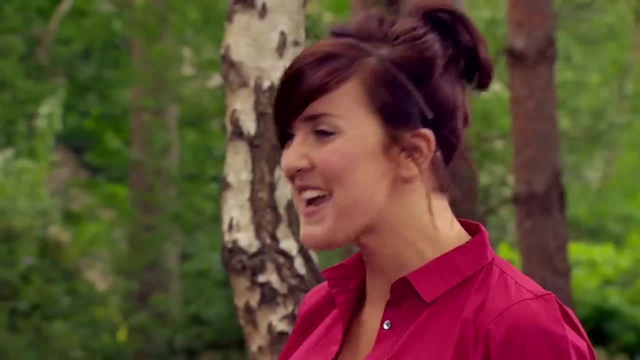 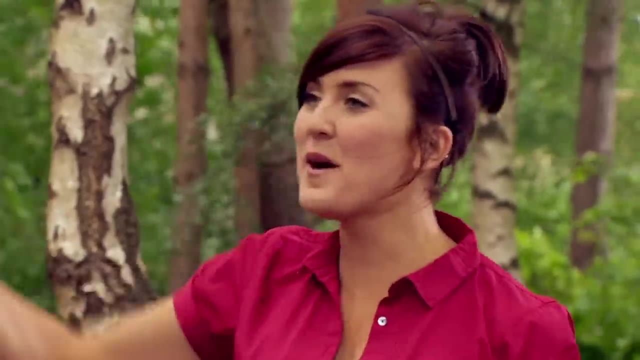 And hang on. who are all your friends hiding behind the trees? I'm Jake. I'm Rose. I'm Haiyan, Haiyan, come on over everyone. Great to meet all of you. So what are we going to do today? 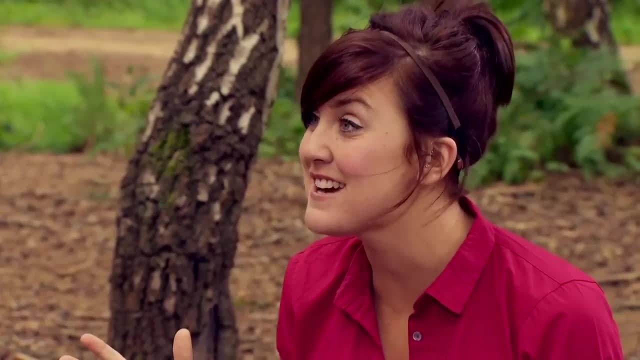 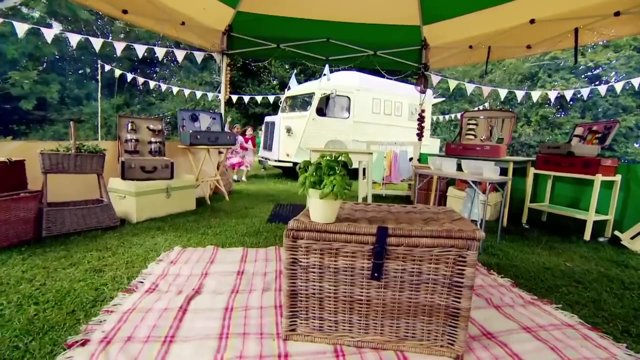 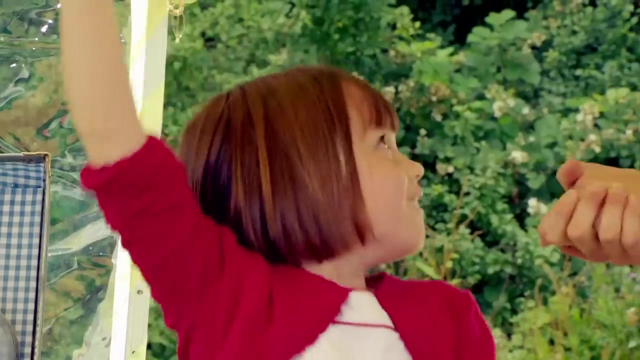 Let's have a teddy bear picnic And I've got the perfect recipe for us to cook. Follow me. Welcome to my outdoor kitchen. Now. who wants to know what we're going to cook today? Me Well, today's recipe is the scrumptious, the delicious. 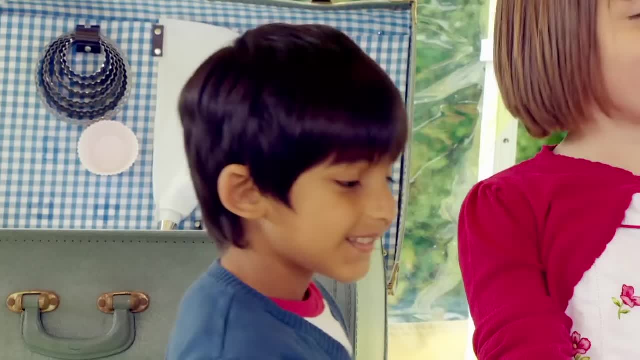 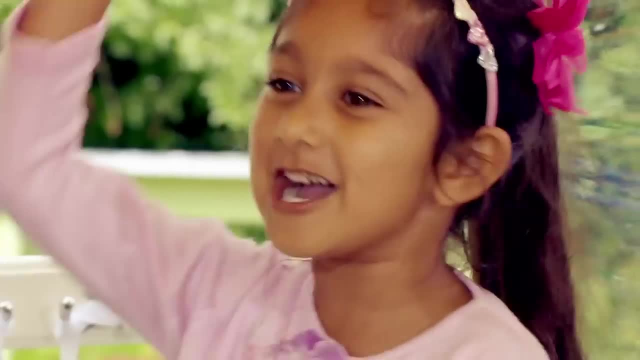 cheese and tomato melts. They look good, don't they? Yeah, But before we get cooking, we've got to do something really important. Does anyone know what it is? Wash our hands. That's right. we need to wash our hands. 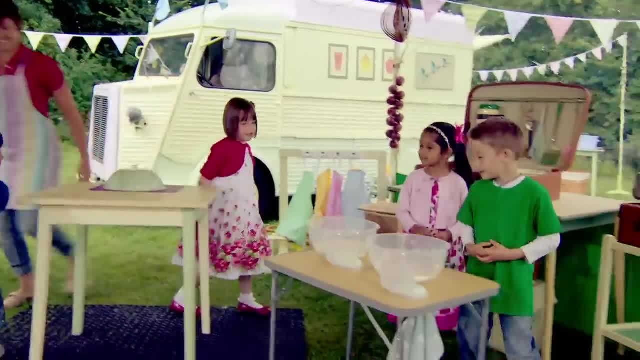 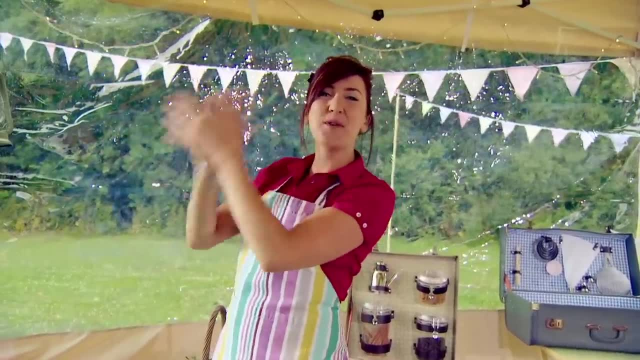 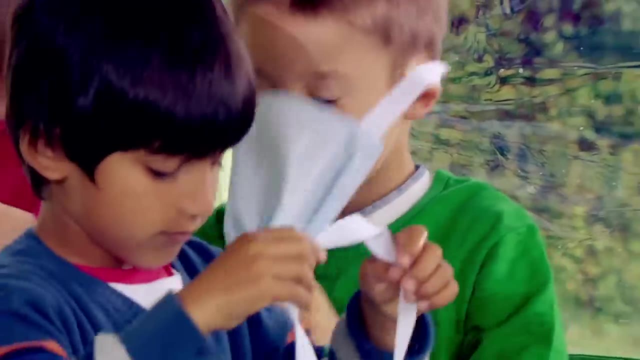 So let's get going. Roll up your sleeves, Give your hands a wash With slippy, dippy soap, Splish, splash, splosh. Have you done your hands Washed and dried? Sleeves rolled up, Apron tied: What can you do? 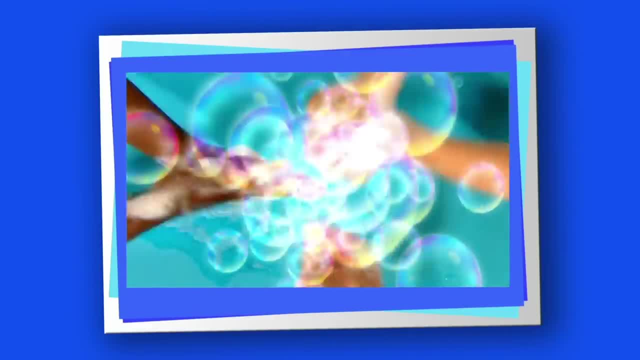 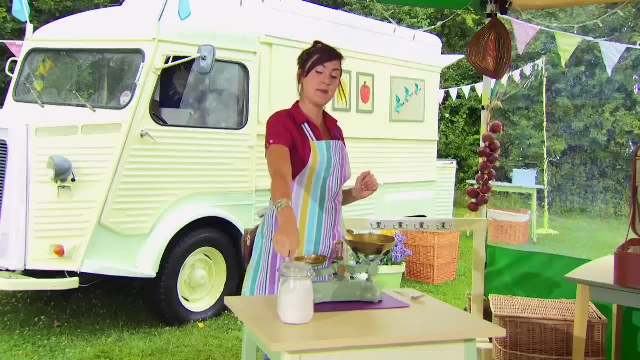 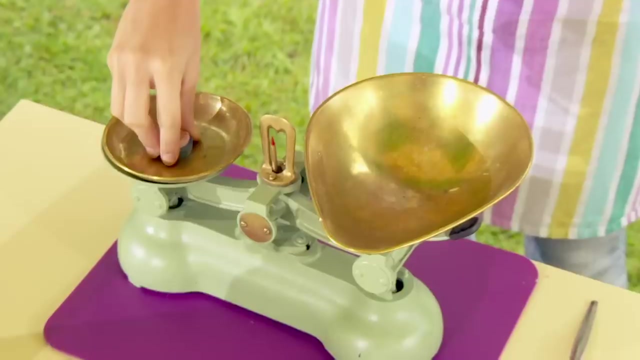 I can cook. Right, let's get started. So the first thing we need for our cheese and tomato melts is some plain flour, And we're going to do some weighing Now. I've got some scales here and these weights weigh the same as the amount of flour that we need. 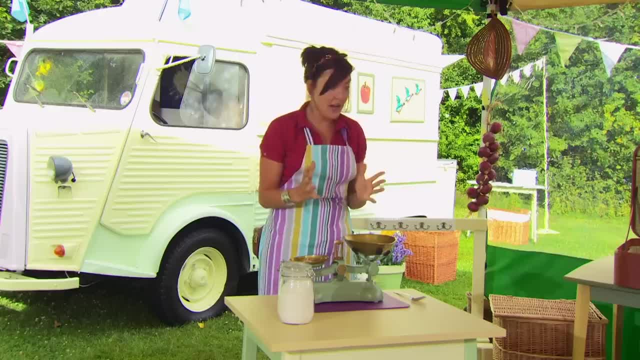 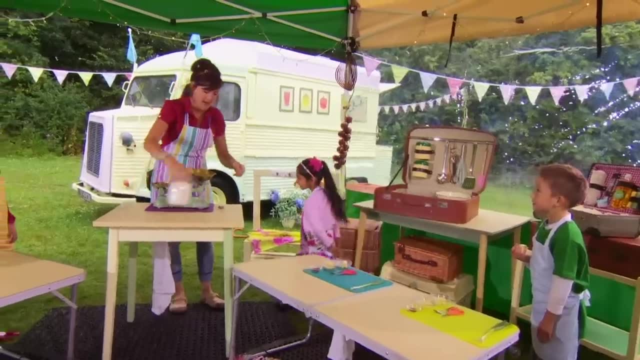 which we're going to put on this side of the scales. So what I need you to do is shout out if we need more or less flour. So Just John, you can come over and help me and you can scoop the flour out with that spoon and put it into our scales. 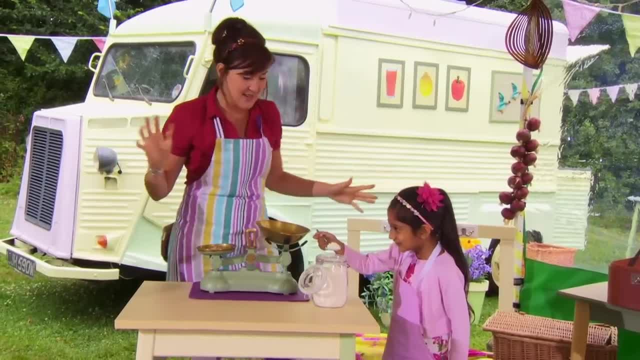 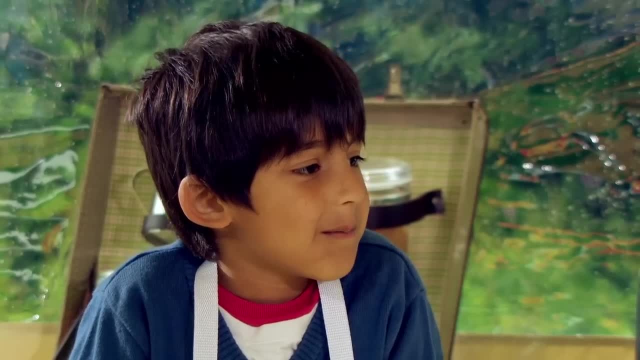 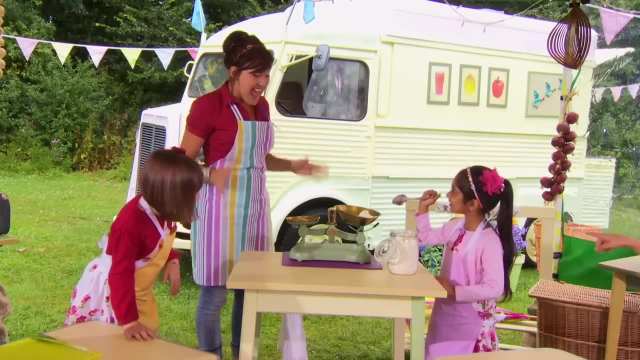 Everyone. are you ready? Yeah, Okay, team, let's go More or less More. Okay, why don't you put a really big mountain of flour in Less, Less, less, less. Wow, that was perfect. 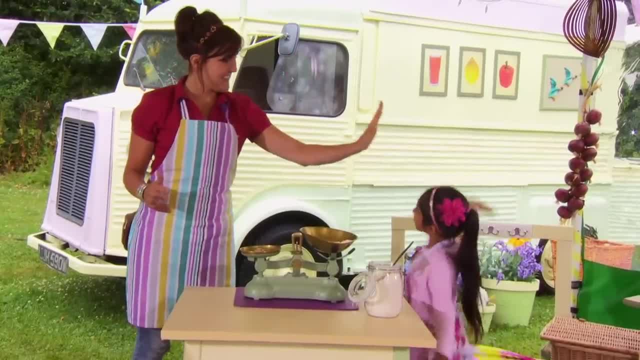 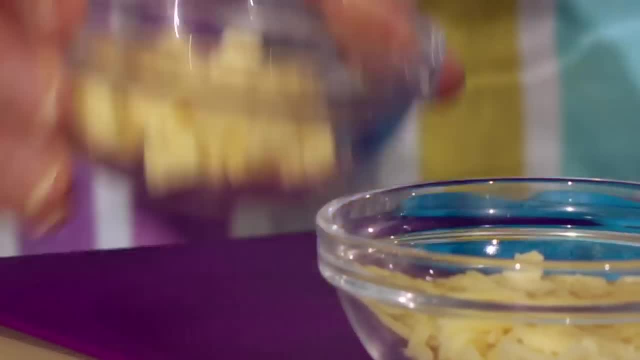 Just John, you did such a great job. Give me a high five. Yes, fantastic, Well done everyone. Next, we're going to add some butter into our flour, So we might need to use our fingers for this and scoop it out into the flour. 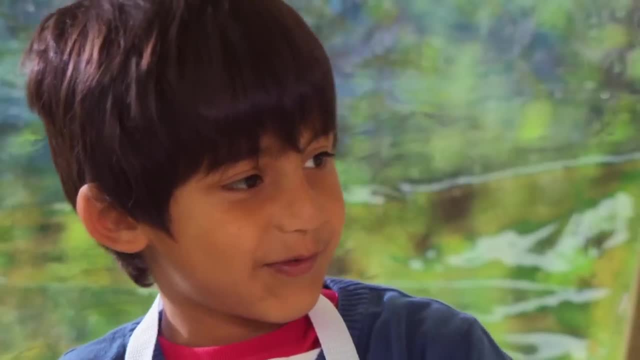 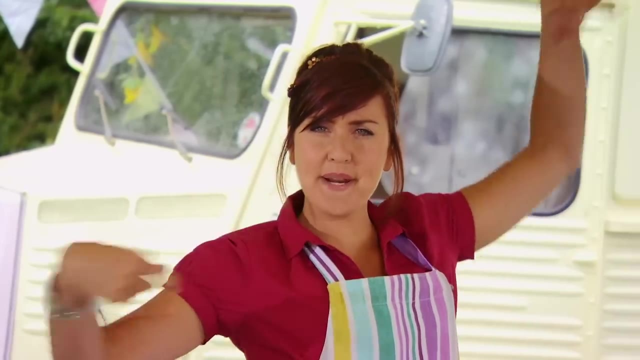 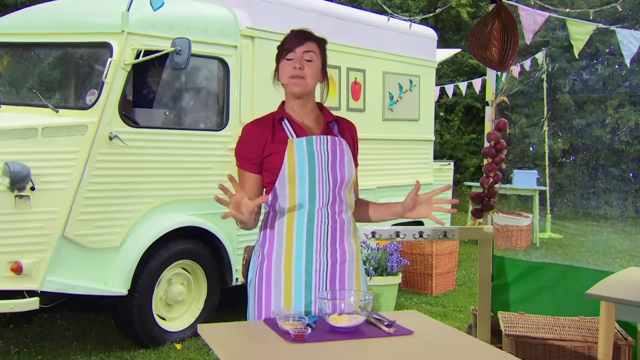 and it makes a big boof noise- Ready Boof. So next we need to add some of this, and it's called paprika. Who can go paprika Paprika? Okay, let's add a pinch of paprika, and for that we're going to need our good friend, the pinchy parrot. 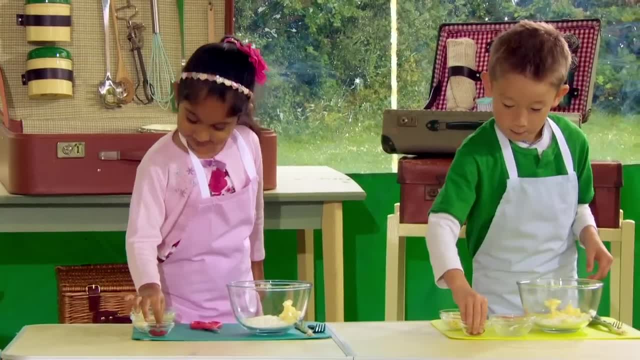 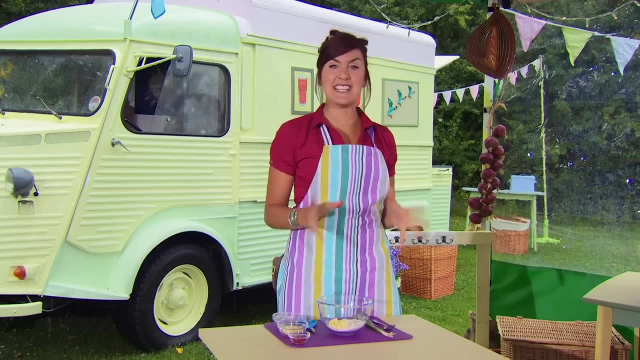 And take a pinch of paprika with your pinchy parrot, and that's going to add lots of delicious flavour to our cheese and tomato melts. Next, we need to tickle the butter and the flour together with our fingers, So let's get tickling everyone. 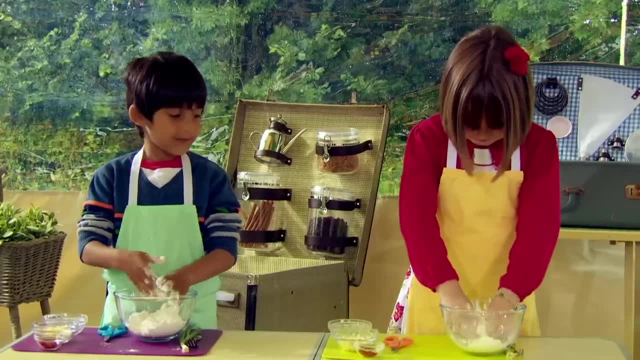 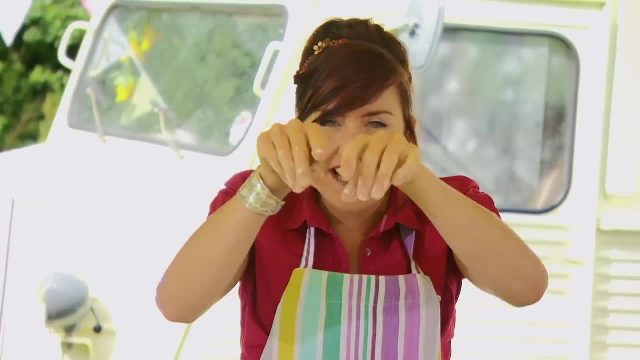 Make sure we get all of those lumps out, team. Oh, it's so soft on my fingers, And don't forget to tickle with us. You go, tickle, tickle, tickle. Brilliant job, You're a top tickler. 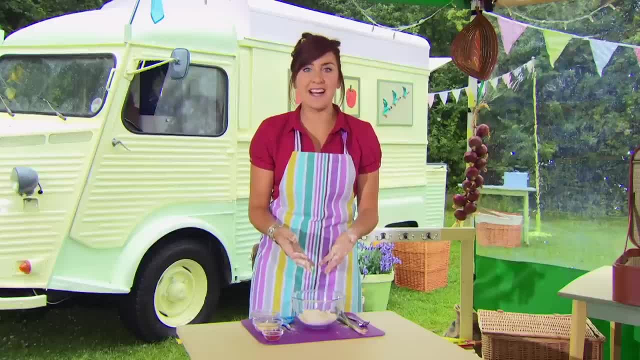 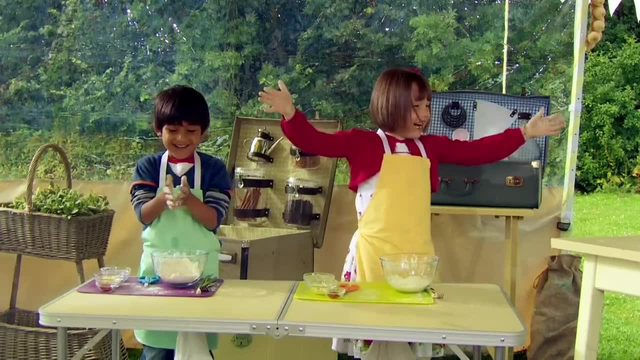 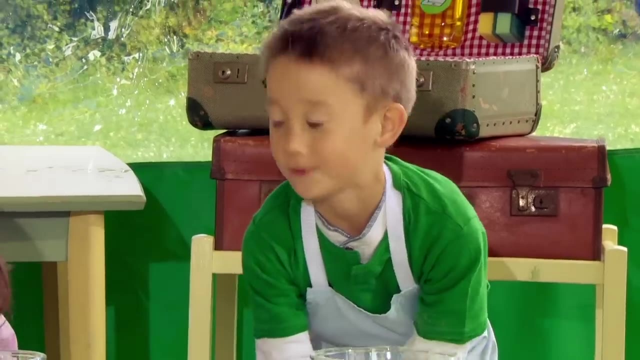 Then, when you've finished, you can make a flower cloud with your hands Ready After three. One, two, three, Boof, Woohoo, And that'll give your hands a quick wipe. Okay, the next ingredient is a spring onion. 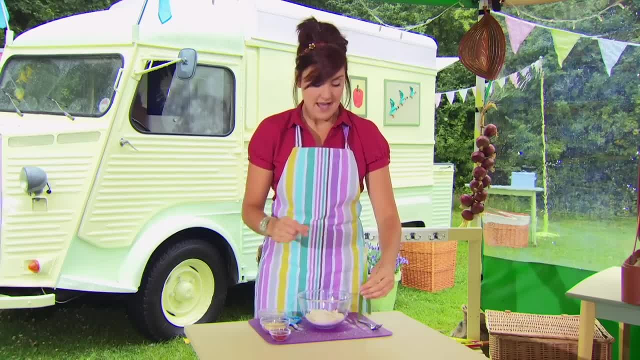 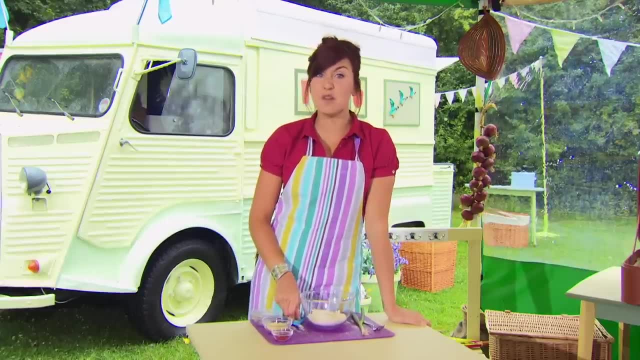 Now we need to give Mr Spring Onion a bit of a haircut, and to do that we're going to use some scissors, But remember the safest scissors. everybody knows that we point them down towards our Cows, That's it. 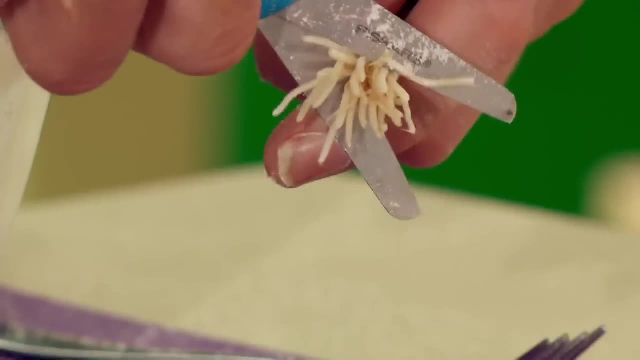 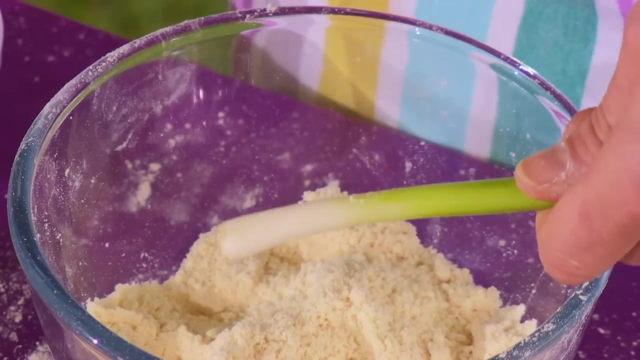 So give Mr Spring Onion a little haircut. Oh, that's it, And now we're going to snip the spring onion into our bowl. So hold it over the bowl and get snipping. Oh, it's very springy. 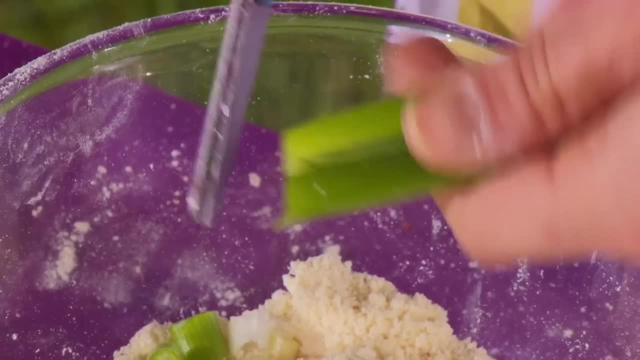 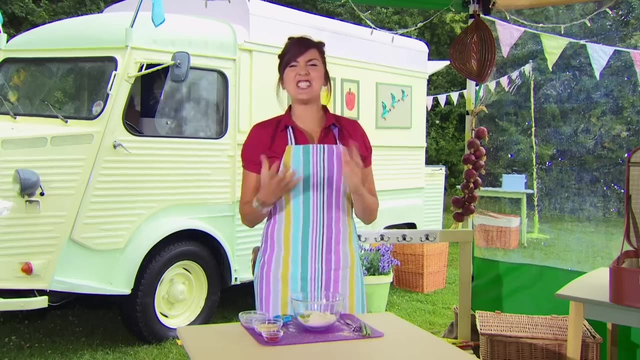 So keep snipping until you get to this part, and then you can stop there and we can put this part in the recycling bin. Our next ingredient is cheddar cheese. Cheddar cheese, Cheddar cheese- Now, cheddar cheese is delicious. 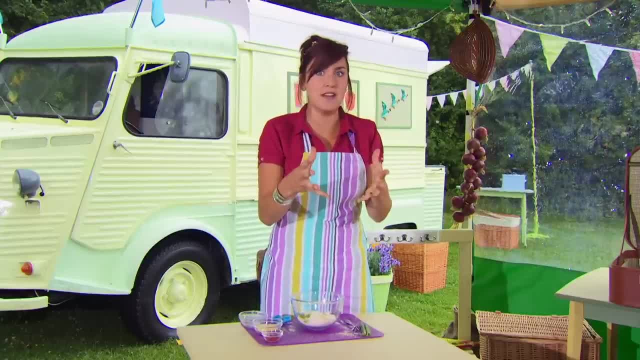 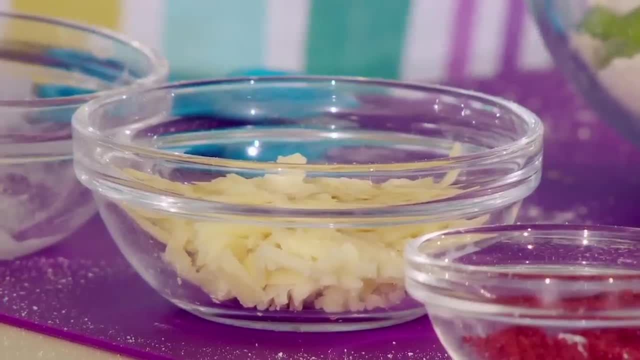 and when you put it on toast and put it in the oven, it all melts. and that is exactly what's going to happen when we put this cheddar cheese into our cheese and tomato sauce. So it melts. It's going to melt like this. 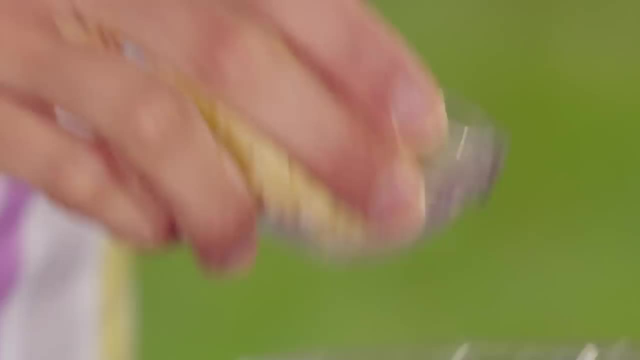 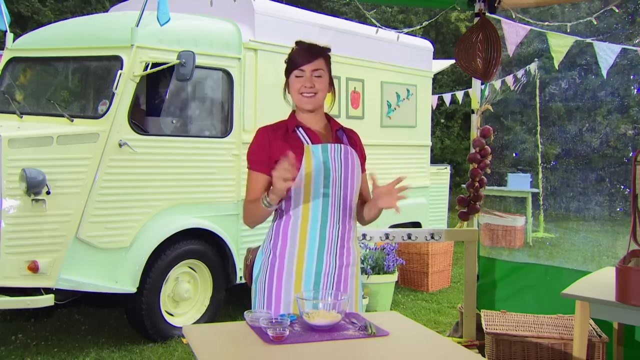 Brilliant. Let's add the cheddar cheese into our recipe, So sprinkle it in And then give everything a good mix, and for that you're going to need your fork. So hold your bowl and let's get mixing. All of the cheese is disappearing. 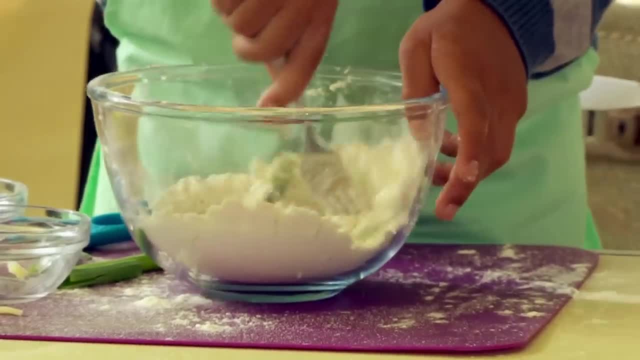 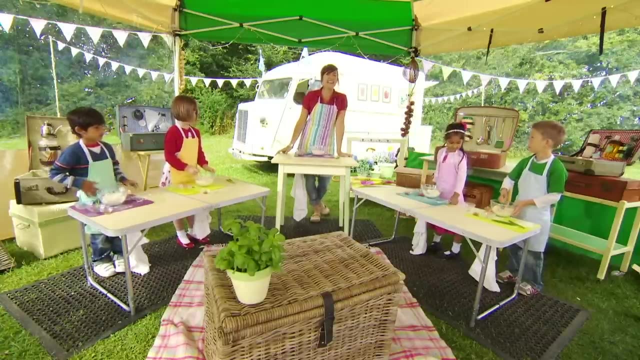 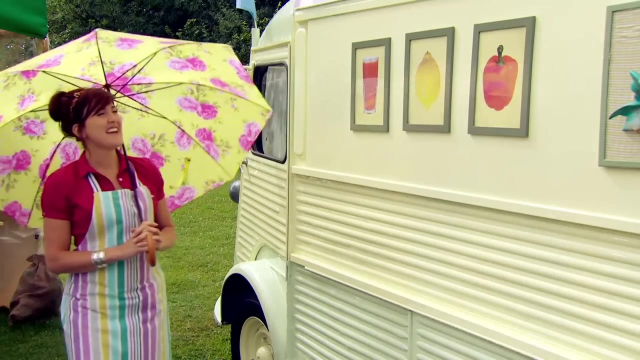 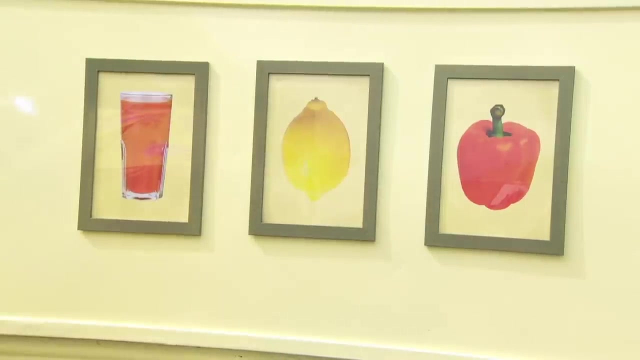 Everything. I wonder what ingredient we're going to need next in our cheese and tomato melts. What is next? Well, let us see if you can guess what it could be. So we've got a red pepper, a lemon and some tomato juice. 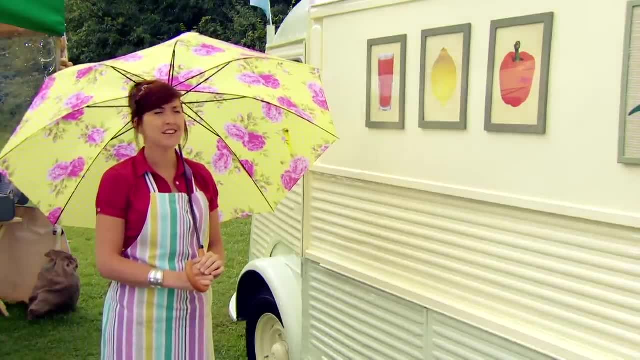 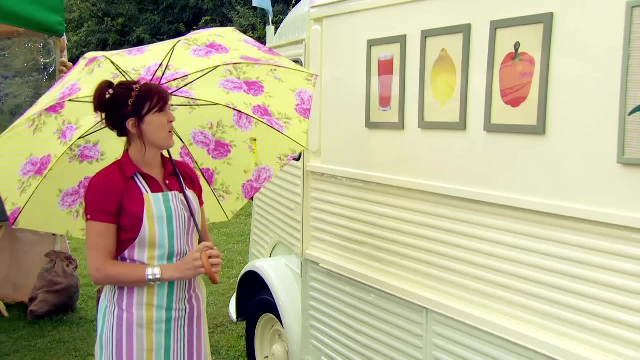 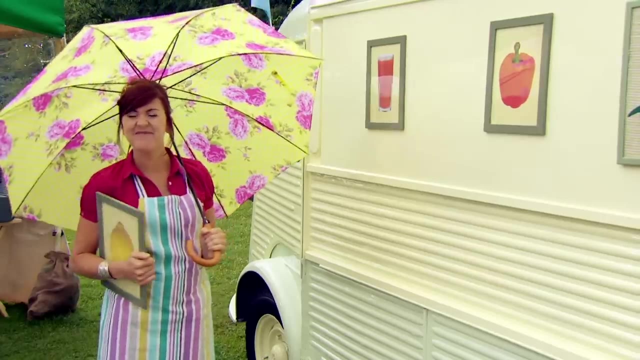 What would you choose for our cheese and tomato melts? Well, the first clue is that the special ingredient is red. Well, a lemon is yellow, so it can't be that one, so we can take that away. OK, here's another clue for you. 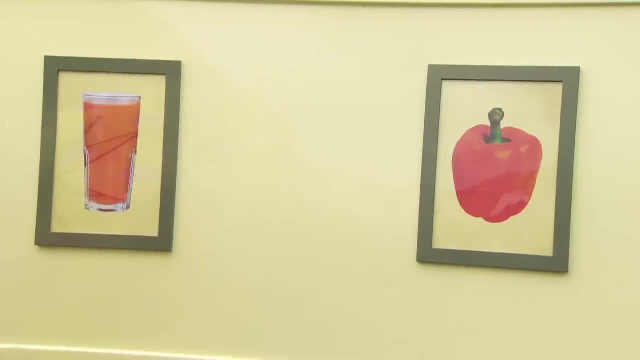 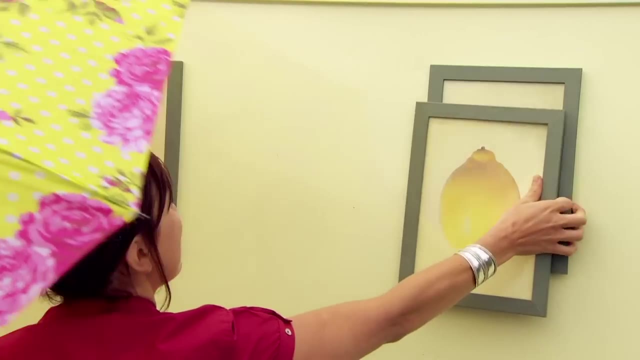 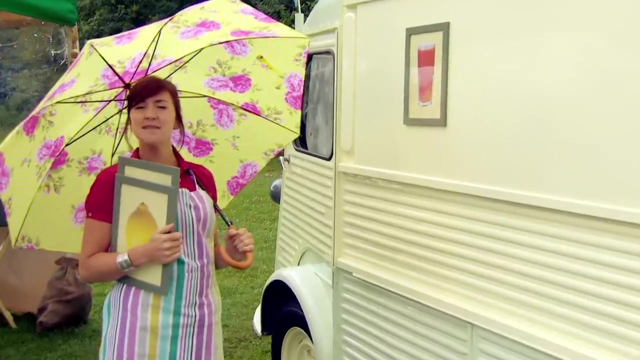 The special ingredient is a liquid. Well, you can't drink a red pepper, can you? So we can take that one away too, Which leaves us with tomato juice. We're going to need some tomato juice in our cheese and tomato melts. 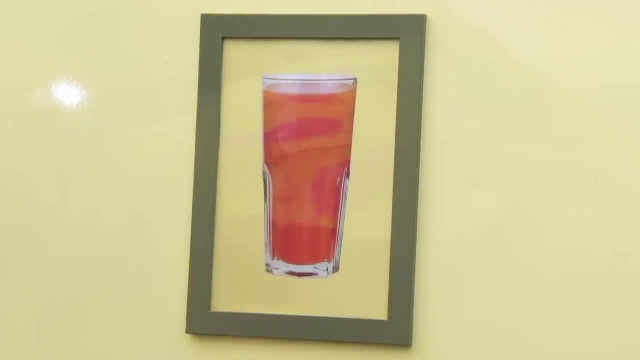 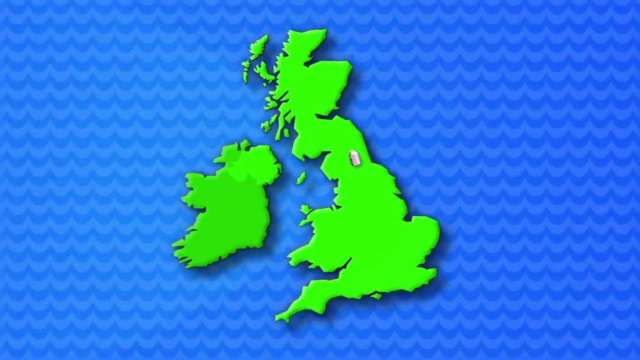 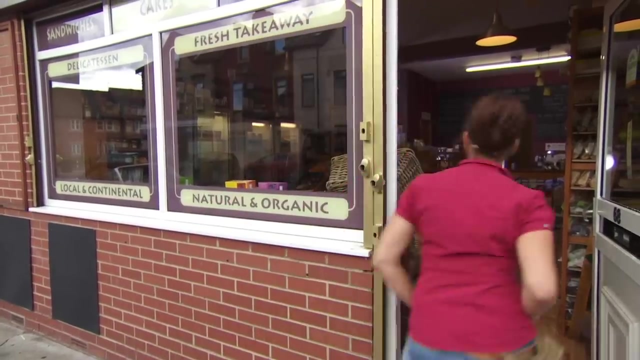 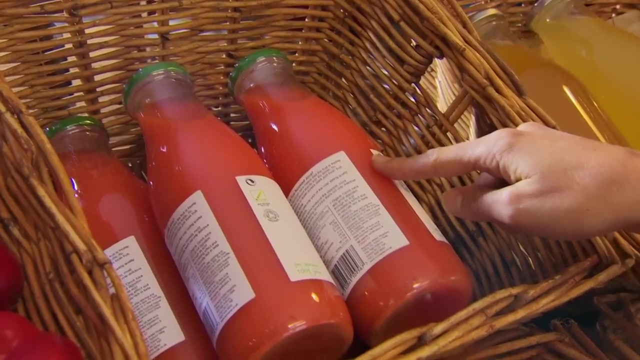 And earlier I went to find some. I've come to a food shop in Newcastle to find out about tomato juice. Let's go and have a look. Juices come from all different types of fruit and vegetables. Carrot juice comes from carrots. 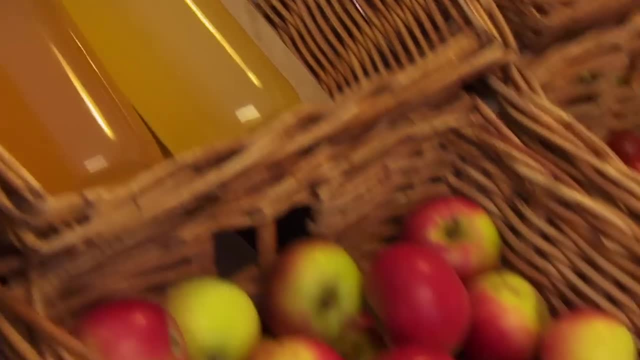 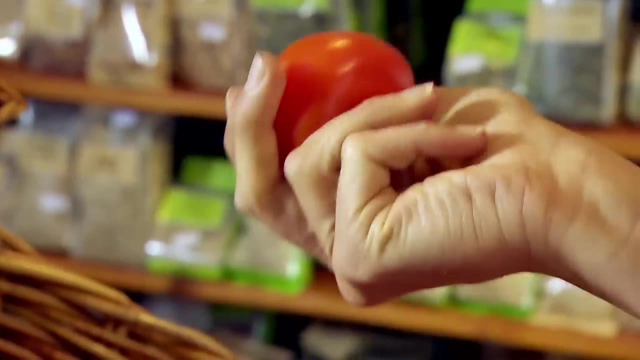 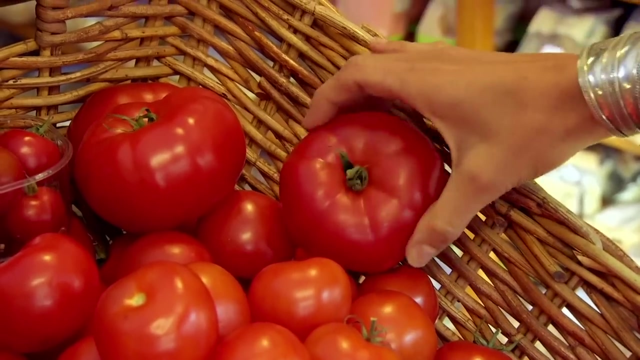 apple juice comes from apples, but the juice that we need for our recipe is tomato juice, and that comes from tomatoes. Tomatoes are a type of fruit and they come in all sorts of different shapes and sizes. These are called beefsteak tomatoes, and these are the ones which are used to make tomato juice. 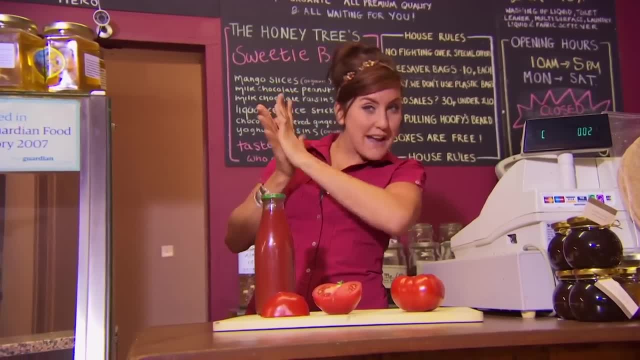 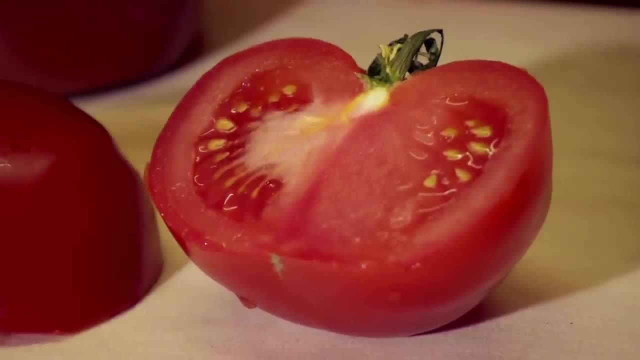 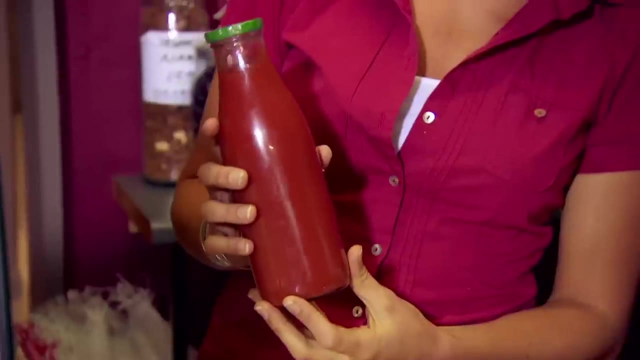 First of all, the tomatoes are pressed together in a big machine. It takes out all of the tomato seeds and it takes off the skins too. The squished tomatoes are then heated up and poured into bottles like these, And in this bottle there are seven beefsteak tomatoes. 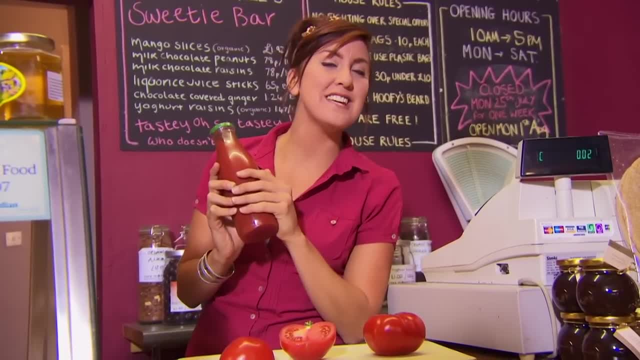 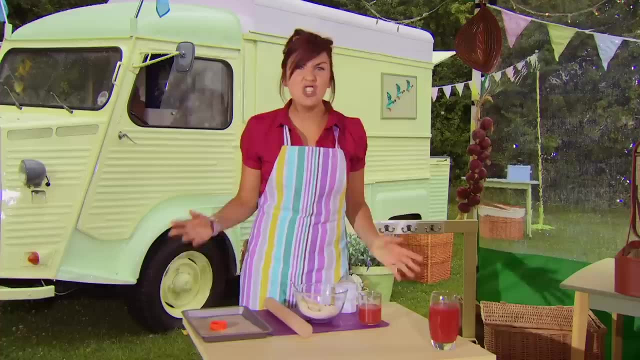 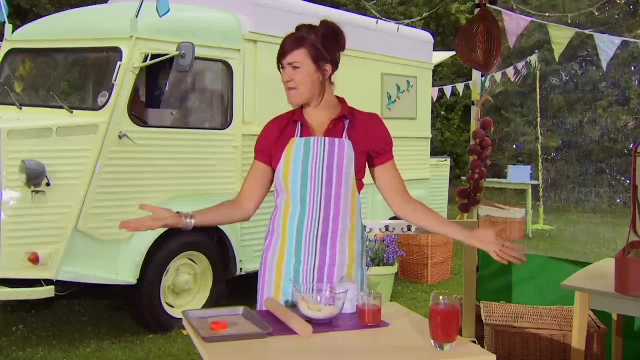 Now, this bottle of tomato juice is going to be perfect for our cheese and tomato melts. It's amazing how many different types of juice you can buy, But for now we're just going to use tomato juice And with it we're going to play the tip and load game. 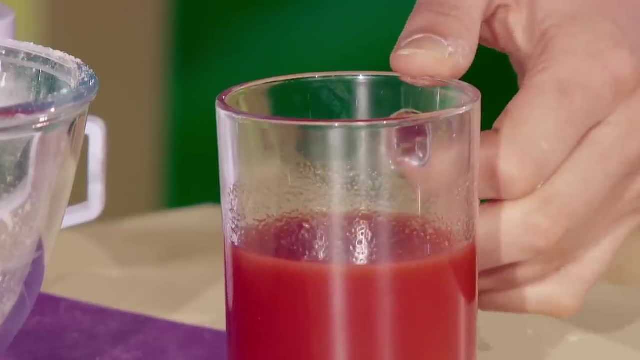 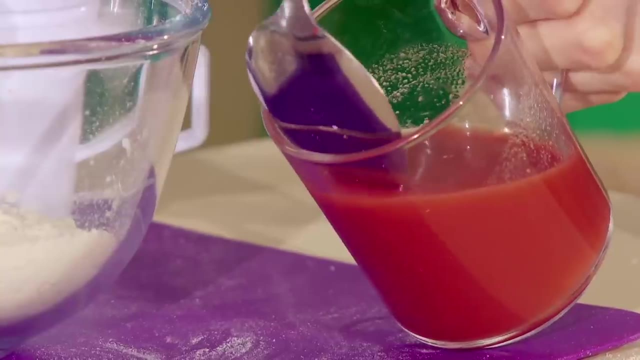 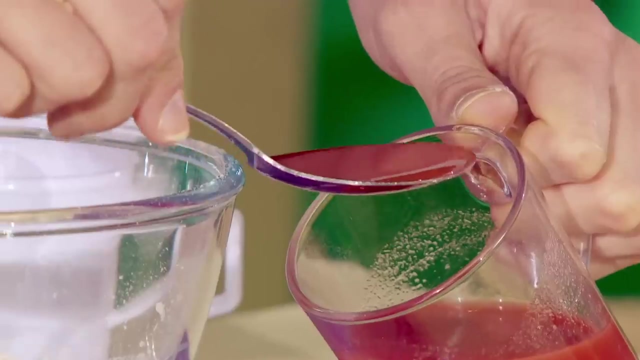 Right, I will show you how to play it. You have to hold the handle of the cup like this. Then you take your spoon, you tip the cup, load up your spoon with one spoonful of tomato juice and, very carefully, bring it over to your bowl. 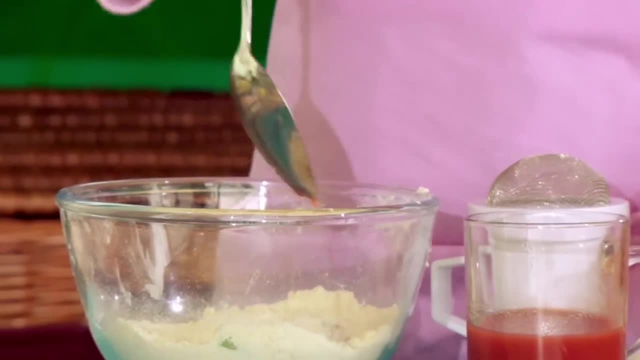 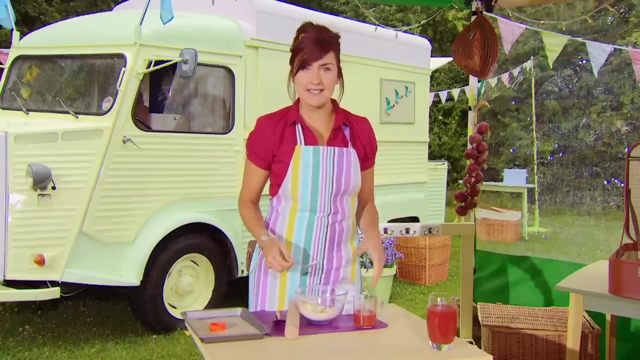 and splash it in Splash Splash. So we only need two tablespoons. and then take your fork and give everything a really good mix, because what we want to do now is make a dough Now if your mixture's a bit dry. everyone. 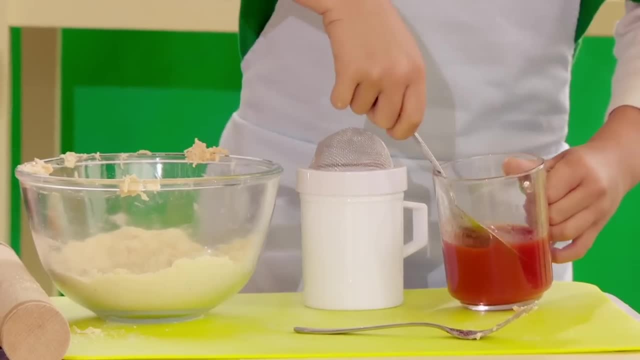 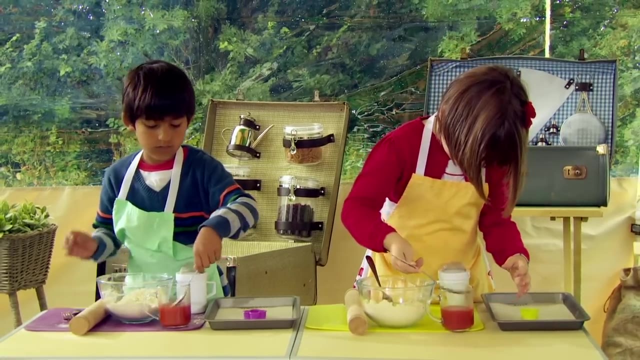 you can just tip and load again and add a little bit more tomato juice. I'm only going to add a little smidge more to mine, Just a tiny bit. Oh, it's all starting to stick together now And when the dough is ready. 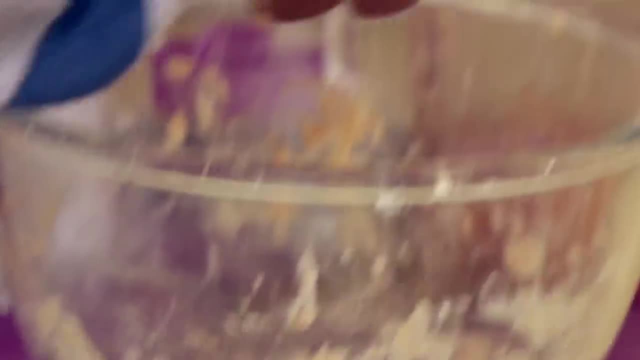 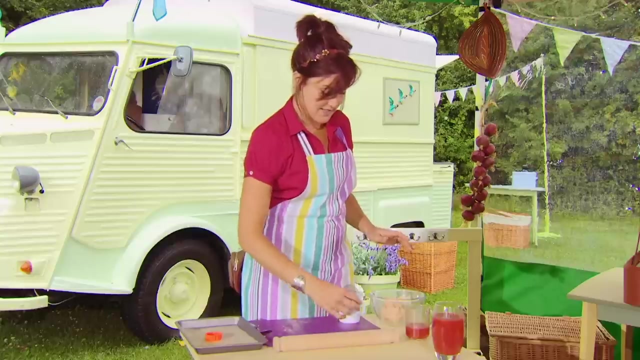 it's all going to stick together in a ball. Now what we need to do is roll it out. So let's move our bowl to the side and make lots of space, and then we're going to sprinkle some flour all over our mat like a big snowstorm. 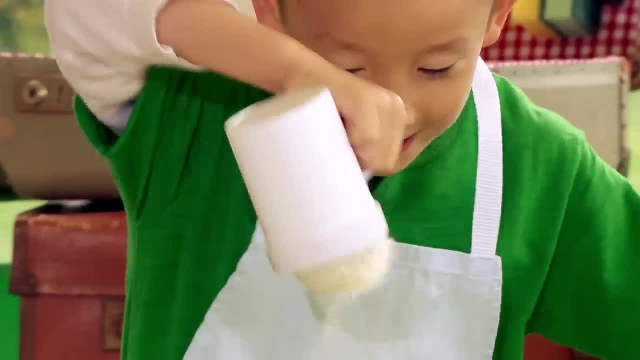 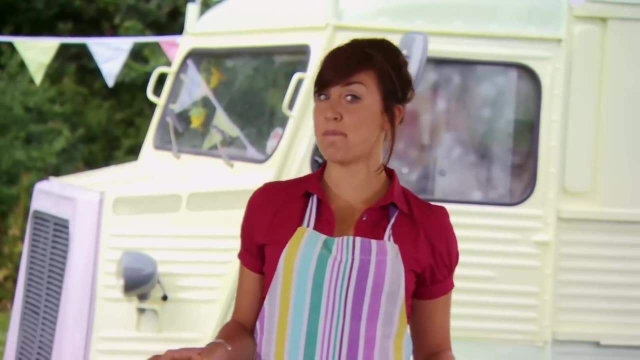 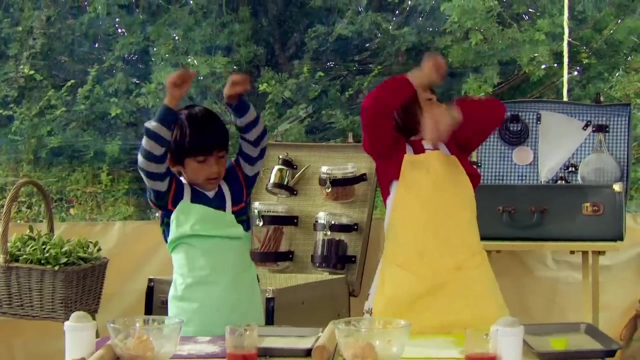 Three, two, one Make it snow for the dough. So the next thing we need to do is some rolling, But before we roll using our rolling pin, we're going to do a rolling warm-up. So you roll up, roll down. 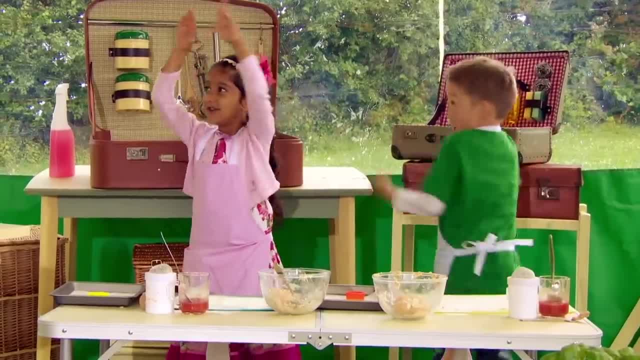 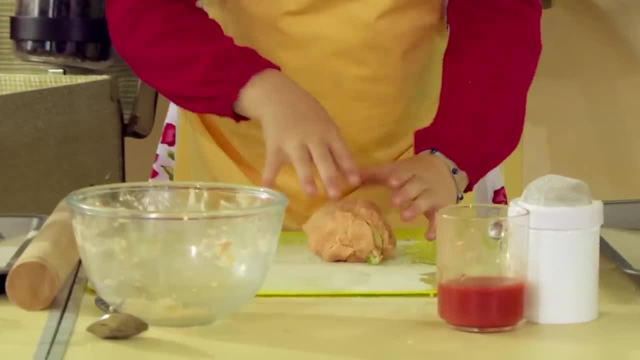 roll to the side and roll all around. Whoa, I think we're ready to do the rolling for our dough. now We take our dough and we put it in the middle of our mat. Sprinkle a little bit more snow on top. 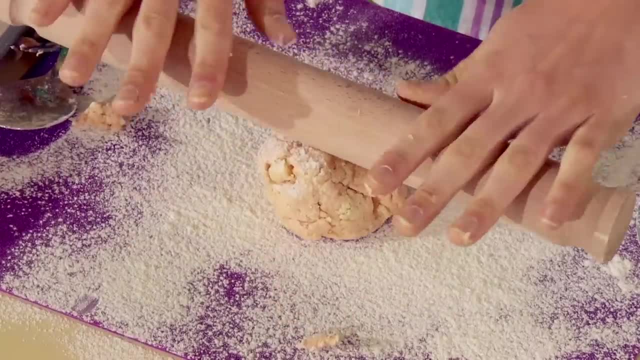 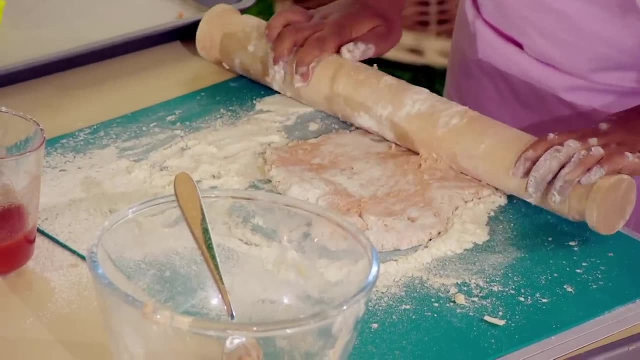 And then we take our rolling pin and we do some rolling, Like I am, And we need to make it big enough so that both of our hands fit onto the dough. Both of my hands can fit on it. Oh, brilliant, Rose, you're done. 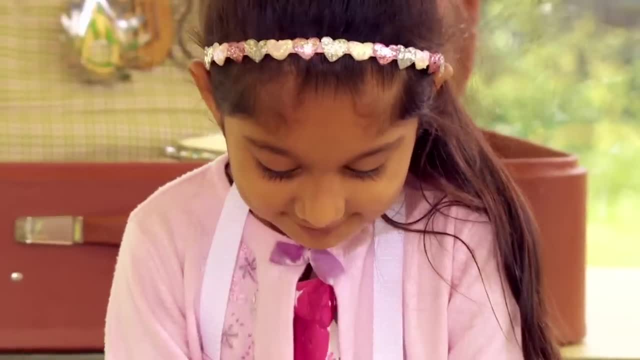 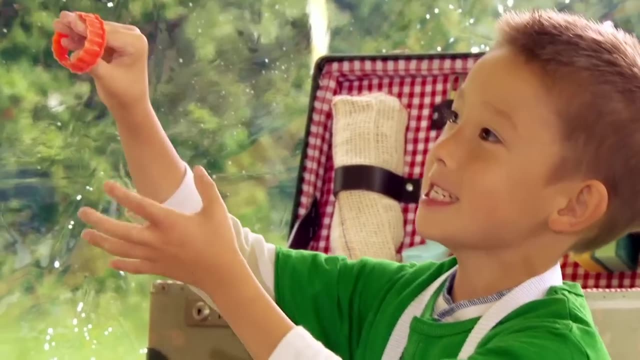 I think my hand's done too, My hand. Now we've all got different shaped but similar sized cutters. I've got a wiggly circle. I've got the same as you I have You have. Now we're going to make six different shapes. 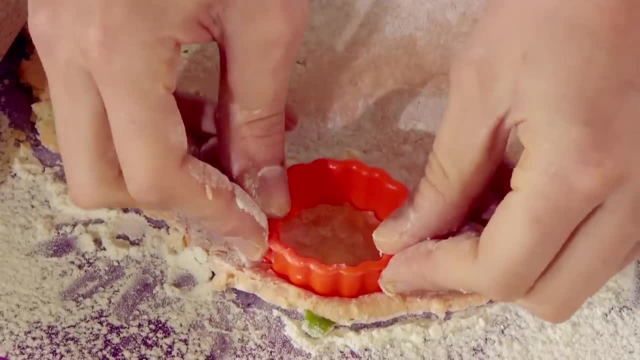 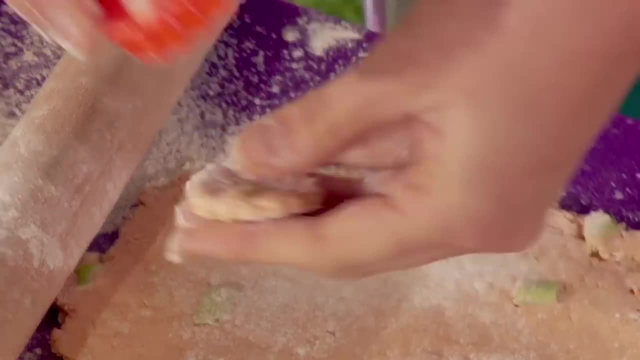 and we're going to start by cutting right up in the corner: Wiggle, wiggle, wiggle, wiggle, wiggle, wiggle, wiggle. So there's one, we'll put that over there: Wiggle, wiggle, wiggle. 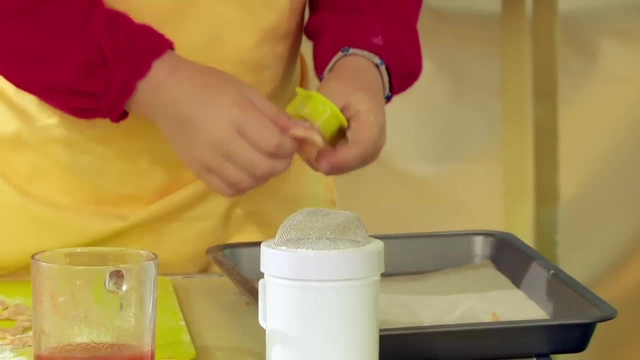 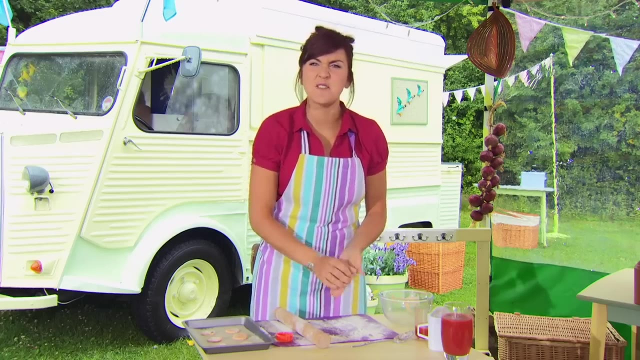 One more: Wiggle, wiggle, wiggle. I've got six. I've got loads of dough left. I think I'll put that in the freezer to make more melts later on. And that, everyone is it. You've done it. 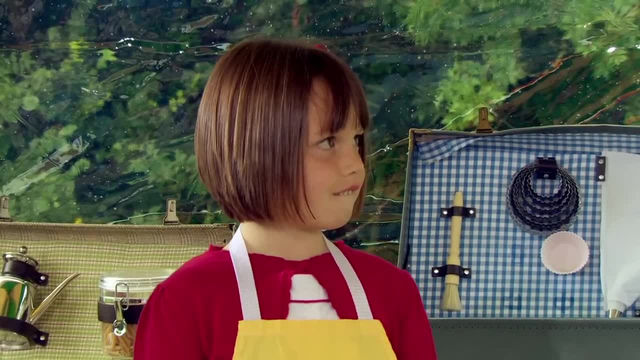 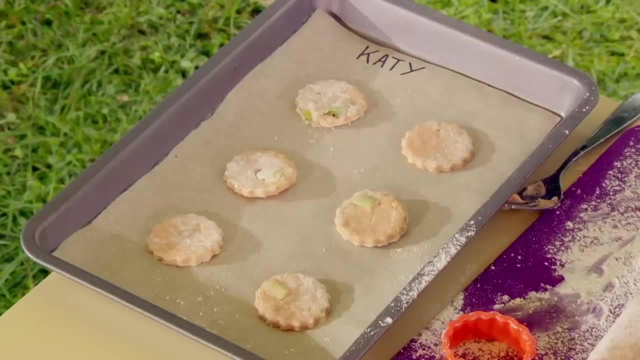 You've put all the ingredients together for your cheese and tomato melts and you've done it all by yourself. Well done. And now I'm going to put them in the oven. But remember, ovens are hot, so don't go near. 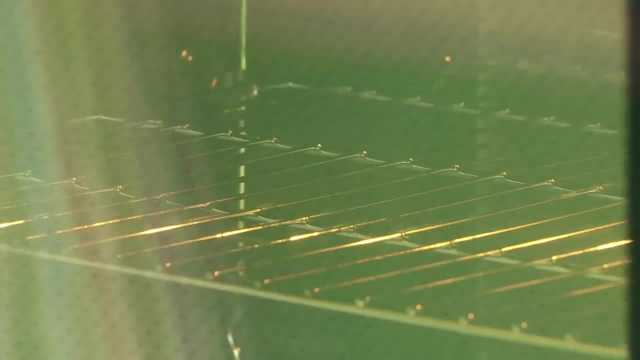 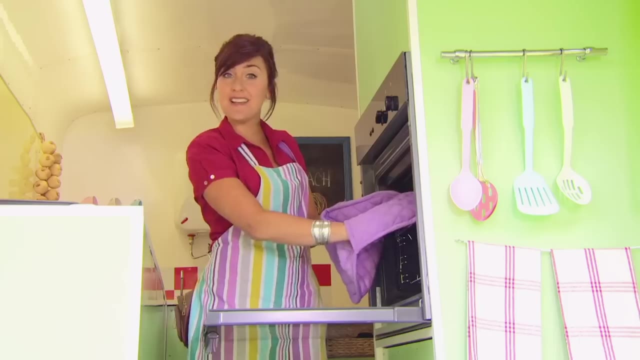 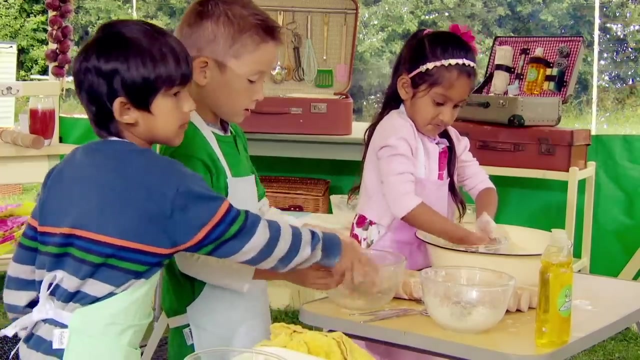 Ask a grown-up to help you here. Now we've cooked with you and had lots of fun. Let's tidy up and think of all the things that we have done. There was Swing, Tickling, Snipping, Rolling, Now clearing any mess. 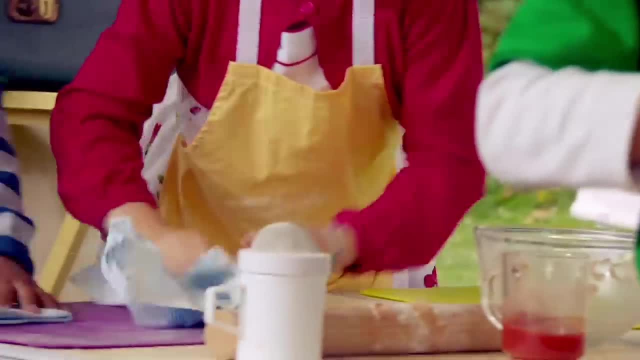 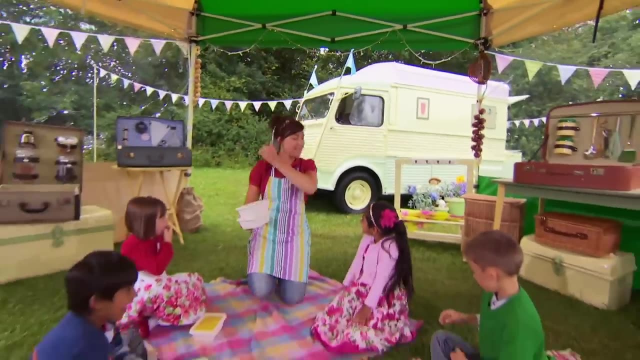 and putting things away is always fun to do at the end of the day. And here they are, everyone all ready for us to eat. Who's excited Me? I am so excited, Jake. let's have a look at yours. 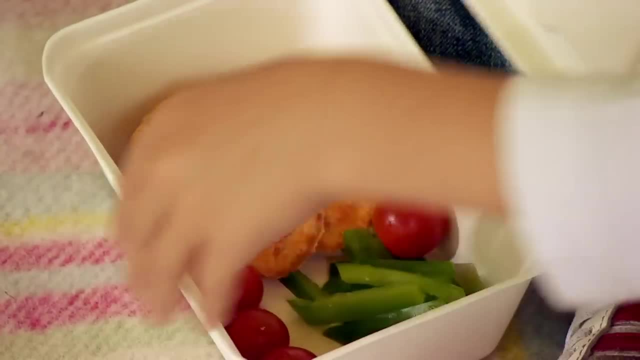 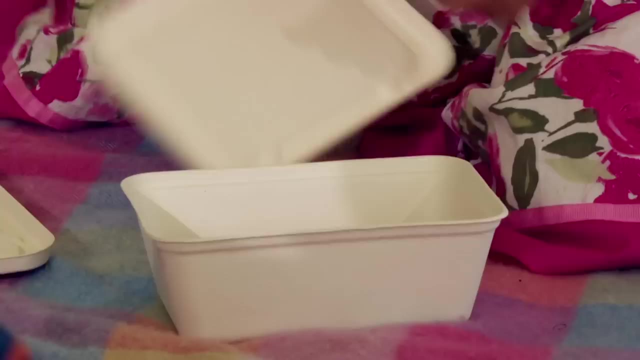 Ready Go. What do you think, Jake? It looks nice. It looks really tasty, doesn't it? Yeah, Let's put the lids on top of our food and we'll save the rest for later. We've travelled to you. 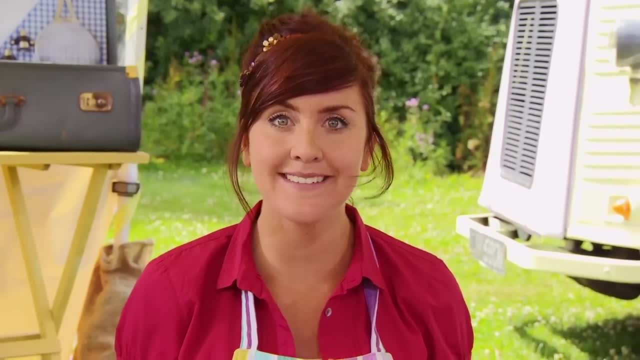 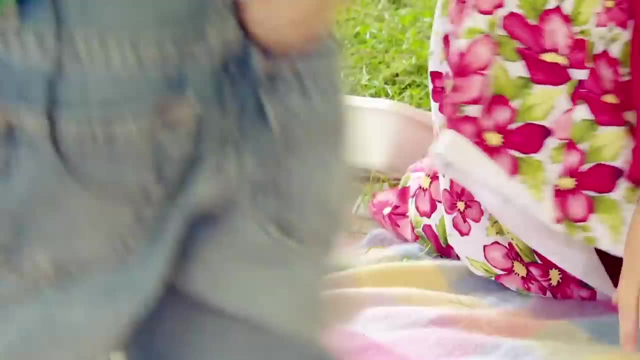 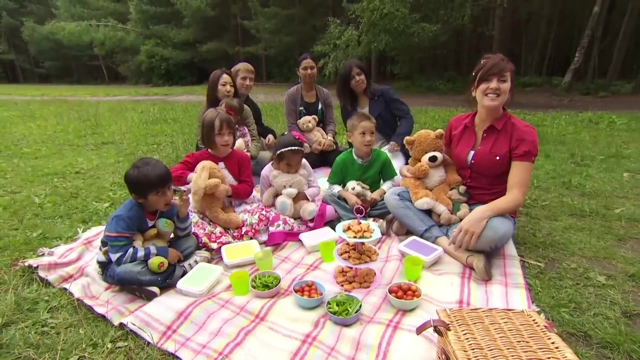 cooked and had fun. Now let's have a party with everyone. Yeah, Come on everyone, Let's go, And you can come too. Come on. Well, here we are in the forest and we're all ready to have our teddy bear picnic.